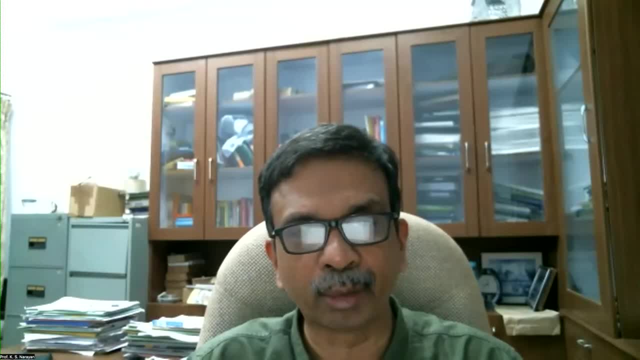 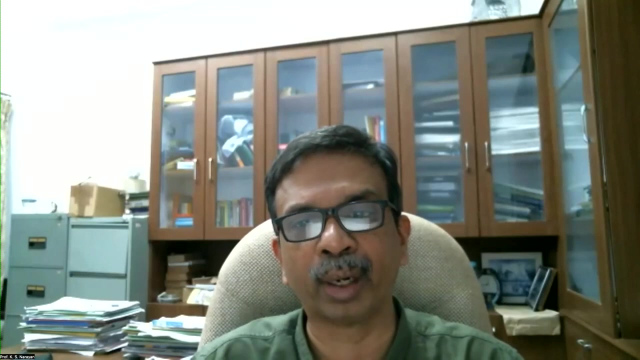 can find our previous webinars on YouTube. We normally have these webinars on Saturdays live twice a month, typically at this time five in the evening. I am joined in here by Dr Sushila Venkatraman of IIT ACB, who has been the major driver for these webinar series. 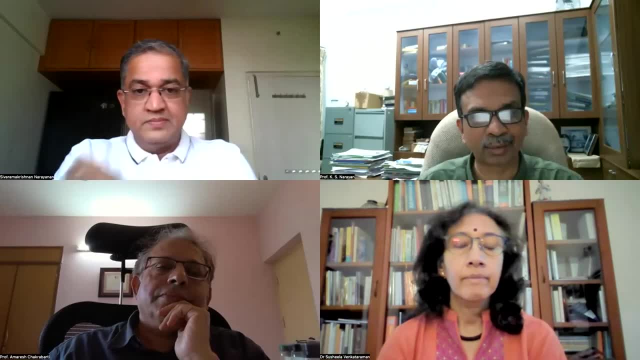 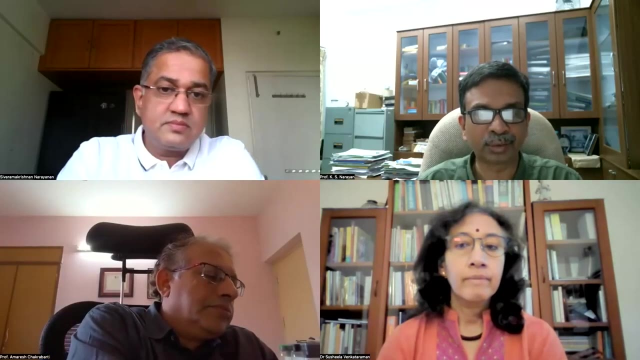 And during this course of pandemic we also realized the importance of manufacturing that too, at scale and speed. So this webinar today is going to be very relevant, considering that In the last seven, eight years, industry 4.0 has taken root across. 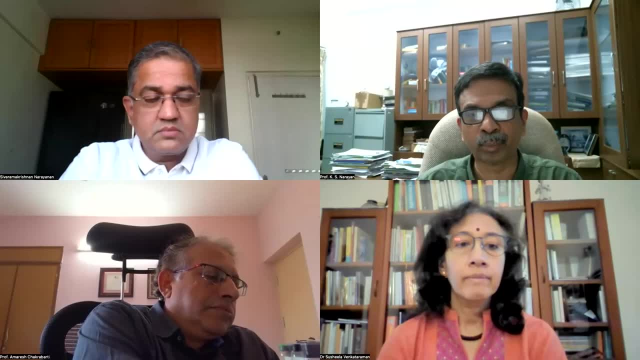 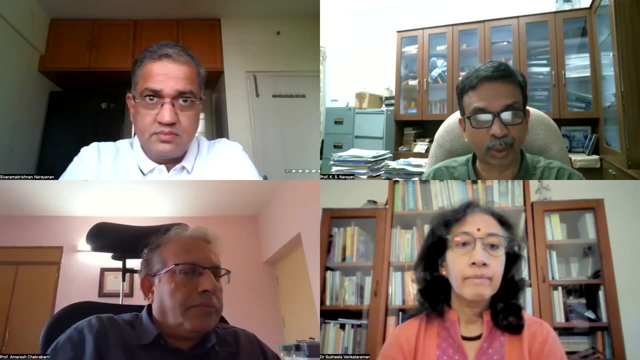 the world in advances in computing power and algorithmic research has accelerated the process of adoption and productivity gained from this concept. So we are very pleased to have Dr Sushila here with us as he discusses the things that are going to happen in this future. 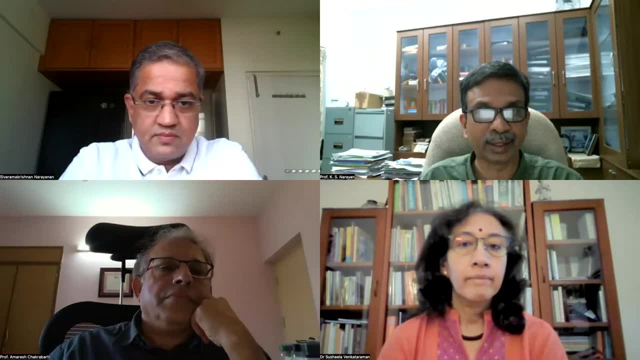 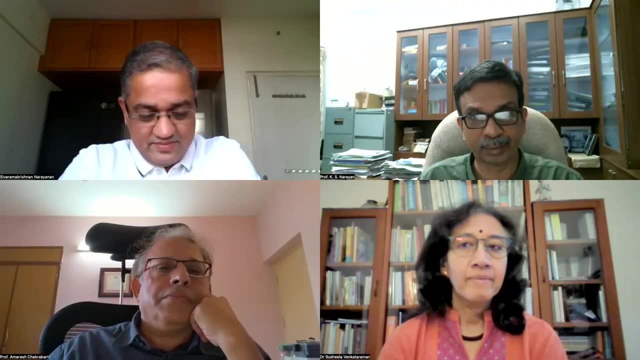 Hi everyone. my name is KS Narayan and I am the Chief Executive Officer of the IIT Alumni Centre. We are overseeing the manufacturing of these technologies. We are currently working on the development of a new product, ie the IIT building machine. In this video, we 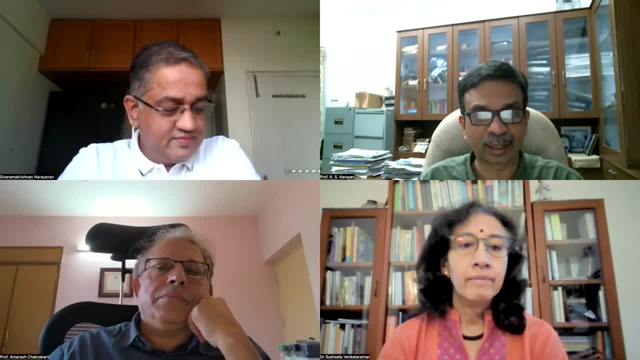 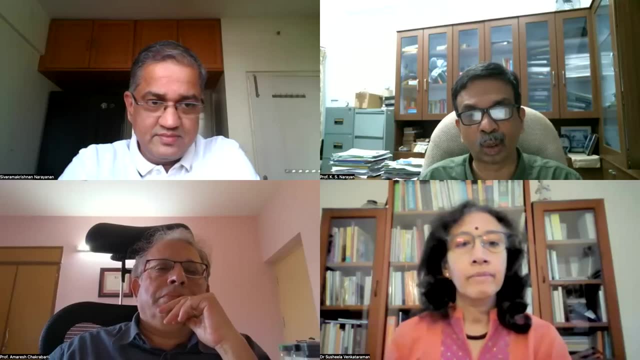 will discuss the concept of integration to IIT and then we will discuss all of its features. Thanks for those institutions involved in solving some of the next generation manufacturing challenges for his clientele, using technologies like machine learning, industrial automation, business analytics, etc. 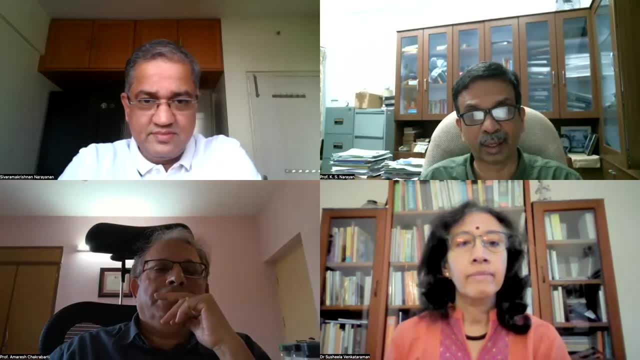 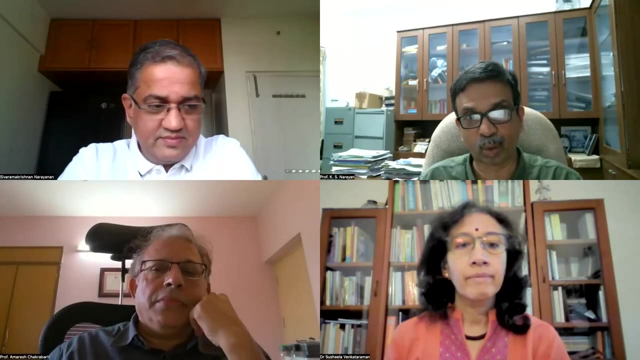 He is a mechanical engineer from Bangalore University and a post-graduating management from IIM Calcutta, So moderating this talk today is Professor Amresh Chakraborty, a very well-known figure, a senior professor and current chairman of the Center for Product Design and Manufacturing. 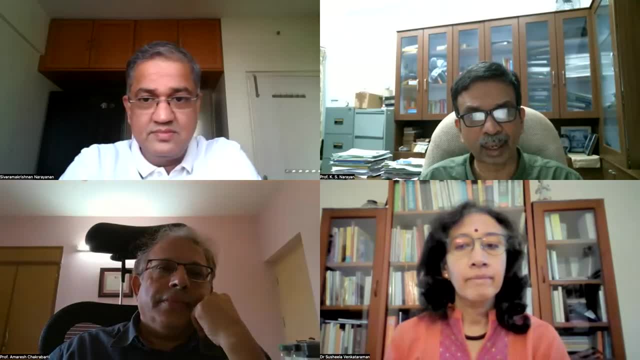 at Indian Institute of Science Bangalore. He is also an engineer, is an IIC alumni, took an ME and a PhD in engineering design from the University of Cambridge, where he has led the design synthesis group for nearly a decade. So after joining IIC. 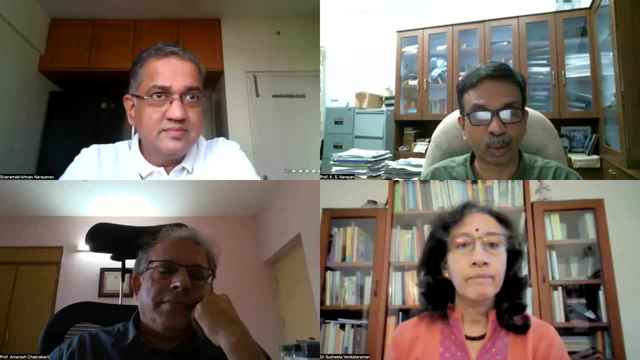 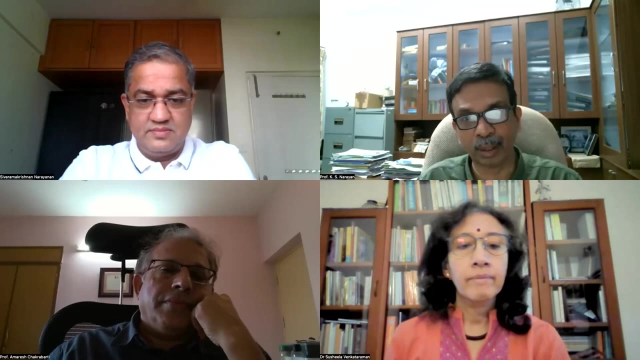 he has been a senior professor and current chairman of the Center for Product Design and Manufacturing at Indian Institute of Science, Bangalore. He has been very actively involved and very well-known for the design research methodology. He has founded the Ideas Lab, India's first design observatory. He is also the editor of the artificial intelligence for. 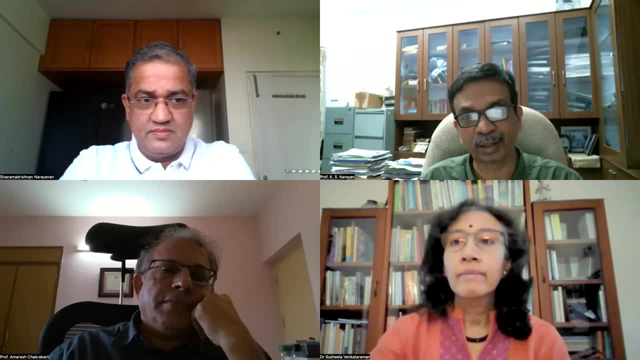 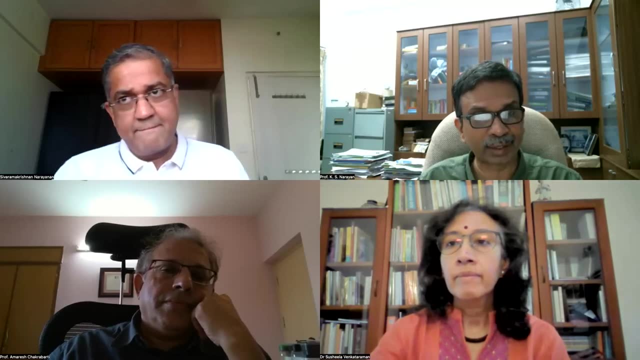 engineering, design analysis and manufacturing AIE and BAM journal. I think it's a well-known journal in the field, So in fact he has written a lot about the design research methodology and the design research methodology. He has also written a chapter titled What is Industry 4.0 for India? 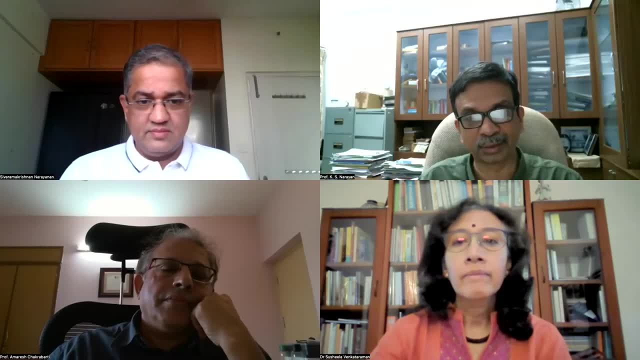 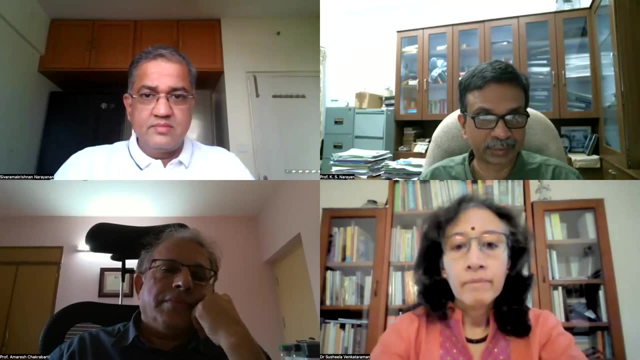 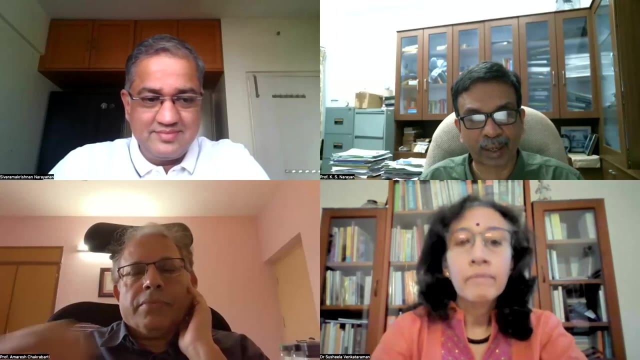 a recent chapter in a Springer series book, So we'll have an interesting view from an academia also over this discussion. Okay, so, with this short introduction over to the speakers, And just before I hand it over to the speaker, I just want to let people know that they can engage. 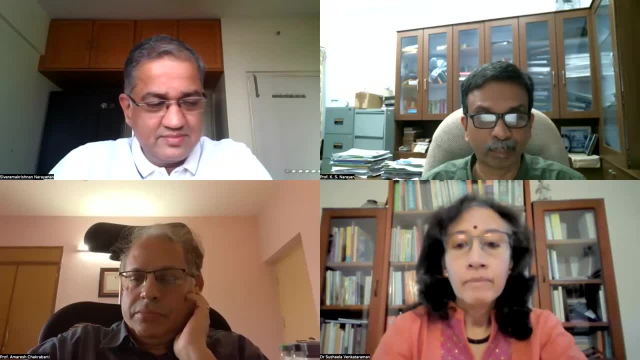 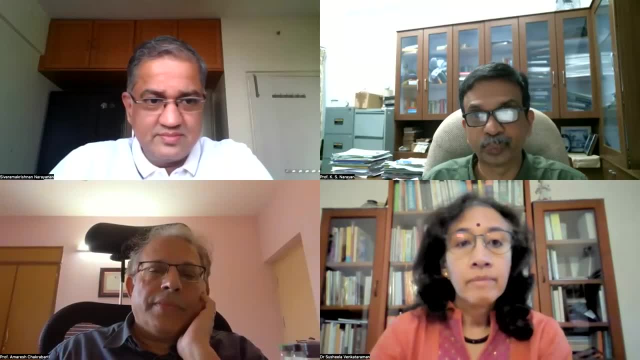 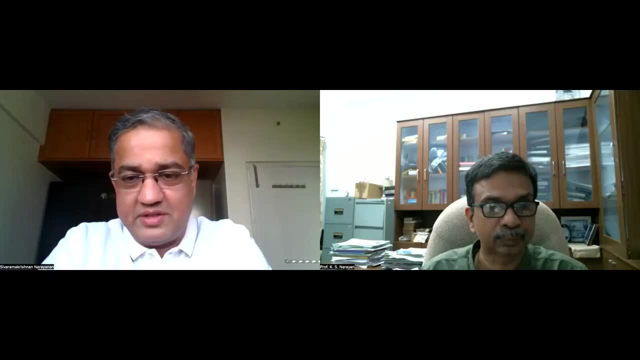 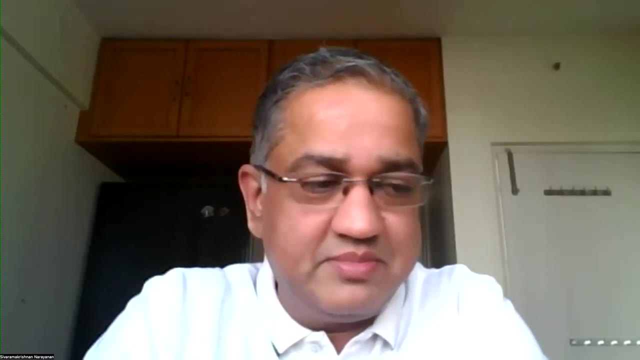 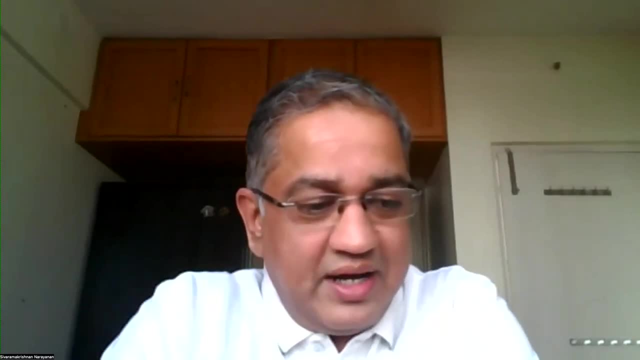 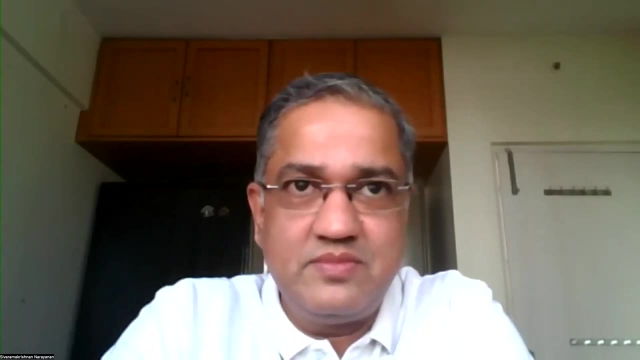 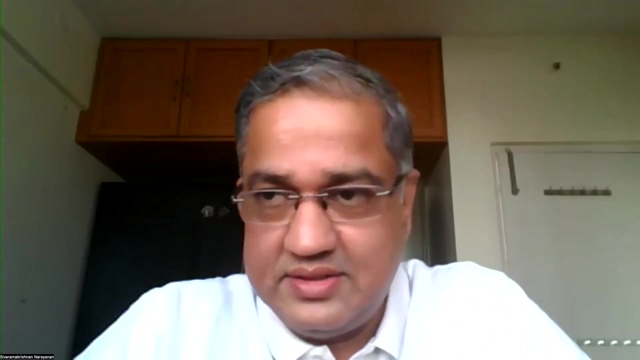 indulged in quite extensively. Just one last piece that I probably missed out. I believe. you know, as a management professional, as a working professional, you should, you know, kind of get your hands dirty in the subjects that you're interested in. So, following that, 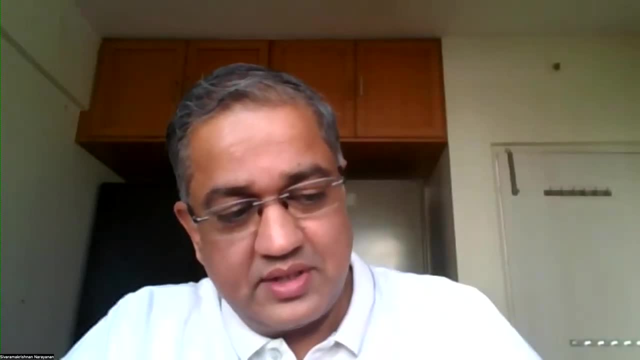 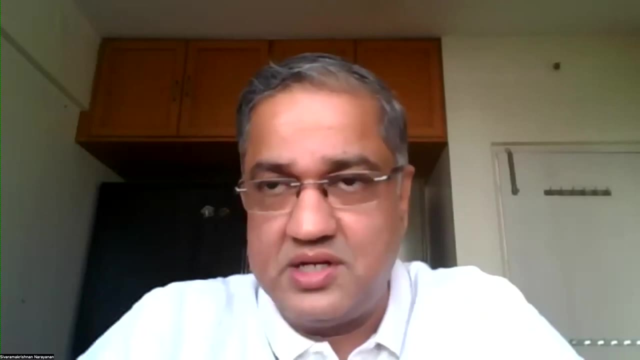 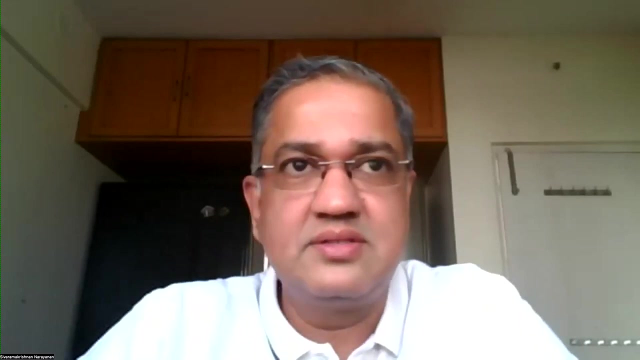 principle. I also acquired for myself a postgraduate program, a certificate from Purdue University, after working for a year in the space of artificial intelligence and machine learning, So I finished this in the year of 2021.. So this field and the areas that I'm going to talk about is so interesting and such a central part of what 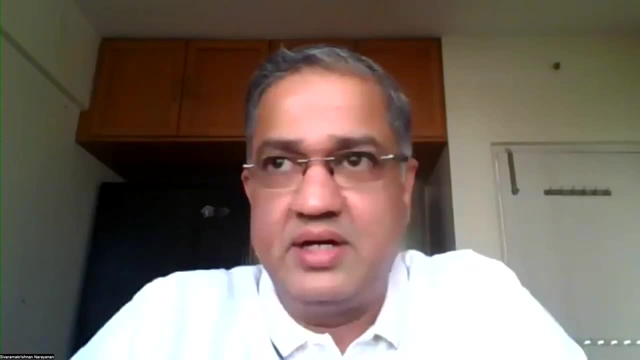 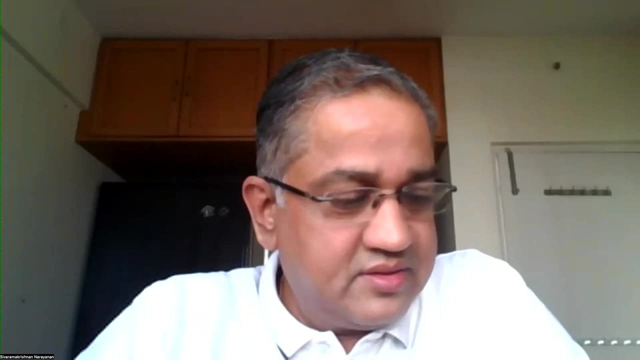 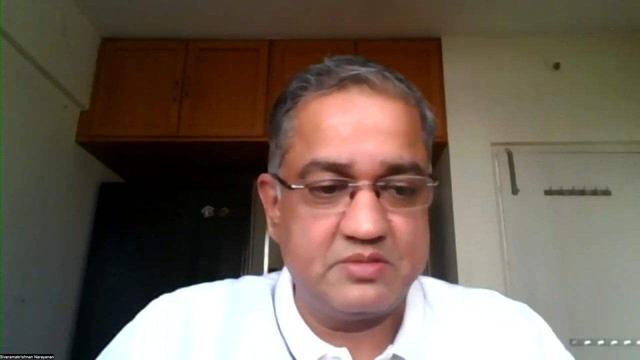 I do that. I thought I'd be letting myself down and my clientele down if I don't have a better and more formal visibility of the topics at hand. So that's about me And, like I said, I'm happy to be here and I will share my screen so that we can start today's proceedings. I hope you can all hear. 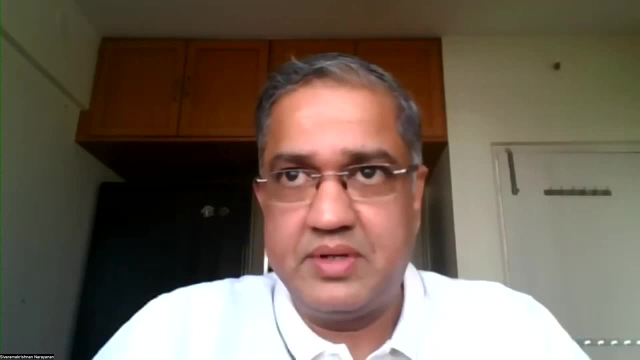 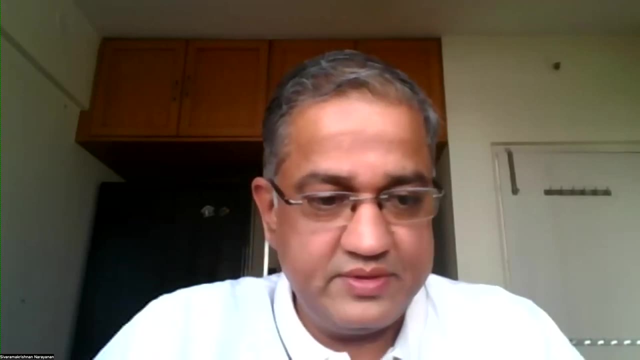 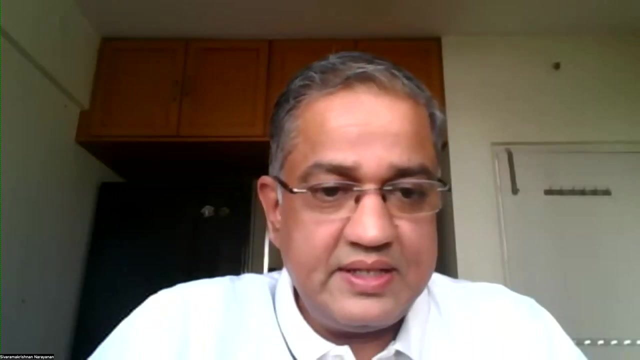 me clearly. if there is any problem, Please do type it up in the Q&A so that the moderators can just stop me and we can rectify the problem for you Can hear you. Okay, Let me share my screen And if you can confirm that, you can see it. 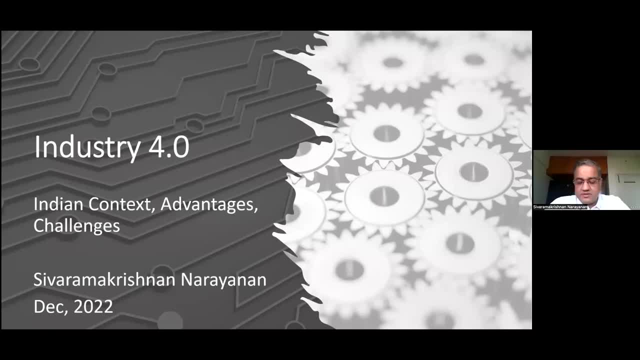 Yes, all good, Okay, Wonderful. So what I'll do is: I mean, it's a topic you know. on the one hand, it is a passion And, as with people that are passionate about any subject, the rest of the world sometimes just gets bored out of their skulls. So what I've 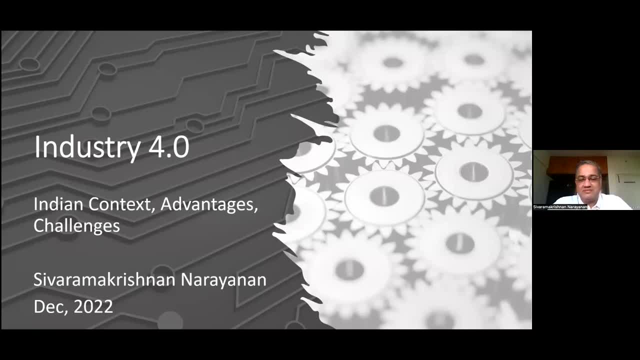 done is to try and keep it in two levels right. So one is to try and see if we can cover the broad policy, the landscape that we're talking about here in India. What does the landscape look like? What is the landscape of the industry for in general? And then the second half of this. 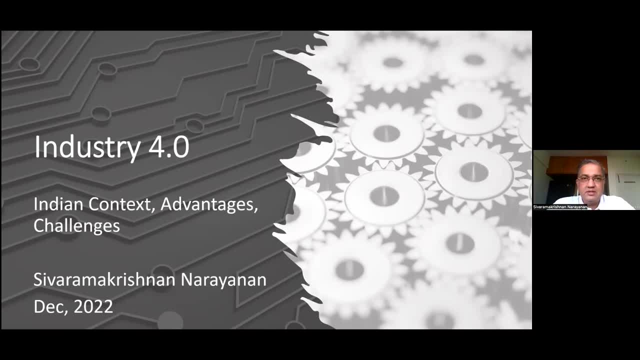 day's discussion will be more focused around practical examples, examples that I have seen, worked on myself in various engagements for various clients- kind of without naming the names, because this is going to be a public, accessible video- try and provide you a flavor of what happens right and how typically clients go about doing the work. 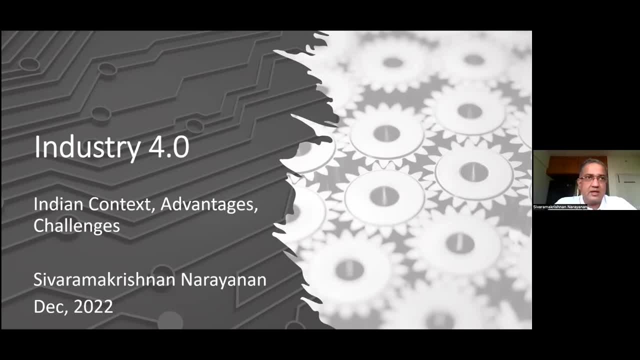 It's fascinating. It is fascinating. It is sometimes brilliant, sometimes extraordinarily creative. of course, extraordinarily frustrating for the people that are doing this in the field, because no good work comes out of simply luck. A lot of hard work goes into it And that is. 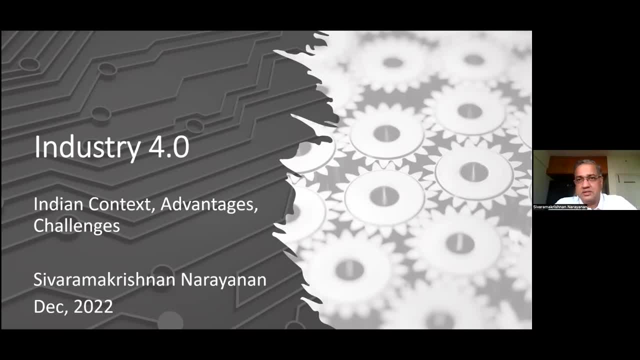 something that I wish to highlight for those of you who are interested in this journey and the end outcomes of this journey. So it's been a very interesting discussion. I hope I did And I hope you enjoyed it. Thank you very much. Thank you. 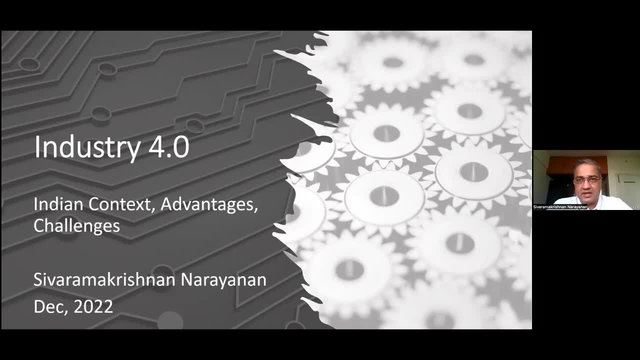 Thank you in two parts: one which is more policy and high level, another which is more examples and from the ground, and you know. any questions, any clarifications, any doubts anybody may have, please feel free to post it up and i'm more than happy to take them along with professor. 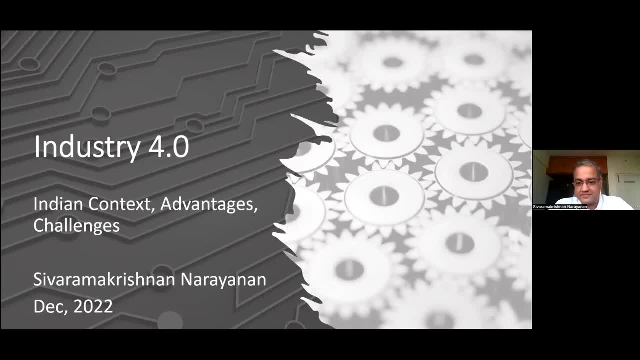 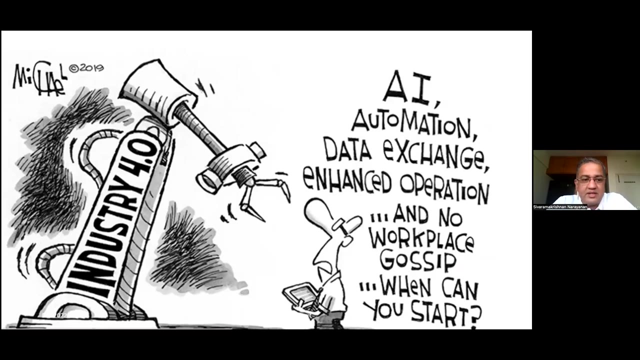 professor amrish, my collaborator for the day. let me get going. so what is this all about? right? so industry four: why is it four? why not four and a half? why not six? so there is a lot of, obviously a lot of excitement about it. so i start. i start with something that you know. we see this almost. 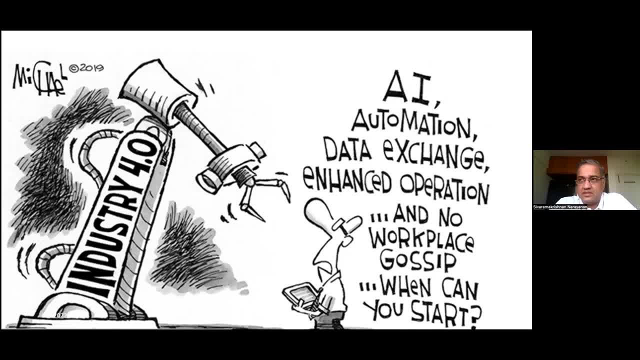 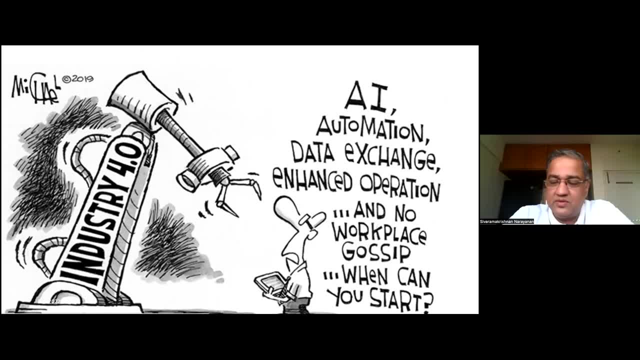 in every technology that takes birth over the last hundred eighty hundred years. right, and this is a typical management person saying: you know, you don't even gossip, you know, and i'm getting more productivity per rupee of invested money. uh, so when can i start? right, everything is positive, so it's almost a silver bullet, right? 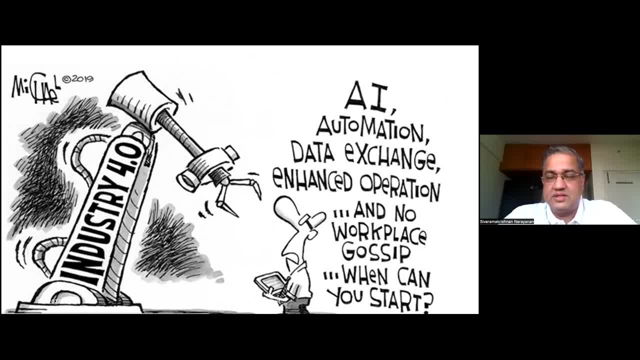 and anything, uh that we have seen in the last several years, whether it is a simple payroll application in the middle of the century, last century uh, or the erp systems that we are all now very familiar with, uh, in the last 25, 30 years, my career actually runs in parallel to the growth. 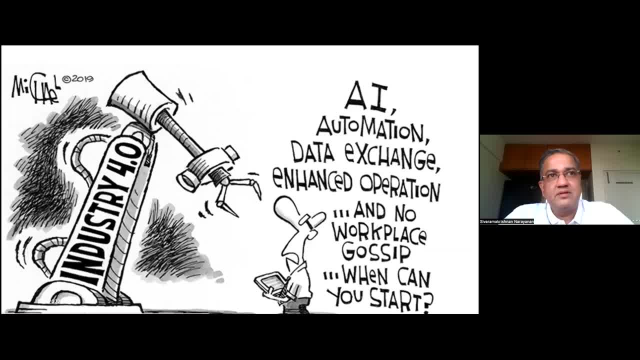 of erp in india and everybody is almost always saying this will solve all the problems. so in fact i'll just stay here for a minute. uh, just to summarize, you know another humorous episode. so we were doing an erp project for a very big company in the west. 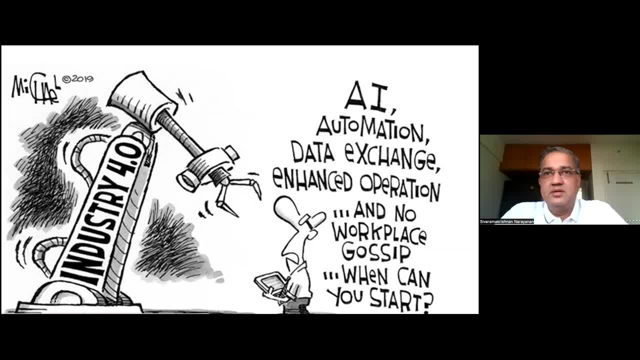 and uh, one of my colleagues was in the room, uh, along with the cio, and we were. it was a little late in the day, um, and the expectations were running high from the client. and my colleague says, from behind his computer: once we go live, uh, if you post a, 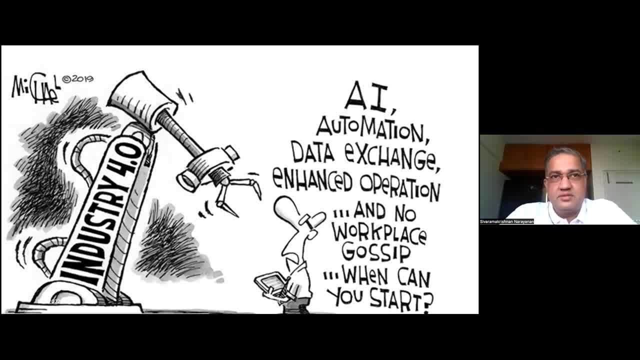 wrong accounting entry, then a red light will glow in your room. so the cia was obviously taken aback and he said: how do you say that? how does how does the crp, uh, tell me or you know, warn me that a wrong accounting entry has been passed? so my friend gets up, goes to the switchboard and turns on a lamp. 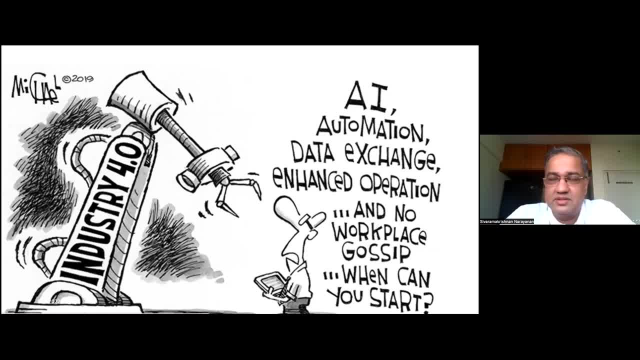 and say: this is how, because i'll see the accounting entries wrong in the system and i'll go and turn on a lamp so many times. uh, the uh. the way that things are done may not be all automatically automated and, uh, you know, very slick uh, but the end of, at the end of the day, uh, we from india, we. 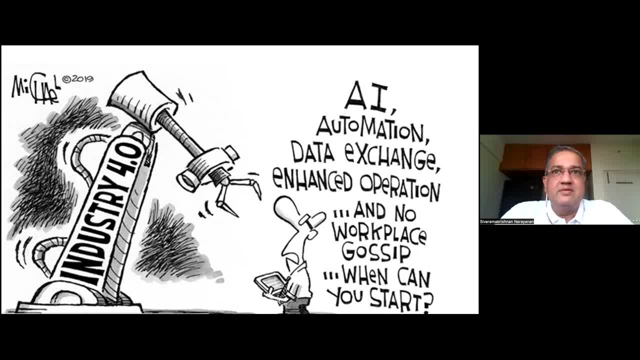 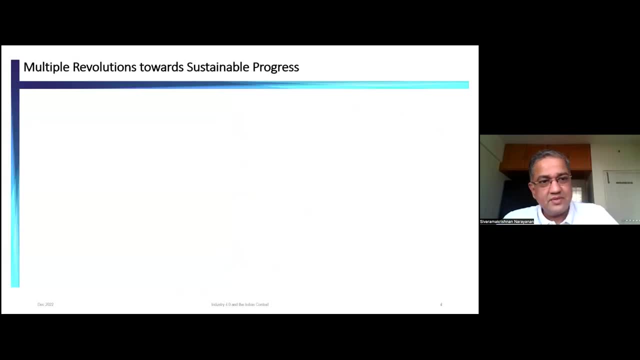 have this mentality of getting things done. uh, many times it is great, many times it's not so. uh, this one in particular, the industry revolution 4, offers us a chance to really become world beaters in manufacturing. so we will talk about how this happens, right? so what is industry revolution 4? 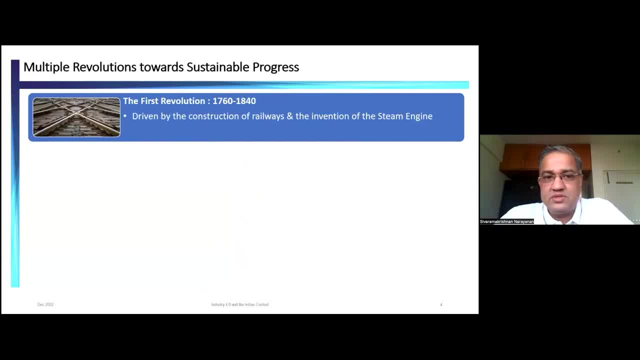 and why 4?? right, so the first revolution was really driven by the construction of railways and the invention of the steam engine, right? so if you all remember your history lessons from school, the cotton gin and the steam, uh, james watt and the experiments that he did with the steam engine- uh, that's where. 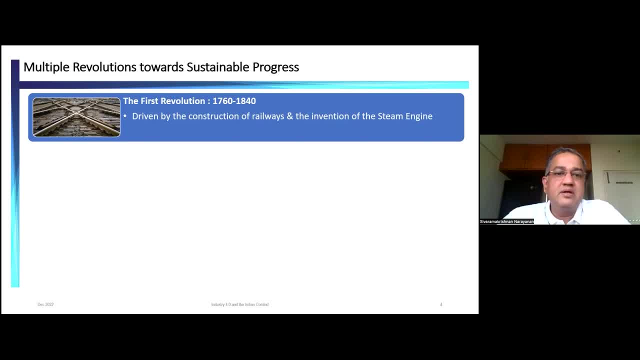 the whole industrial revolution starts, uh, and this lasted between 1760 and 1840, right, and this period of history was extraordinarily rich and productive in both scientific- uh, thinking and engineering, um, and this was the first industry revolution where things moved from merely being handmailed. 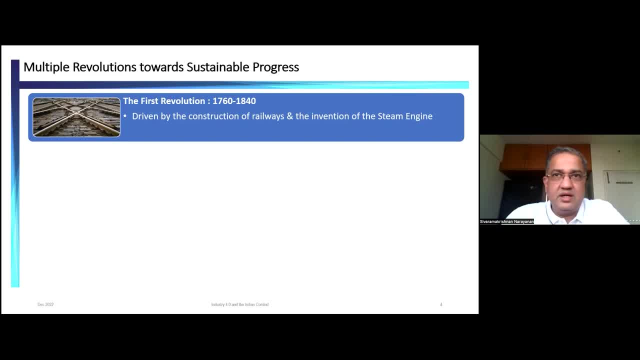 to being more machine driven, more scalable and, you know, repeatable kind of work. the second revolution started when ford started his model t factory, right where he wanted to have a vast factory which owned everything from the forests of teak to the final marketing of cars to the 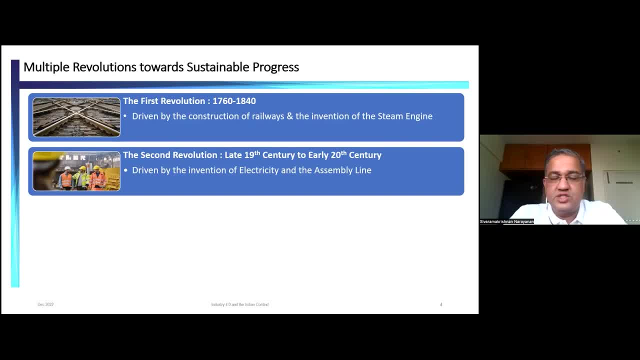 customers, customers, the assembly line, the invention of electricity, Thomas Edison, Nikolai Tesla- great people that worked a lot in electricity- and, of course, Michael Faraday right. So in all of this there was a lot of gain that people made. 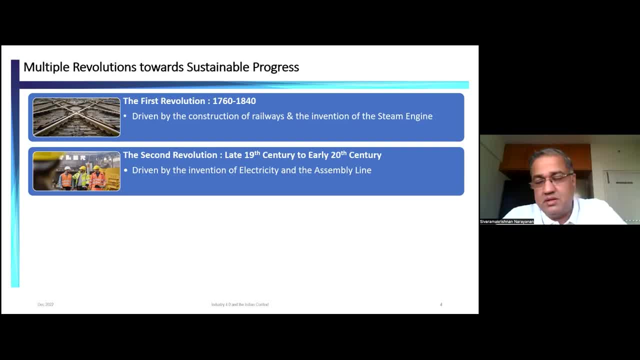 And today the modern assembly line is a symbol of the industry, of the manufacturing industry, to that extent So it's become a characteristic of the industry. It was not so about 100 years ago. The third industrial evolution: I'm sure a lot of us have lived through this. 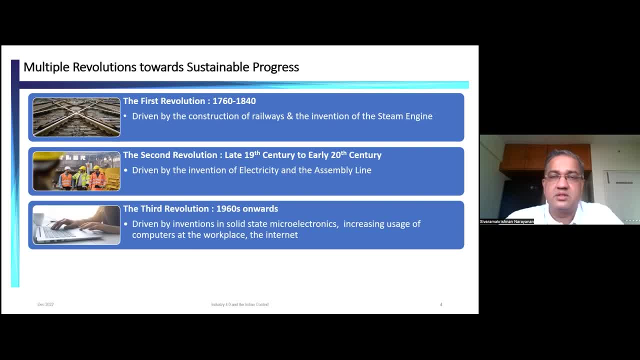 It really started when the first ENIAC computer, which occupied an entire block, and when it was turned on, the legend goes that the lights of Philadelphia dimmed a little bit. It consumed that much power And from then to now, when we carry a smartphone in our pocket which has the computing power, 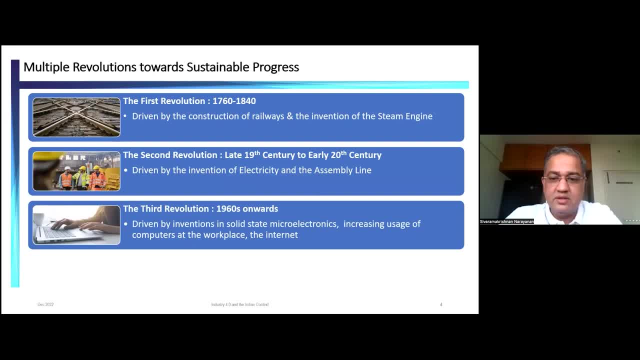 equivalent to that machine That occupied an entire block. I think we have seen the growth of this where almost every department in every company that we go to use a small spreadsheet application or a very large and complex design application. Yesterday, in fact, I was in a company that manufactures components for the aerospace. 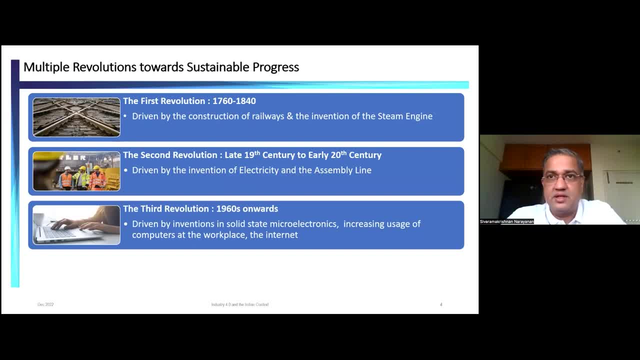 industry and the laser cutting machines that I saw there, and this is here right here in Bangalore. It could have. It could have been in any advanced part of the world, and the computer that was sitting on it was just as powerful as an ENIAC, helping cut components for the industry right. 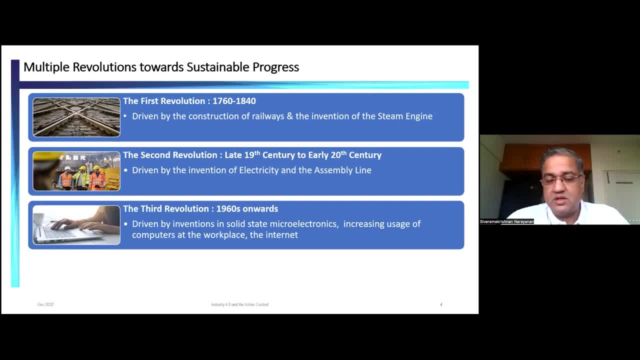 So this came about because of improvements in solid state microelectronics and almost a frenetic pace of adoption of computers in all aspects of work that we do today And what we are doing right now. this presentation is just as well a child of the third industrial. 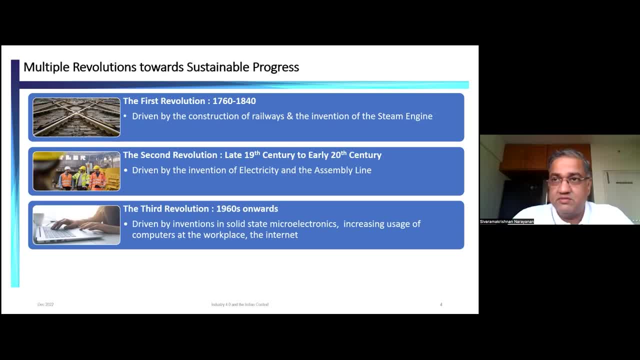 evolution That I'm able to talk to all of you on a video conference from home, clearly, and sharing my screen and also looking at the questions that you're posting. So there is a collaboration that's happening which was simply not possible as recently. 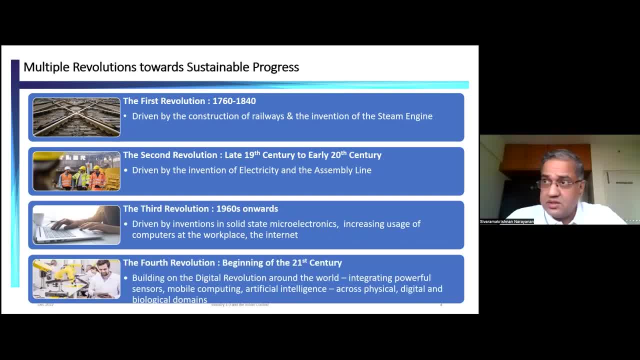 as eight to 10 years back. Now this brings us to the fourth industrial evolution, which is now very interesting because very disparate, very unconnected or previously unconnected aspects- And we're seeing a lot of these aspects of business- have started getting connected. 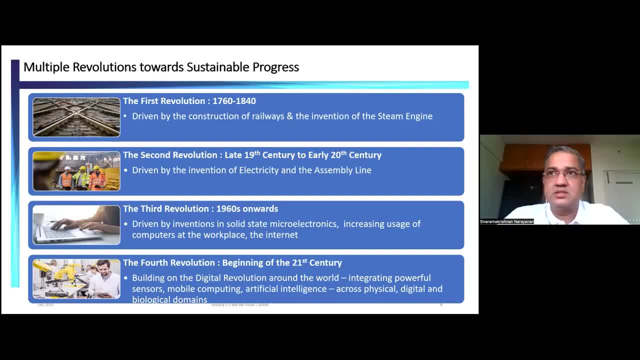 So suddenly we are seeing biology, which was earlier limited to a pharmaceutical industry or a biotechnology industry, people who are specialized there. now it is thrown open And a lot of people are engaging in aspects that we previously thought was inaccessible. It is: technology has democratized the possibility of engineers working in advanced biology applications. 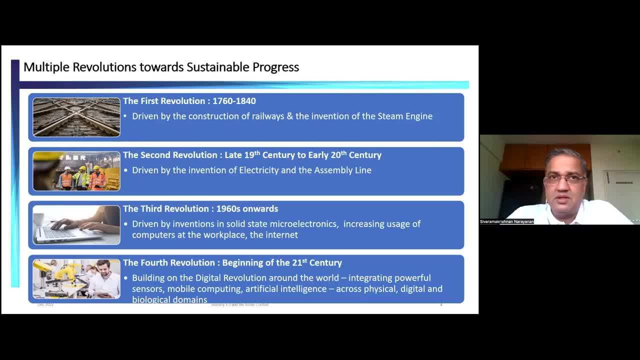 nanotechnology for diagnostics And even in patients. there's something we've all read about, And some of these are actually here in India: Right Hospitals in India using nanotechnology to identify if there are cancers that they cannot otherwise access using standard imaging technologies. 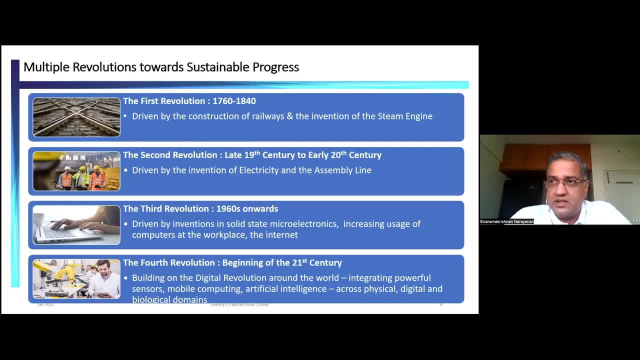 So a lot of these things which are otherwise unheard of and what would have sounded straight out of a book from science fiction is now available to us. who would have imagined that you can actually print human tissue- And we will talk about this in a little while- And the phenomenal work that 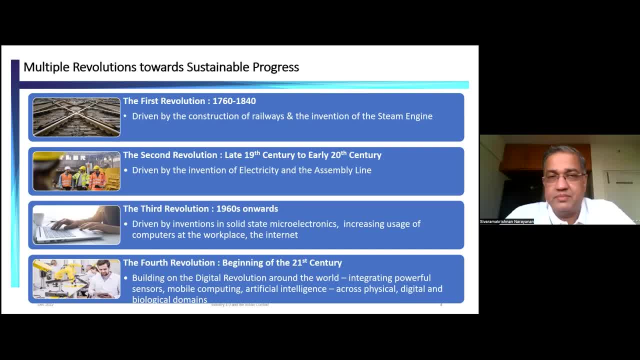 is happening right here in Bangalore, right? And if you just go and type up some of the phrases- and I was just doing a simple thought experiment in preparation for this presentation And I was typing things like industry four in Bangalore, 3D printing in Bangalore, you know some experiments. 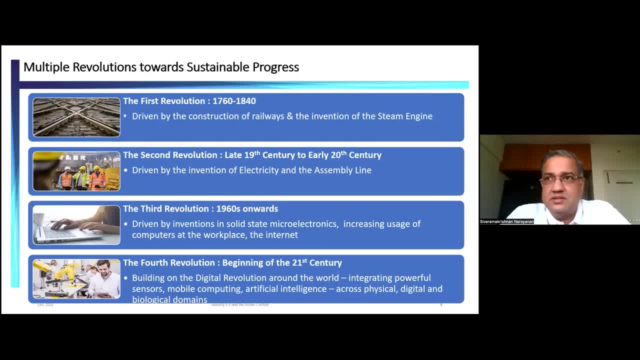 like this into a Google search bar And within 0.35 seconds- 0.7 seconds- I got a million search hits. okay for this kind of a very general, very casual search And I'm sure a lot of those. 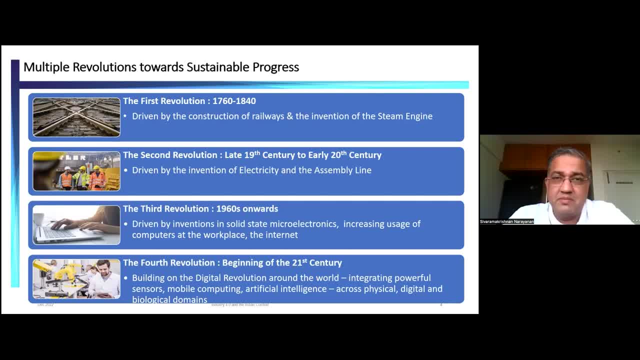 would be repeated or junk, or probably not in Bangalore, But suffice to say that the first 8,, 10, 20 links that Google threw back at me were all in Bangalore. right, And this is just Bangalore, And the rest of India is still an untapped, unexplored potential. A lot of these companies. 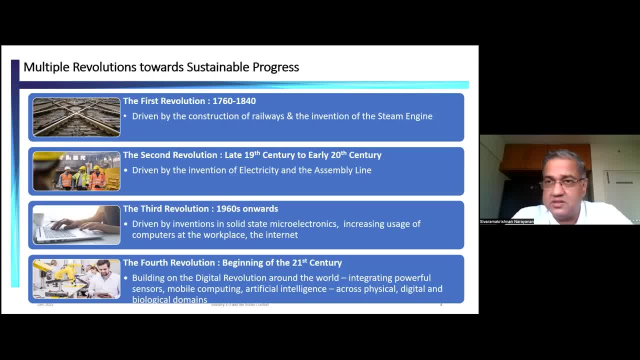 are bringing together space technology, biology, engineering, physics and, of course, at the root of all of it- mathematics- advanced mathematics- in ways that we have never imagined before, And today we are poised in a place where we can actually turn this to our advantage. 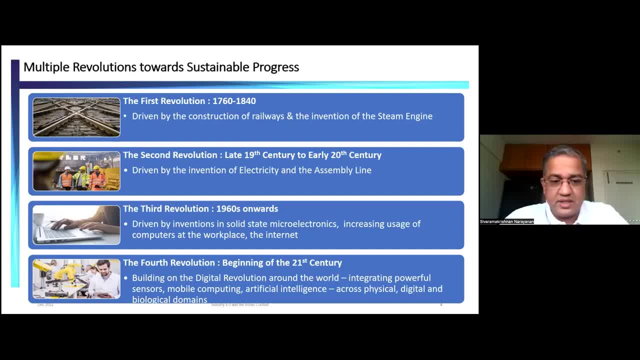 It is for us to figure out what we need to do, right. So this is why it is the fourth industrial revolution And we are looking at standing here today. we are looking at a sustainable future. we are looking at how we can not damage the one planet we know beyond repair for our future. 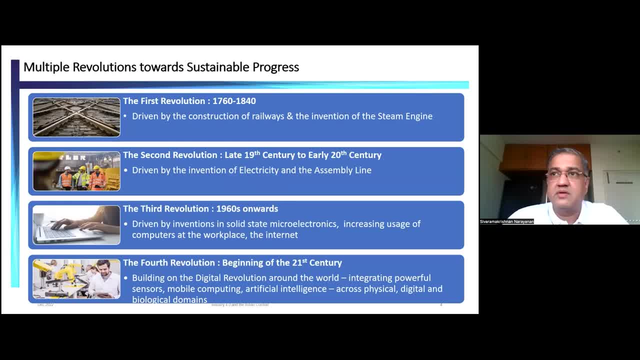 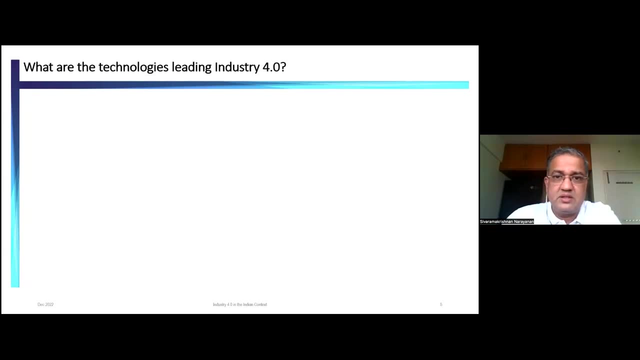 generations, and how we can build on some of these technologies in ways that help us get you know, contain global warming, get back into a more sustainable track of development. So what is it that takes us into industry four? So the first and foremost is green energy. right, How do we harness the sources that we have in abundance in nature- solar energy, wind, energy, waves, geothermal, magnetic, you name it. 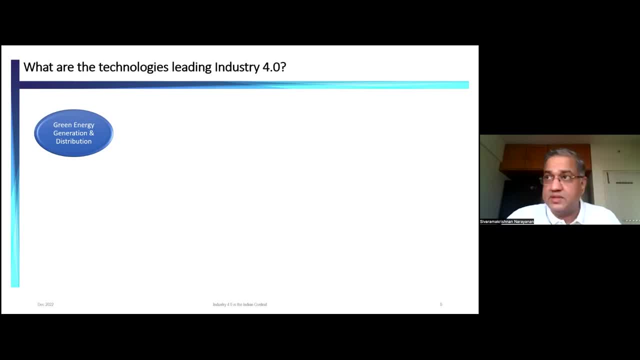 How can we generate this energy in carbon neutral ways and how can we distribute it right? While electric cars are all the race cars, right? While electric cars are all the rage today, you know, the question really that hangs over the industry is: are they actually, when they finally are in the hands of the consumer, are they truly carbon neutral right? 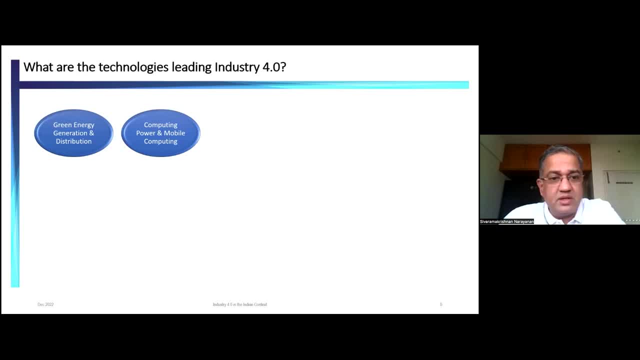 So that's something to think about. Of course, we've touched upon a little bit on computing power and mobile computing. We have immense power in our fingertips. I mean a little toddler. today my own sons had more efficiency on an iPad when they were three and four than when I had with a laptop when I was three and four, than when I had with a laptop when I was six and a half years old. I mean a little toddler today. my own sons had more efficiency on an iPad when they were three and four than when I had with a laptop when I was six and a half years old. I mean a little toddler today. my own sons had more efficiency on an iPad when they were three and four than when I had with a laptop when I was six and a half years old. 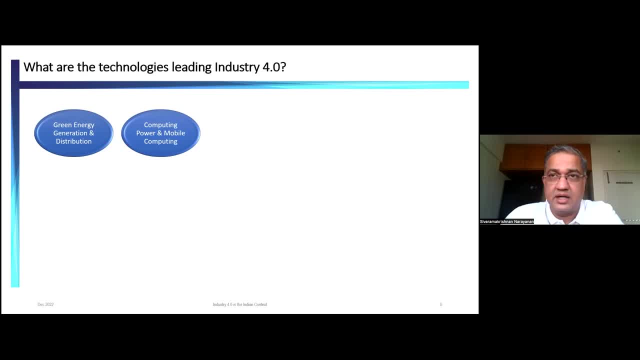 And that's how fast the new generation has taken to technology, and that's how fast technology has made itself understandable to people that don't even know how to read and write. My own parents, of course, on the wrong side of the retirement age, are able to navigate through a complex payment application like Google Pay without any assistance from me. 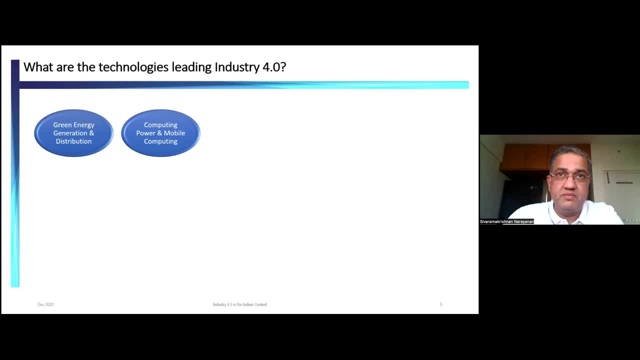 And that's impressive, right. How easy it is for people with no understanding. How easy it is for people with no understanding of how payments technologies work, to use a technology and to make it happen for themselves, And their life is better as a consequence. 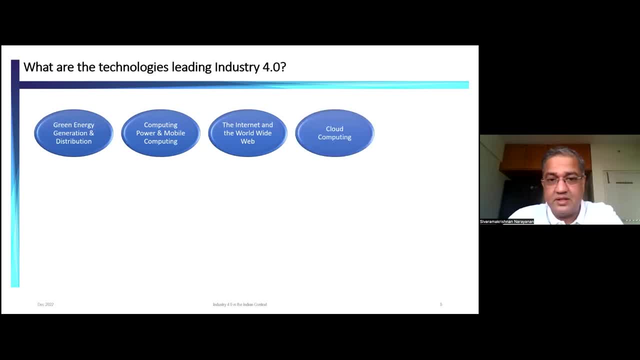 Of course, the internet has revolutionized what we do today: Cloud computing. More and more people want to rent computing space and computing power rather than buy. Things have changed dramatically, And those of you who have been on Twitter in the last couple of days- 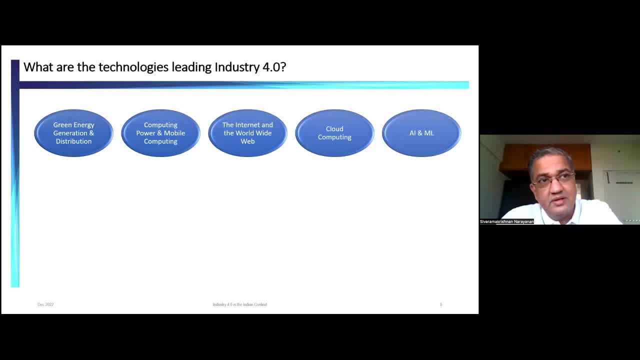 OpenAI has released A new version of their chat GPT and it is incredible to see what people are typing up there. Chat GPT is basically a chat bot, but it is a lot more than chat bot. It is an incredible piece of work. 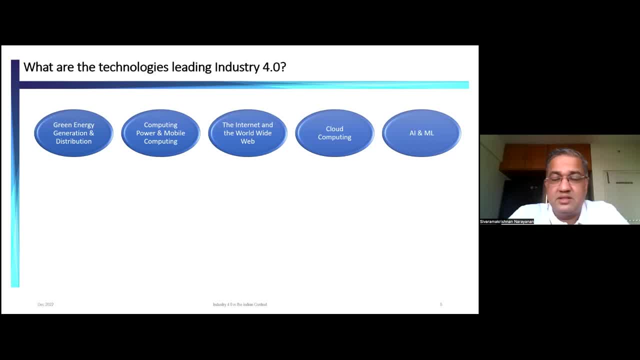 You will not, sitting on the other side of your computer, understand the person that is responding to you is not a person, it is a machine, So it can type for your programs. It can say: You know, make a Shakespeare, make a, make a sketch, a single act, play in the style of Shakespeare and use a modern context, say the prime minister of UK, for example, and you will have a paragraph that looks like Shakespeare wrote about the prime minister of the UK. 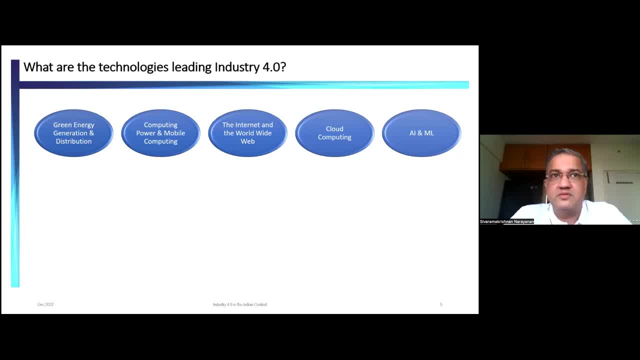 And this is a computer right. It doesn't know who is the prime minister of UK and who is the who is Shakespeare or what is the style of Shakespeare, but it's just been fed an incredible amount of data That it has read on its own, understood it stored it in structures and is pushing it back to you in a way that you, as a human being, can understand. this is about the current prime minister of the UK and it's written in the style that Shakespeare would write. 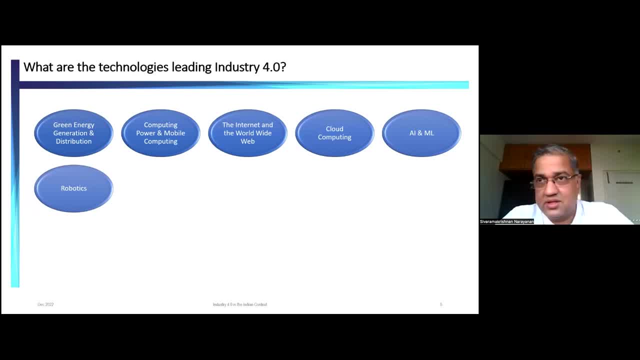 Robotics. we've seen it in the caricature that I've put it up in the first slide here today, and we have seen several factories, whether it be Amazon warehouses or automotive factories, or Factories, Factories that assemble pharmaceuticals you know for for global supply and distribution. as we've seen in the Corona phase, robots are almost entirely- you know, almost- invisibly- taken over the shop floor, right. 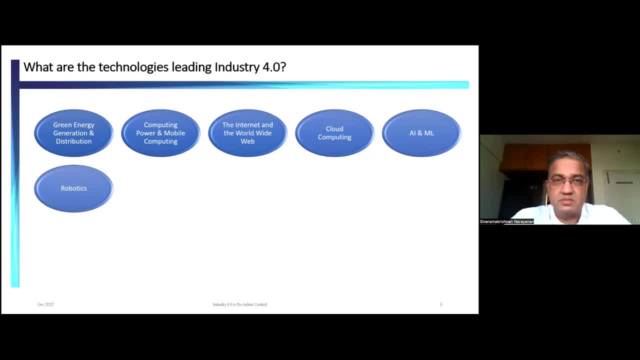 There are so many robots today that do applications that human beings were doing not so long back dangerous things, things that fatigue a human being beyond a certain limit. robots are able to do them tirelessly. Of course there are safety issues. Of course there are power consumption issues, but the efficiency and the productivity gain far outweigh the costs of these things. digital twins: right. 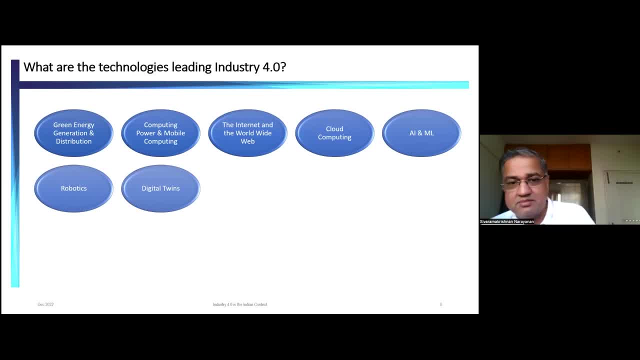 Sounds sounds like a biological term, but it's actually something that has taken off in the recent past. You know how can I use the data that comes out of the everyday actions that we do, whether it is procuring stuff, Manufacturing, 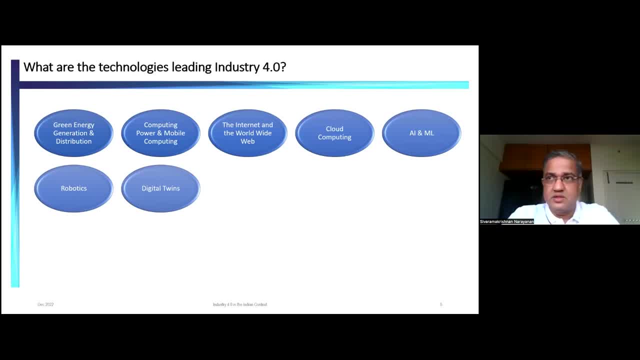 Things, distribution of things: cars, pharmaceuticals, you know Amazon, books, whatever you buy, excuse me, You collect data. you collect data about the location of where your components have gone. where are they coming from? Are they delayed? 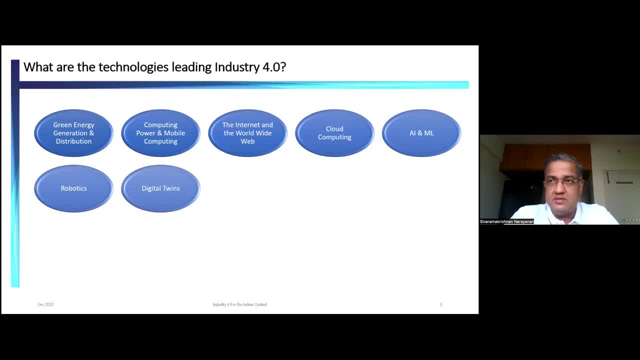 Are they on time? Are they of the right quality? Are they not fitting you because something went wrong in the process? Various things, which are data that were earlier What we can call dark data, which is data that we did not know how to use, or data that could not be used today. 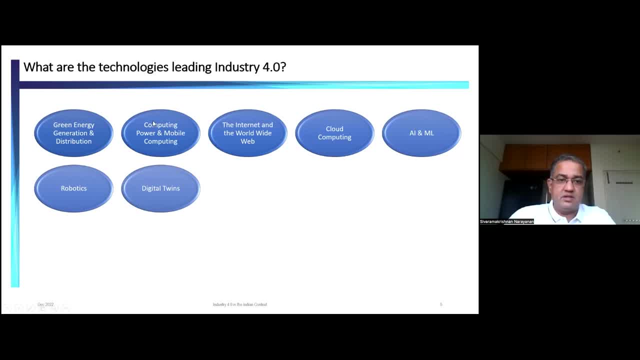 That data is possible to be used because we have the earlier aspect of computing power. So the digital twins helps you make a model of your physical world. So it's a twin in that sense and it works with data that you have generated in the past. 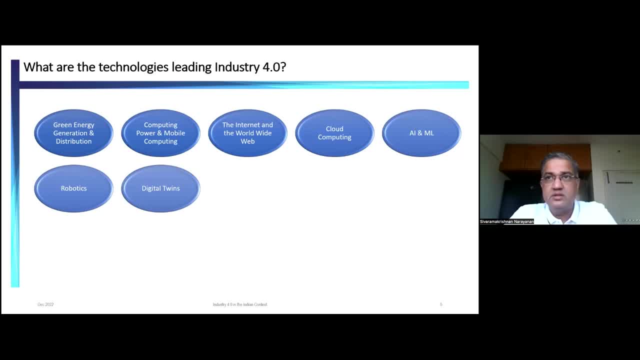 So it is your own information, So you're actually cloned, You're physical, You're digital infrastructure- into a digital system and then, using a process of and that sits on the cloud, and using a process of machine learning, you are able to understand what went wrong in the past. 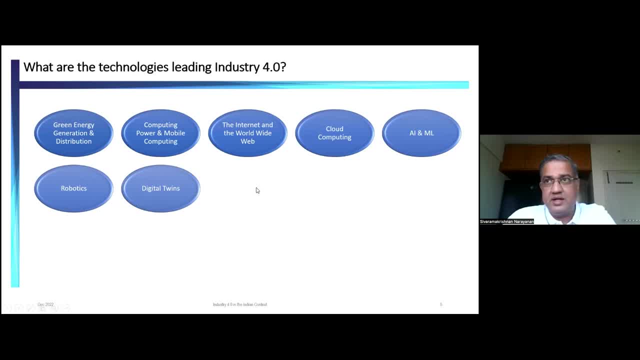 Imagine if all that data that you had, you could actually predict, using some modeling, what would happen, you know, and what is the confidence level with which you can predict what will happen. Right, So if this upstream machine failed, what is the likelihood that I'm going to fail? 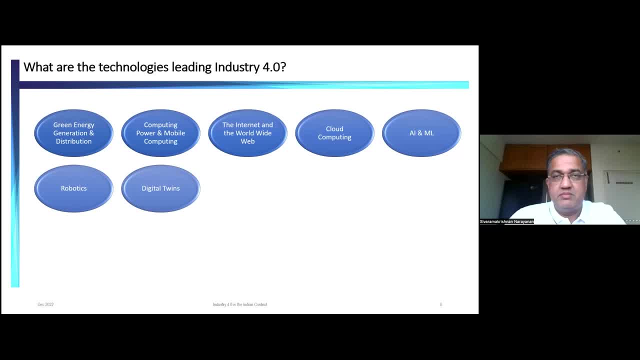 Right. So if this upstream machine failed, what is the likelihood that I'm going to fail? Right, So there's the likelihood that I will have a problem somewhere downstream. If this went down for maintenance, what is the impact that it would have on my capacity? So you can make these models in a far easier, far more simpler way, Because, just like I gave the example of Google Pay and the elderly generation, it is possible for a less computer savvy person to use these models to understand what is likely to happen and make a business intelligent decision that way. 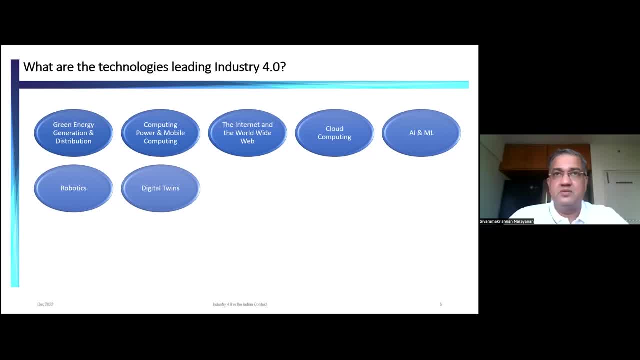 Right, not so long back was, you know, behavior at the workplace right And we normally assume that when somebody comes into work they come with the best intentions, right, They want to do the best, they want to deliver the best for the organization and so on. So if you put the factors that they can, 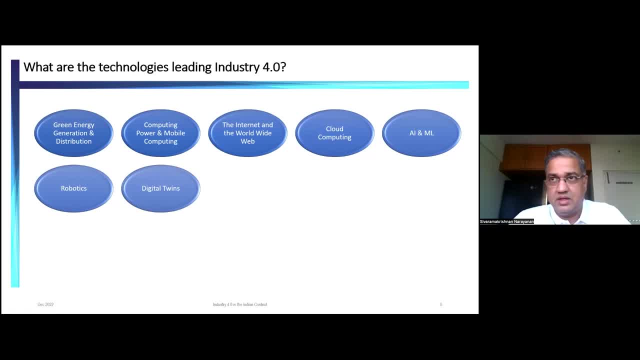 work with. if you put them, give them parameters on which they can make a good decision, more often than not, your expectation is that they will make the right decision. They may get overwhelmed because of the amount of data that they have to process. 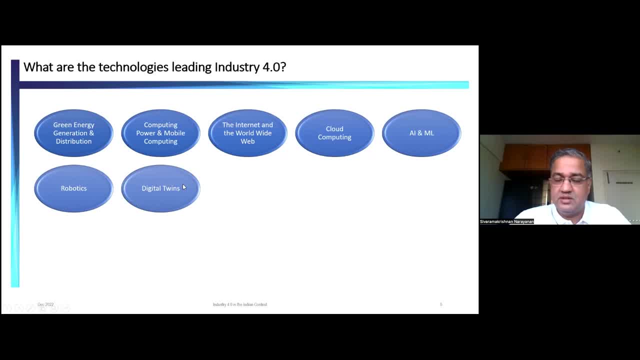 But if they understand it and if they're given it in a simple enough way, they will make a good decision. So some of these things are basically helping the human being at the center of it all to understand and to take actions that are meaningful and that are beneficial for the 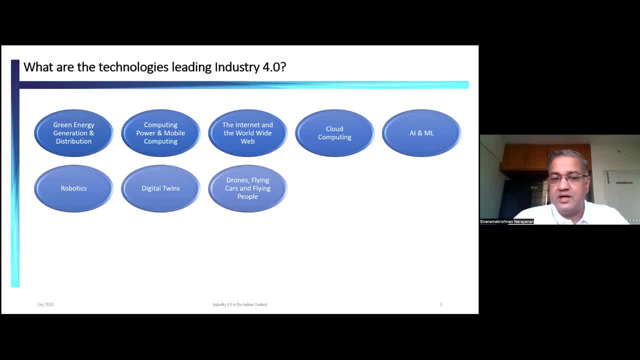 organization in the long run. Drones flying cars, drones- we have seen A lot of companies- DHL, Amazon- they are piloting drones, They are piloting drones, They are piloting drones. India still has to have a policy on drones Flying people. I mean, we have seen Iron Man. 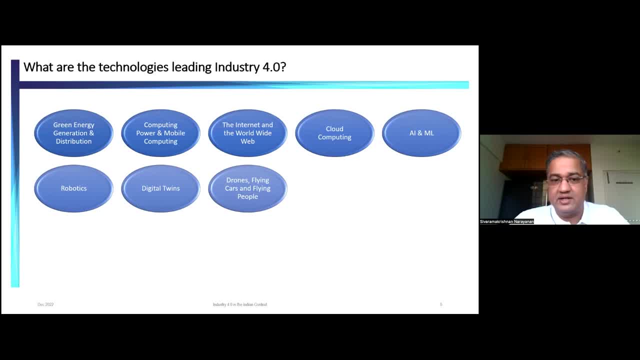 of course, in Marvel, but flying people are not yet a reality. Flying cars are fast becoming a reality, Though I shudder to think, with the conditions of Indian roads, how flying cars would be in India. But as an aside right, I'm sure we will find the policies and the frameworks. 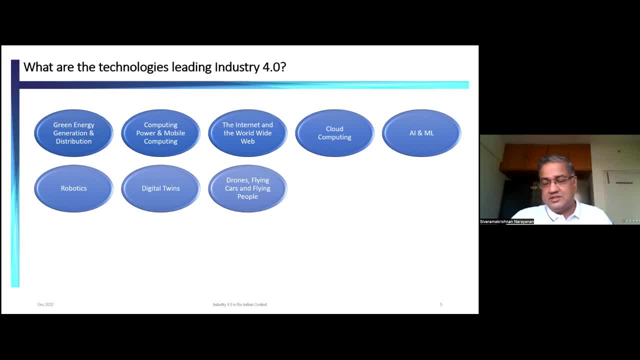 that will help manage this, But it's an interesting time for figuring out how autonomous flight can help our lives become better In India. this seems a little bit far-fetched, so I'm just going to leave it there as one of the elements that is coming in. 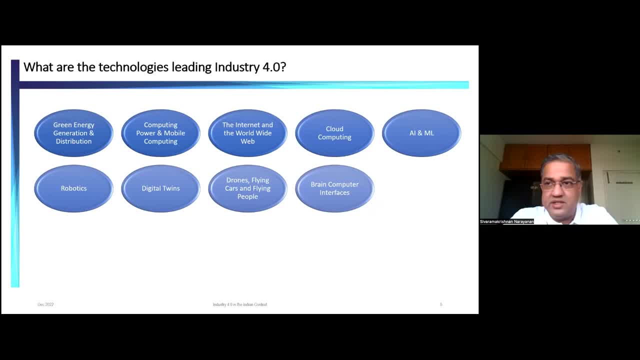 Brain-computer interfaces. You would have seen recently the owner of Tesla, Mr Elon Musk, talking about some technologies around this. There are videos on the internet, YouTube- where a paraplegic man kicks off a football. You know great, A football tournament in South America- Unimaginable a couple of decades ago. 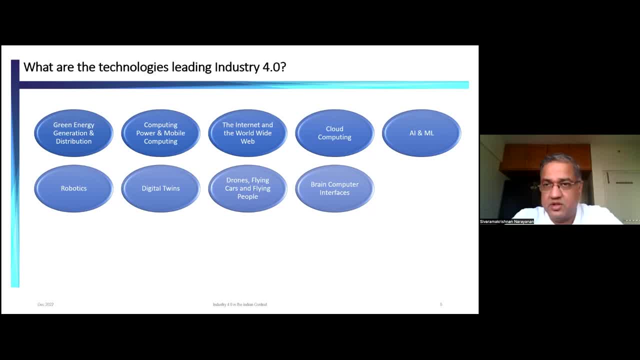 And he controlled his limbs. He couldn't move his limbs, arms or legs because of an accident, And he was actually controlling his lips using an exoskeleton that was hooked onto his brain. All right, So imagine the quality of life that is possible by providing some of this in a more 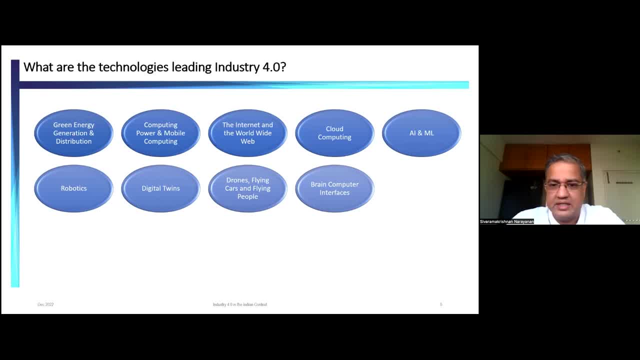 mobile fashion Right, And we will get there, I believe. Virtual and augmented reality: A lot of us are hearing about metaverse. I, for one, I'm still confused as to how this can be used, But we are already seeing some practical applications, like self-driving cars, for example, is one of the 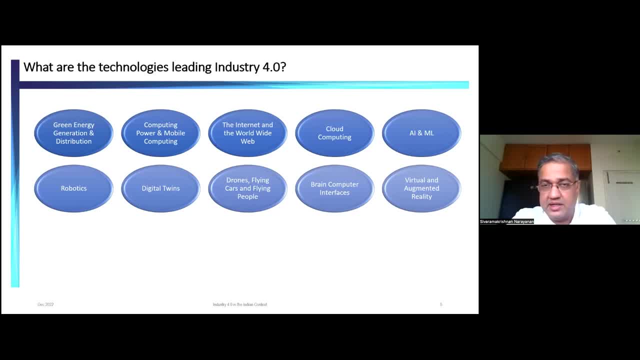 examples where augmented reality is making this a reality today in various Western countries. Also, when a worker is actually managing on the shop floor, she can actually look at various warehouse shelves, understand what is the product. they're using a combination of augmented reality, RFID and whatever business application they are running. 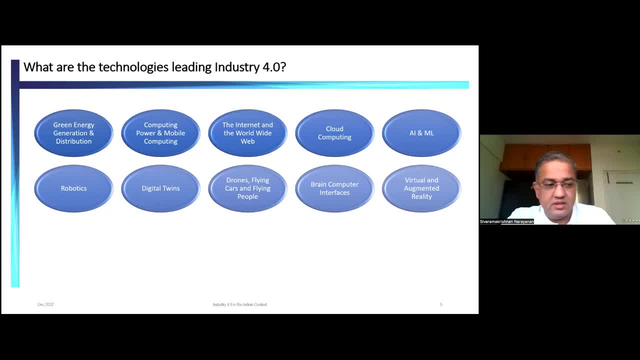 in the warehouse. So it's possible for even today, using Oculus or Google Lens or any of these technologies, to identify what is happening in the shop floor, And this is a reality. tool Additive manufacturing or 3D printing: I will talk about this a little bit. 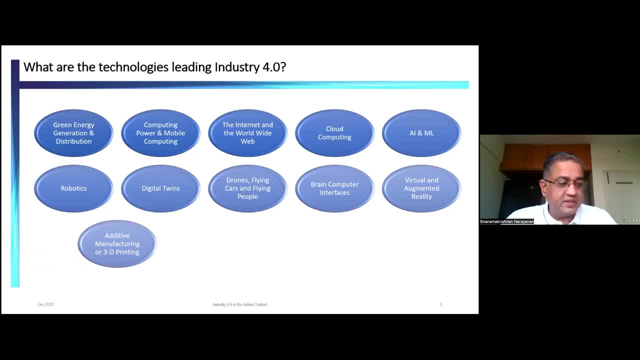 later, But I think it's a very important thing And I think it's important for us to be able to do this. So let's talk about a couple of companies that I have the privilege of being associated with are doing something that is pathbreaking from an Indian society point of view. 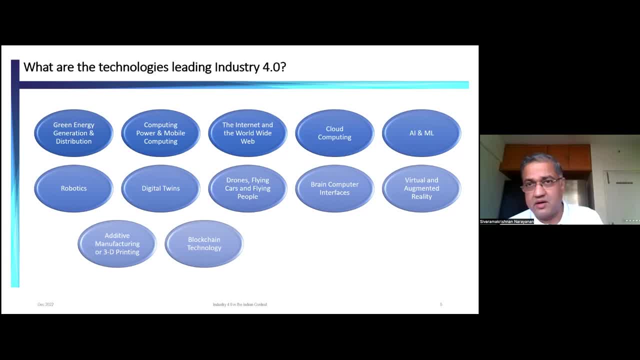 Blockchain technology. We hear a lot about this. This has been an experiment. Of course, it does involve some bit of regulation, but not in the fintech area, which is where we are seeing a lot of bubbles and bursts in the recent past- crypto and whatnot. 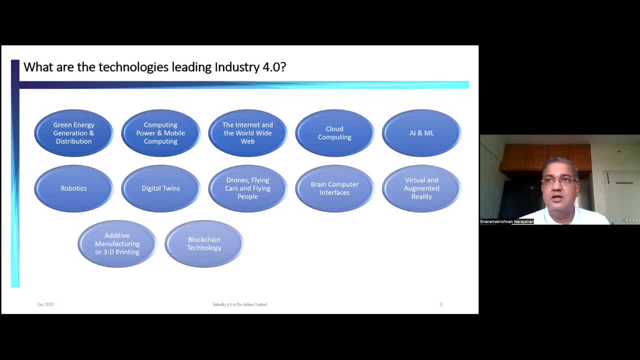 And we are seeing a lot of these things happening in domains like automotive spares, in domains like pharmaceuticals and so on. So I'll be talking about it a little bit too. Biotechnology, like I mentioned a little while ago, it is one of those areas that has come. 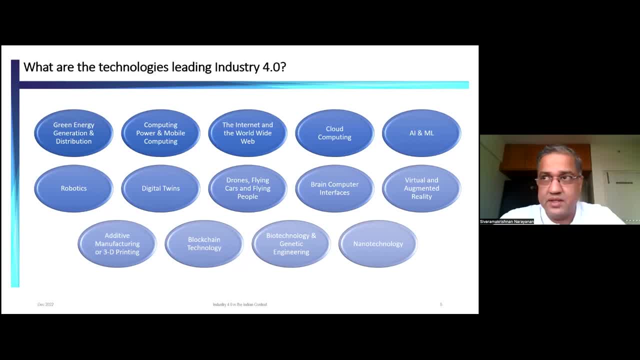 very close to engineering and manufacturing these days because of the kind of combinations of technologies that we can bring. What used to be earlier a very pristine terrain only a few people can get in has become a more generic, more democratic area for people to participate. 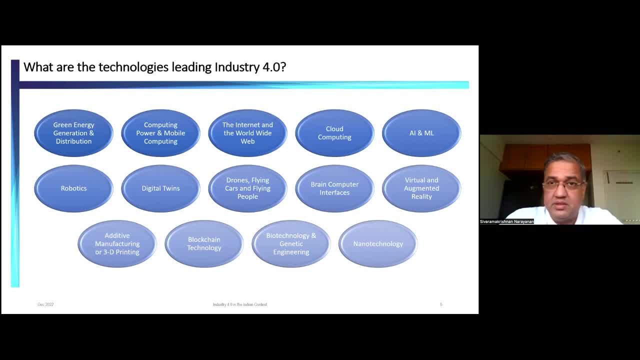 And finally, nanotechnology. a lot of research has happened in the last several decades in nanotechnology. Now we're seeing slowly the packaging applications of some of these things enter into even the Indian industry, because one of the things that the government has over the last couple of decades is how can we use the productivity and the gains? 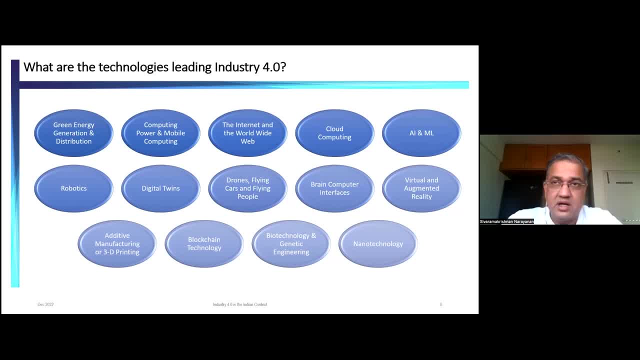 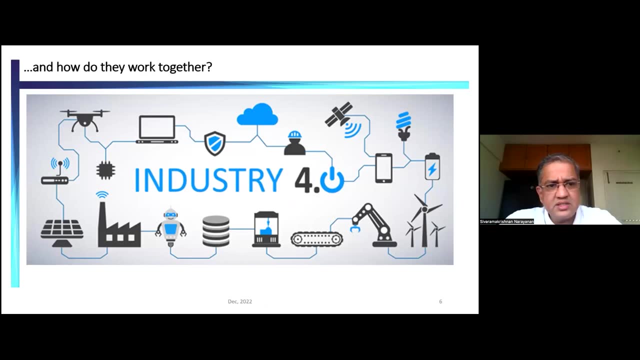 for the agricultural sector, given the large number of people that are employed there, and food processing was one of the thrust areas for several years across multiple governments, and nanotechnology plays a part that. how does it all work together? right, i think i've touched upon it a little bit krish, we've lost you, okay. uh, it is possible for us to take green energy. 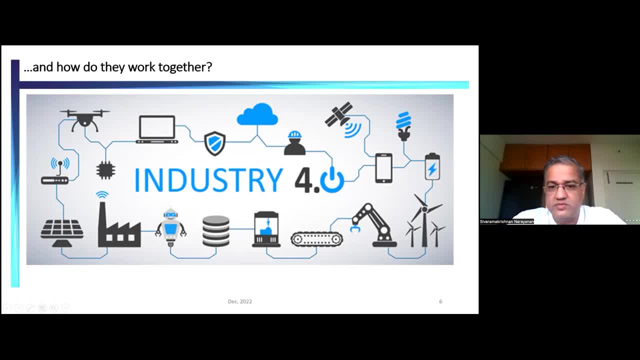 on this side what is represented as a set of windmills into battery technologies. right. so we are seeing the explosion of battery supply chains in india. even as recently as today morning, i was reading: amaraja batteries is planning to set up more units in talangana. for, you know, not just 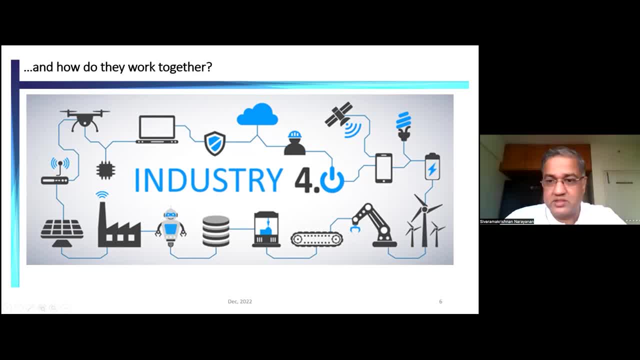 batteries, but also battery swap infrastructure. of course we have cfl lamps and so on, the mobile phone and the internet that we have seen here connecting up people and the machines that run drones and the factories and the robots that sit in the factory right now. if you imagine um this for a bit, it is not just the big blocks. 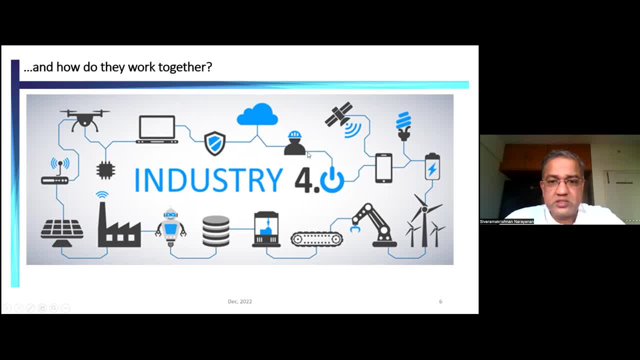 of course, this is the security aspect of it. it is not just the big blocks, the people, the security, the computers and the drones, but these lines that are actually connecting these various technologies together that are important right now. just imagine if these were all just to kind of relate it to our everyday life and if this was a cross-section. 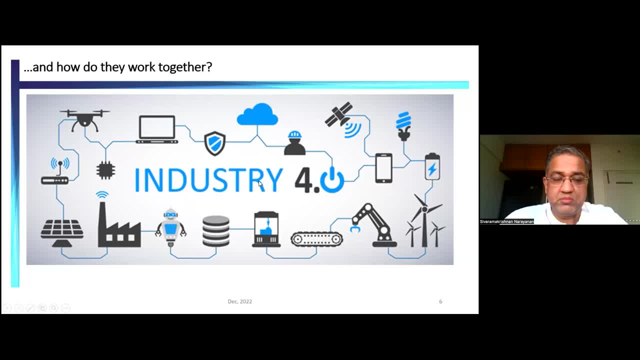 of an indian society, an indian state where there are people from multiple regions, multiple states of india living together, and somebody speaking odia and somebody speaking hindi and somebody speaking assamese, and they don't have a common language. they don't have english or hindi or any. 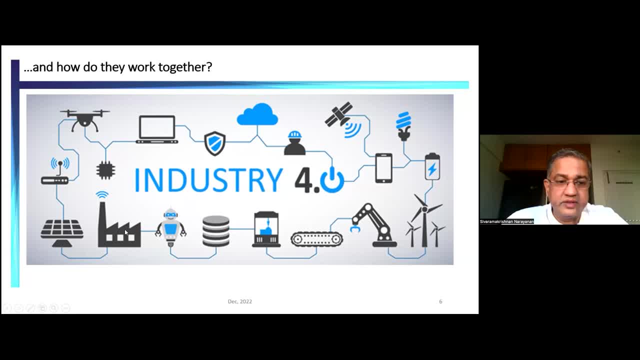 common language that they can talk to each other. imagine how this communication would be right. it is. it is going to be hard. they're going to be, you know, trying to understand each other, and then the next person is going to be the other person, and then they will have additional interpreters sitting here and there which are trying to 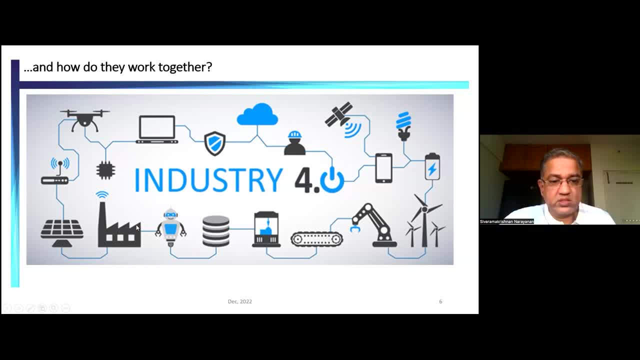 understand from both and then telling the other guy what the first person was talking here. these lines, this common infrastructure of data transfer and integration, play just as much an important role as these objects themselves. right, so for us to understand this. uh, the one one network, open network, digital commerce that the government is launching. 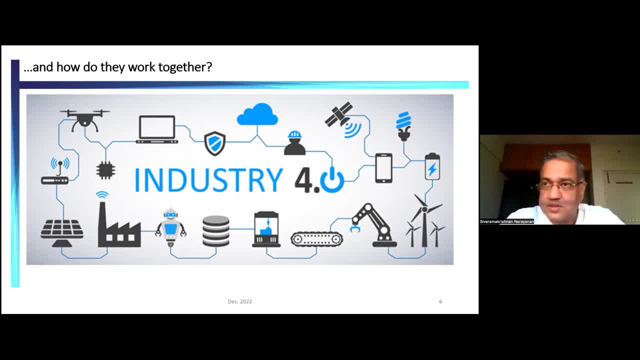 industries- or, you know, almost micro industries- hooking on to this big network and being able to transact anywhere in India with people that may not know the language, but the computer knows what they're talking about. they know whether they are buying a piece of fabric, which this is not. 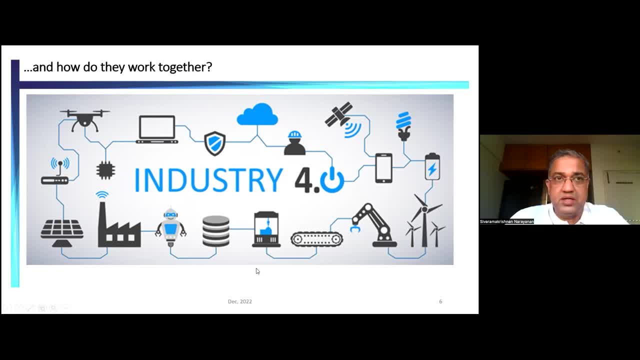 available in their state or whether they are buying a machinery part which has a sophisticated amount of technology that they want to evaluate and take for themselves. so each of these components, including the lines, is important. the data transfer across these and the standardization of the data flows across these different elements of the entire industry for network is very, very important. 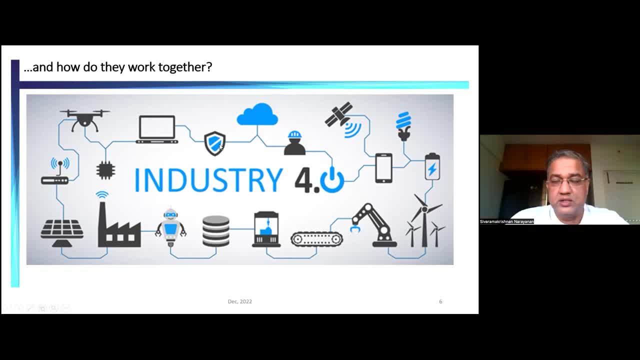 and most crucial is the part that says you need to be, you know, controlled by a secure layer at the end of it. security that you are not losing your ideas or your intellectual properties or even your data, simple things like your date of birth and your gender, and so on and so forth- to 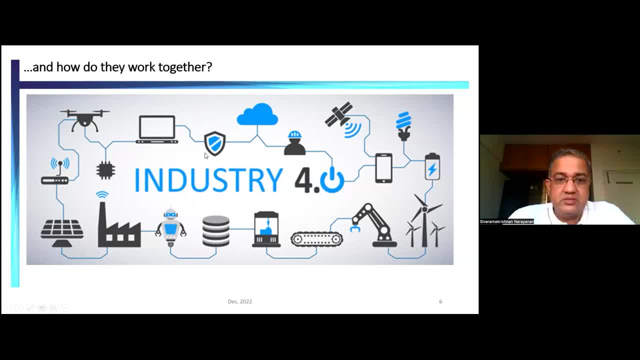 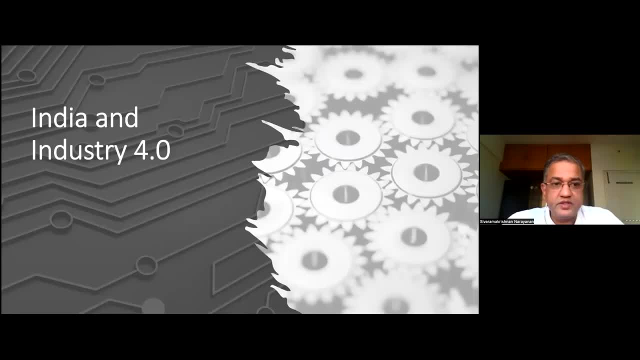 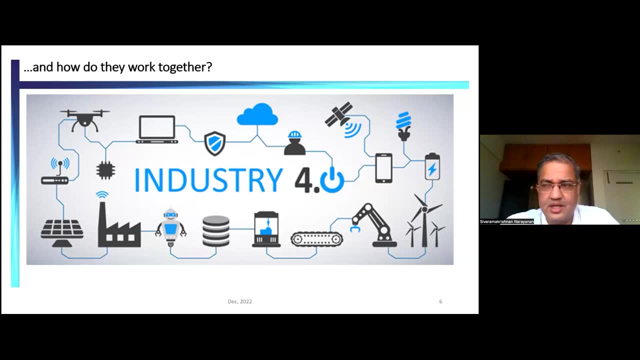 fraudulent people. that is something that is very crucial, and here is where I think the biggest challenge will be as we move forward right? so this is broadly the industry for you. what are the things that go into it, how they are likely to work, what are the important? 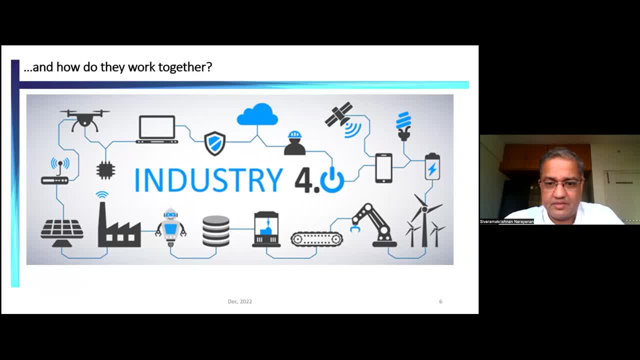 dimensions of this whole architecture, and I'm talking at the industry level. so the architecture is a little, you know, brief and it's a very line diagram kind of architecture, but there are certain dimensions that we can deep dive into as we go through this discussion today. right, I will quickly walk you through my perspective, my point of view on what 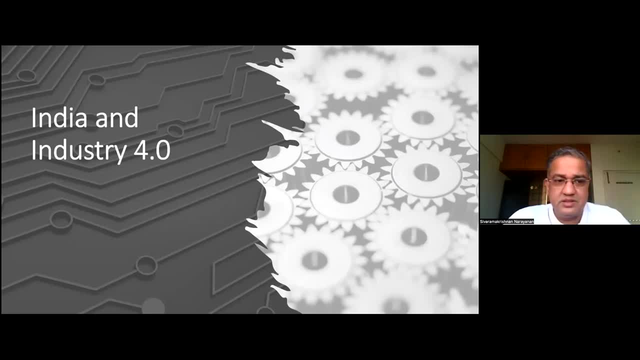 industry. for what is it? where bend and lay are, where there is sort of an area of expertise, where, how do we- well, I как минимum if I give some kind of teamwork to your thinking- between the two of the panel destroyers through door to door? 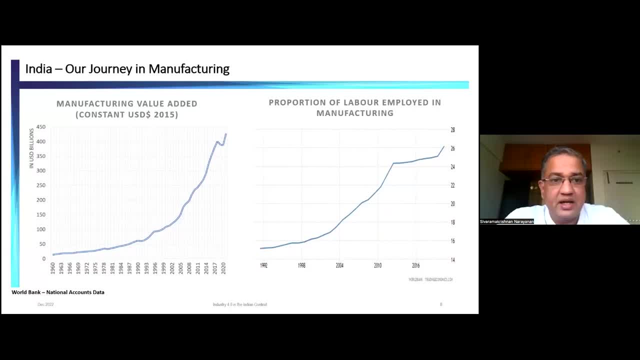 date. if I look at it, you can see that the manufacturing value added at constant US dollars, taken at 2015 rates, has been on a steep incline upwards right. The proportion of labor employed in manufacturing also has shown a steep increase right, And both these are coming from World Bank. 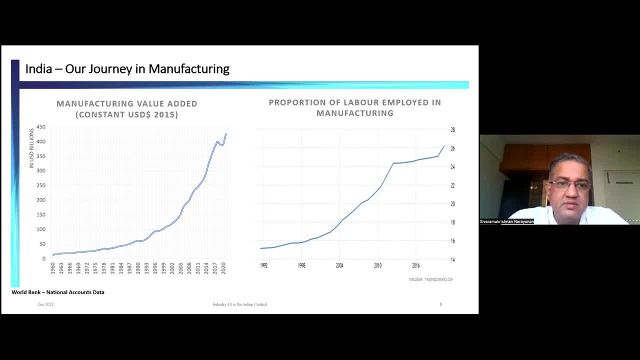 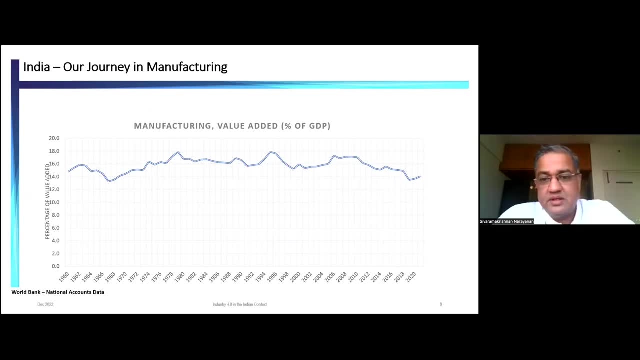 national account data, So it's publicly available. You can source it anytime you want. But if you look at the share of manufacturing as a percentage of GDP, you know the story is very different. The story is that we have been stagnating at around 15 to 17% in that ballpark. 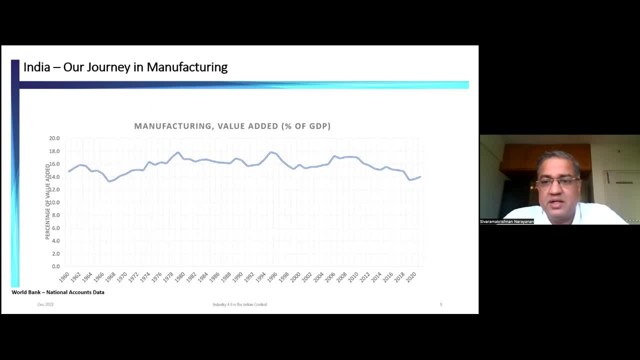 forever. You know, for the last 50 years we've been at the same rate And we are, you know, marching. So the perception is that we are marching towards a $5 trillion economy. But manufacturing is somehow probably not got the memo right. So there are still. 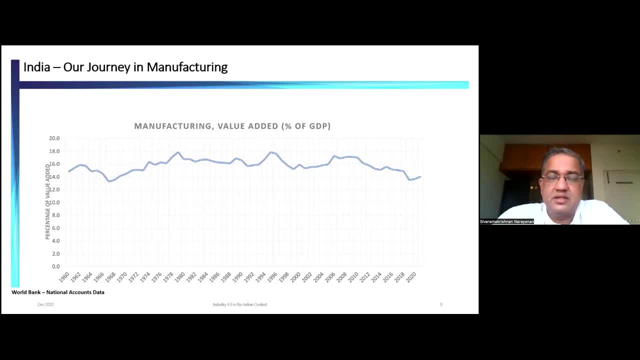 bottlenecks. There are still challenges- Real challenges, some of them imaginary challenges- that we need to overcome as a country right And as we work towards overcoming them. the possibility that manufacturing alone will contribute about 25% of the total value of $5 trillion is a real possibility And we stand at. 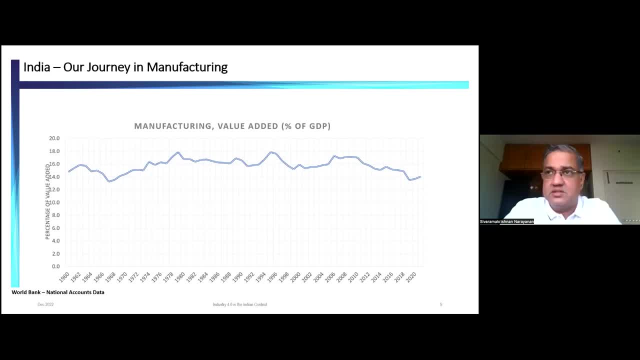 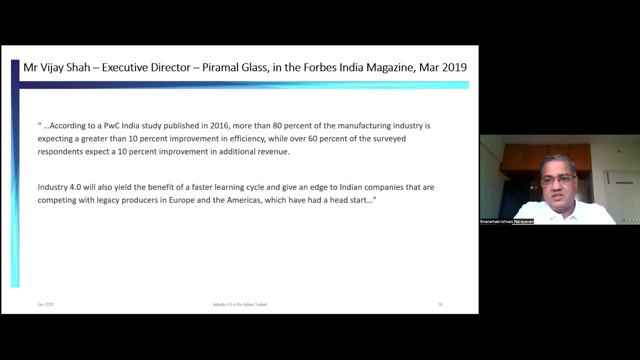 the cusp of that, And there are multiple factors that are giving us this advantage, And it is good for us to be able to overcome them ourselves. What are the disadvantages that we have to overcome or the challenges we have to overcome? So this is from Mr Vijay Shah. It's a direct quote from what 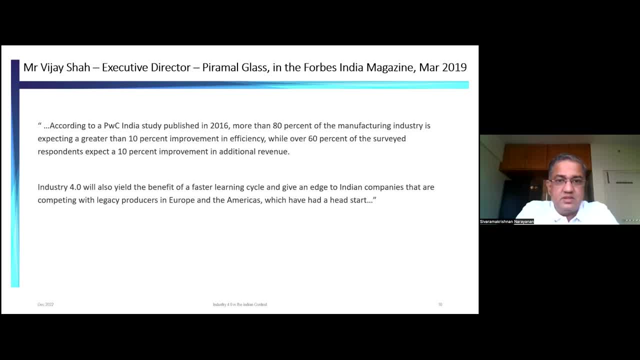 he gave an interview in the Forbes India magazine in March. He's the executive director in Pyramid class. So this is the expectation, right? The industry expectation is 80% of manufacturing industry is expecting a greater than 10% improvement in efficiency And people are expecting: 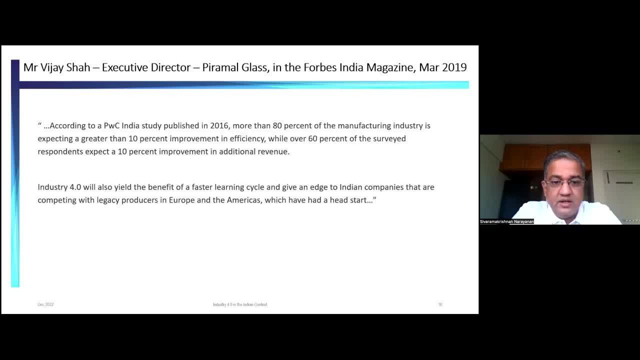 10% improvement in additional in revenue. right Industry will also- industry 4- will also yield the benefit of a faster learning cycle. So there are a lot of expectations. right Faster learning cycle. we will compete with the legacy producers in Europe and America who are already having a. 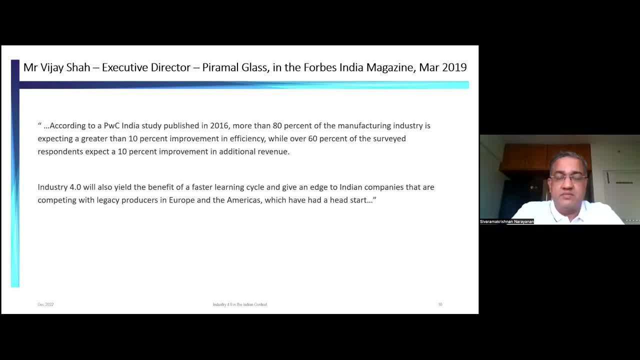 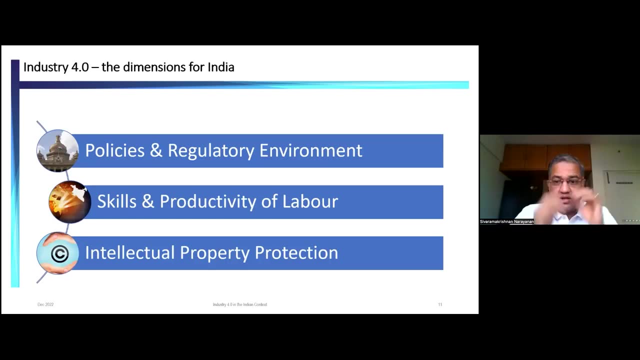 head start and so on. This was pre-COVID And obviously industry 4 in India. even today, because of the pause we had on COVID, we are still starting blocks, so to say right. So this is the expectation. So, if I just dive down a little bit, 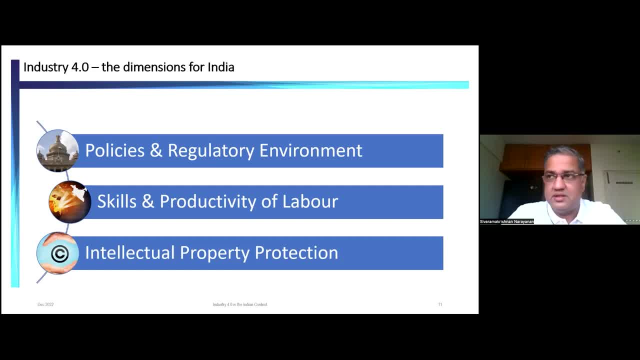 and say: what are we looking at? okay, broadly speaking- and this is the section where I told you that we will talk at a high level initially and then go down to industry examples- So we're talking about, broadly, three areas: policies and regulatory environment, skills and productivity. 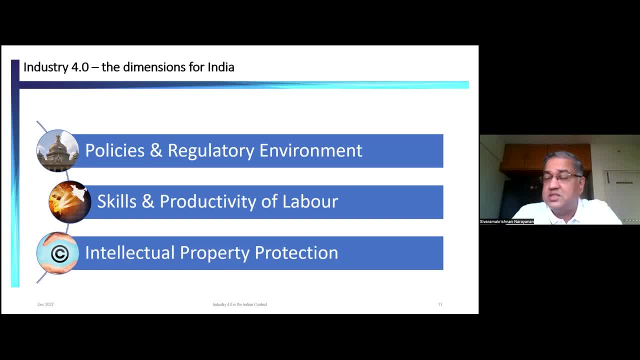 of labor, because that's a very key aspect of the nature of the market that India is. India is a labor. We are not a labor deficient market, We are a labor excessive market. at this point in time, We have more disguised unemployment in 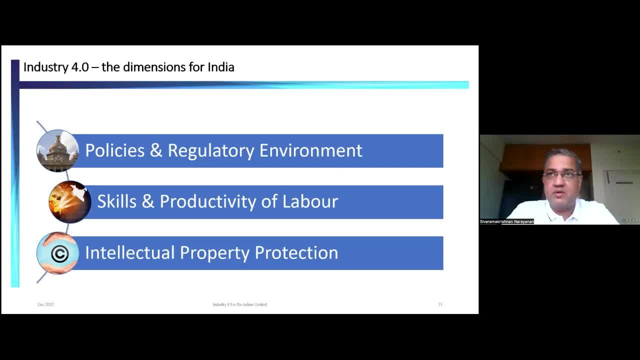 multiple sectors, including agriculture. More people are employed for doing the work of one person, So we need to understand how we can- excuse me, I'll just have a sip of water- And, more importantly, how we can protect the intellectual property that most companies in. 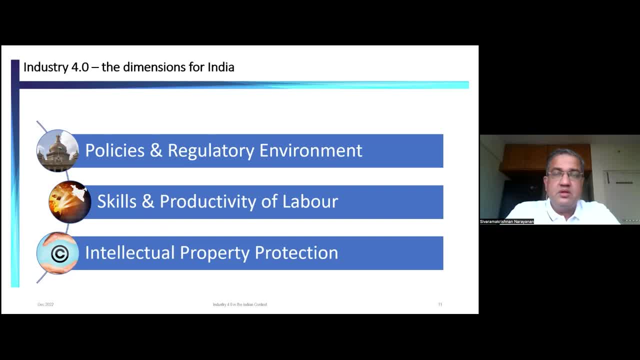 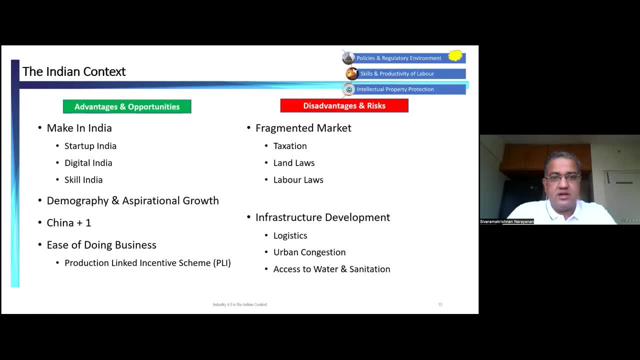 the world are bothered about, right, How they will control and they will make sure that their IP rights are protected. We will talk about this in a little detail. So the first. I've broadly broken this down into two, So let me just 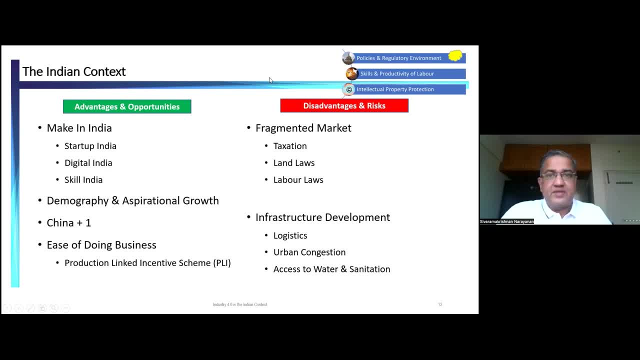 move this on this side a little bit. Yeah, So when we talk about the Indian context and the policies in the regulatory environment, on the left side of the slide today, we have the various advantages or the opportunities for ourselves And the design of the system. the design of the system, the. 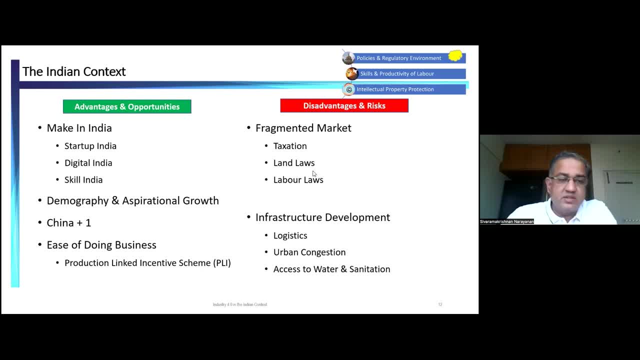 advantages here, And the next two or three slides will go in this fashion. So the first thing is we have a very conscious effort from the government to kind of work on a make in India policy, right? So this is one of the points that was raised also in the IIT ACB manufacturing conclave. a couple of 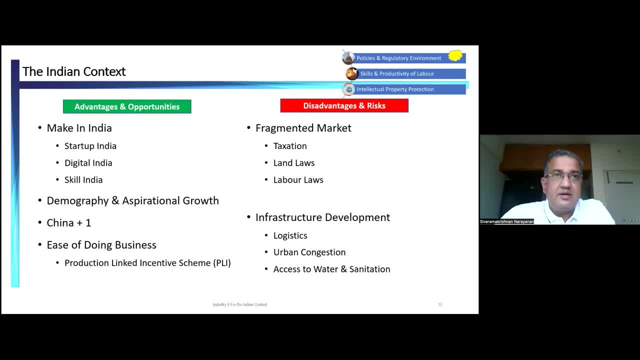 years ago. Should we make or should we buy? And one of the panelists was saying that it's easier to source from Thailand, which has a free trade zone with India. Then it is to source from Roper as an example, right? So thankfully we are moving more towards. 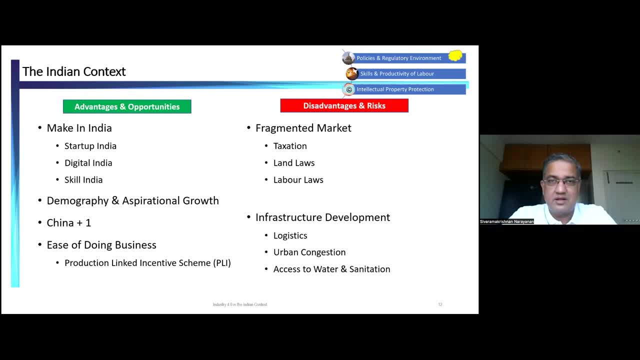 a make in India policy. We are trying to see how we can improve, but more can be done. more should be done, But we have make in India is hopefully an umbrella program- at least to my eyes, it appears so- which also encompasses startup India, digital India and skill India as multiple programs and 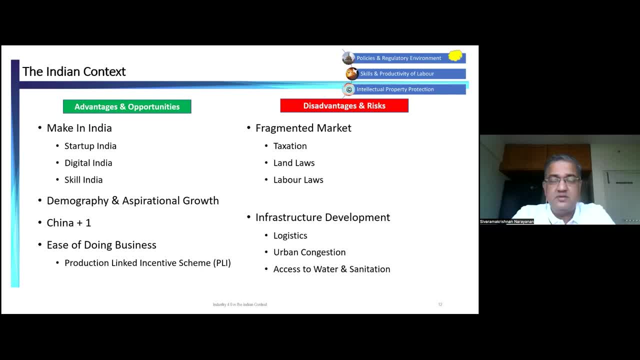 initiatives that the government is working on. All good with the right intentions, but we have to agree and continue to do things with little attention, or a little extra tiny attention, which is tapping into the demography and the aspirational growth that we see. So the demography and the 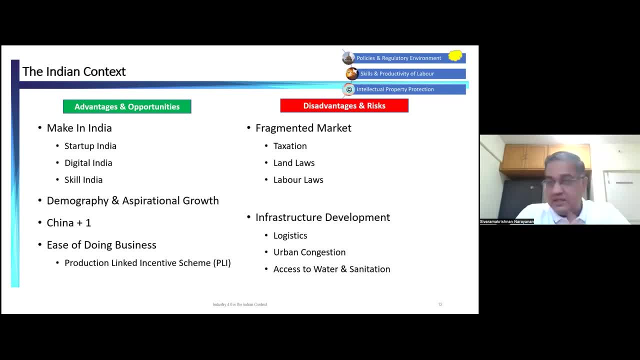 aspirational growth. We must have heard about the demographic dividend. We have more people that are coming into the workforce on a monthly basis. these days, almost a million young men and women enter working age every month. That's the kind of scale that we are talking about. 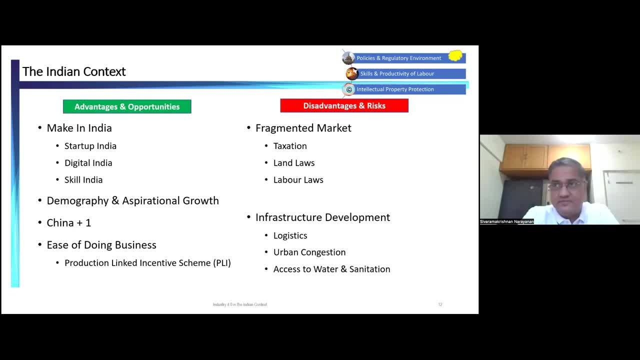 more companies are looking at alternates to China. So China plus one. there are a lot of articles out there which tell us that, you know, India should be in the forefront of China plus one. Some companies have moved, some companies haven't. At the moment there are more companies that are. 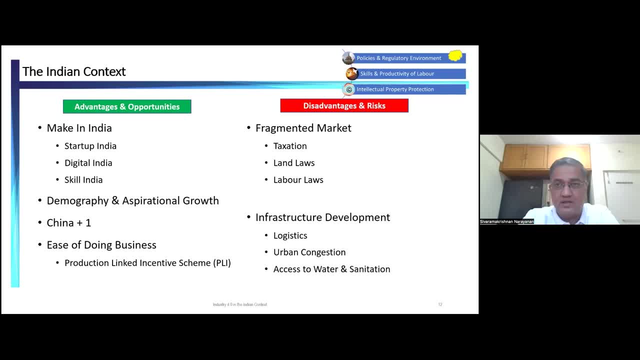 selecting countries like Vietnam and Bangladesh and other parts of Southeast Asia over India. right, And there is something there we need to look at very urgently: Ease of doing business. we are improving the production linked incentive scheme is making life a little bit easier, But 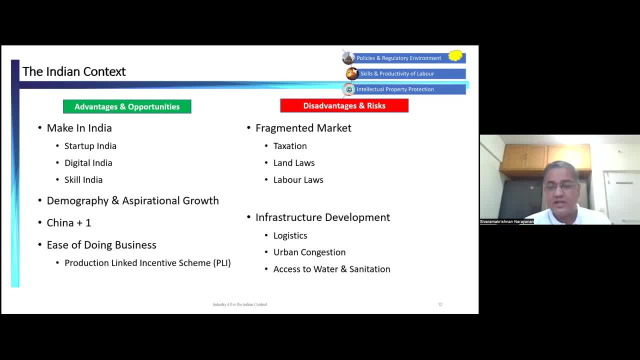 there are also critics of the PLI Right. So while there are advantages, there are some more improvements that is possible in these policy actions. But of course these disadvantages and risks are well known. We have been a fragmented market for a very long time. Taxation laws particularly. 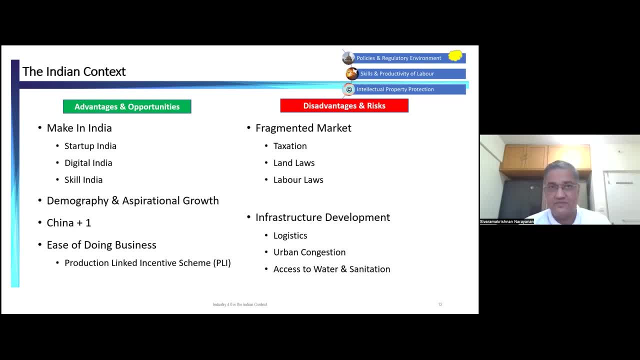 till the GST came into place were quite difficult to navigate in the Indian context. It has. it has improved a lot. It has improved dramatically after GST. But there are also some disadvantages, some points of criticism on the GST which, which the government is hopefully 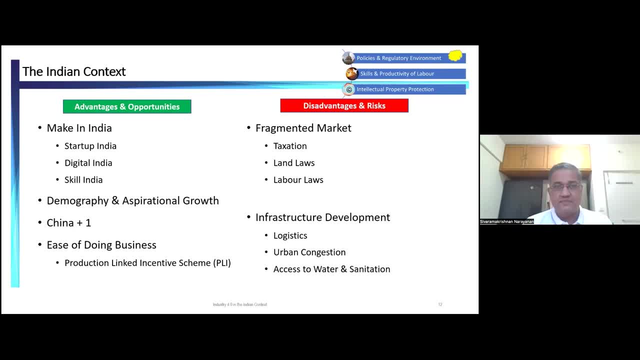 looking at Land laws and labor laws are the hardest ones because they are they affect a large number of people. So there is a lot of, I would say, multiple points of interest on both land and labor which the government needs. 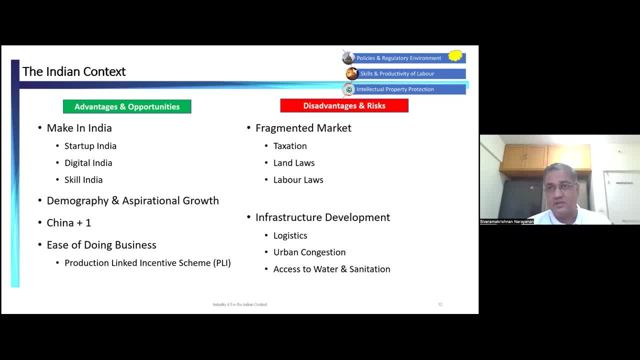 to navigate, which also the industry needs to you know, understand and sensitize the government, So that there is a win-win for all the stakeholders concerned: people that own land or the workers that the industry is interested in and how we can hire and how we can let go. 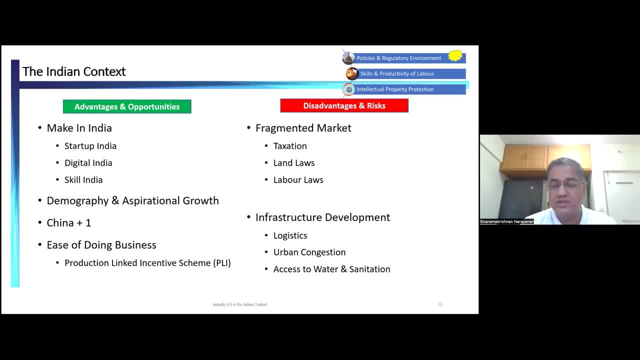 of people. you know so that, but their futures and the economic safety of these people are not affected. So there is a lot to do And today, because of these fragmentations, there is still a bit of hesitation about industry and they demand that the government take care of a lot of these actions on their own. 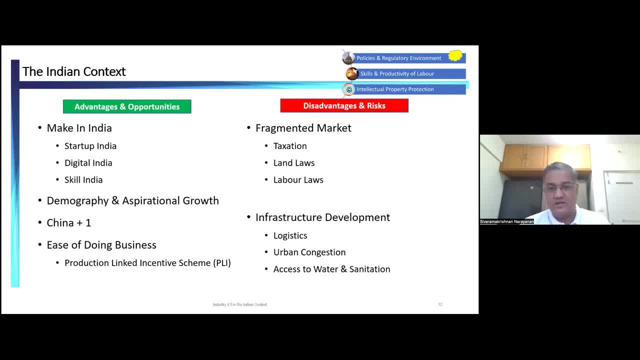 because coercive power only remains with the government right in a democracy like ours. Of course, infrastructure development has got a huge fillip in the recent past, but there is always a but. Logistics are still a challenge. The cost of logistics moving goods from one town or one industrial center to another. 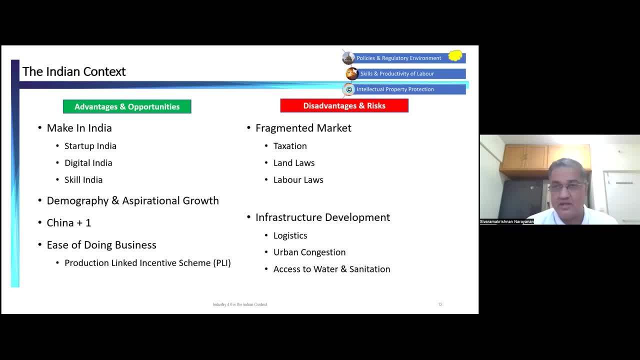 is anywhere between 50 to 70% costlier than any other comparable country in the world. Urban congestion: we all live through it. A lot of us are urban dwellers And there have been many days where each one of us would have thought how nice it would have been if I could just go. 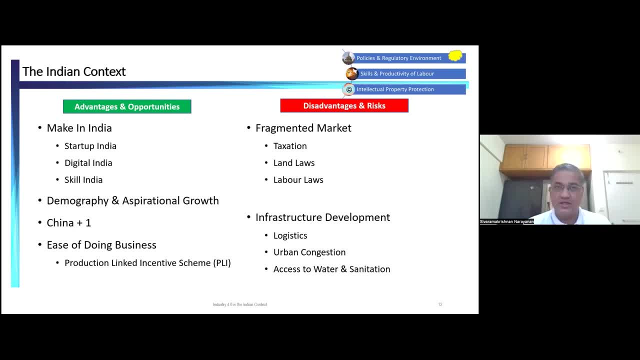 and emulate Mr Sridhar Vembu. settle down in Tenkashi or someplace and, you know, build a center there, where I'm far away from the city. But no, today urban centers offers the most economic opportunities. 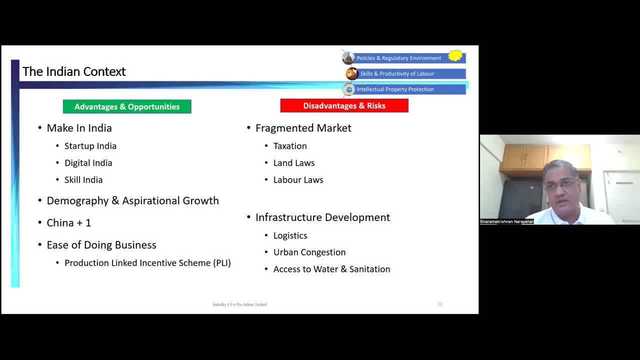 So people still migrate into urban centers rather than out of it, And this causes a real problem. It causes an excess employment in the cities, It causes a deficiency of employment- formal employment- in the rural areas or semi-urban areas, And this remains a challenge. It will continue to remain a challenge till infrastructure is at rest. 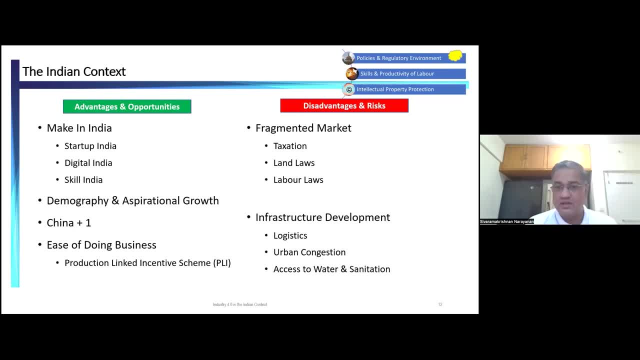 And, of course, access to water and sanitation right. This is critical Again. a lot of this has been done, but more needs to be done. These are all huge mountains to cross and it always will take time. There will always be criticisms, but I think we are setting the direction in the right way. 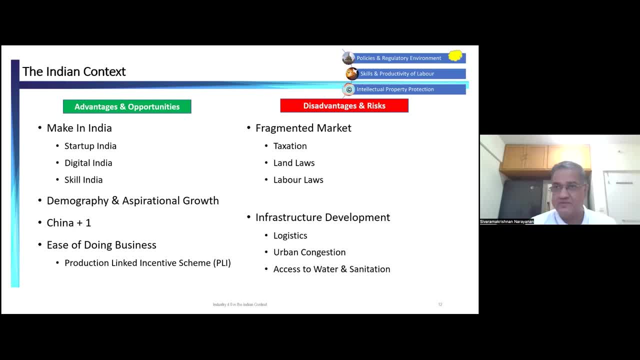 There is a real amount of intent. I'm sure all of us have experienced it in various degrees, but I'm hoping these advantages and these disadvantages will work in our favor. right, The disadvantage is to be mitigated and the advantage is to be strengthened. 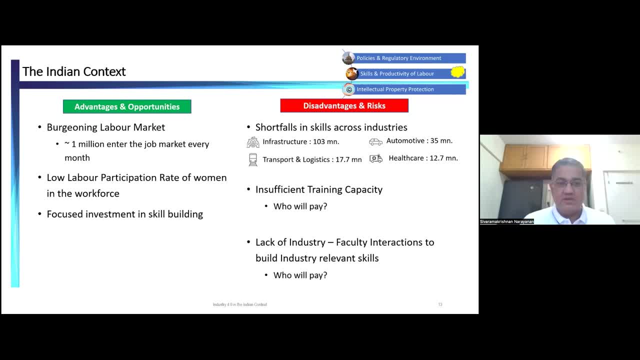 We have a burgeoning labor market I mentioned 1 million enters the job market every month. We have- and I've categorized this very deliberately- a low labor participation rate for women in the workforce right, Which means there is a large amount of women that are untapped, that are probably skilled, that can be employed in. 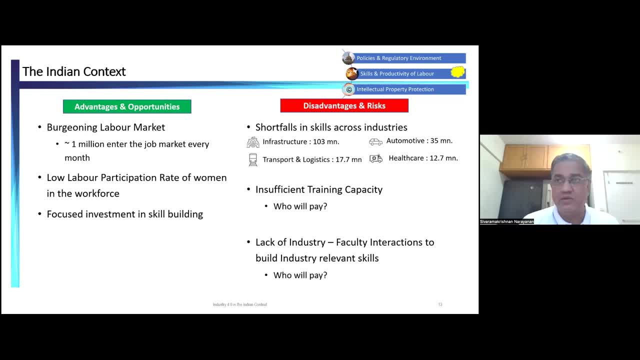 meaningful ways, And I think this is a very meaningful scale work like, for example, assembling a mobile phone, is something that a woman worker can do much better than a male worker, simply because the size of her hands are much finer than a male worker's hands, right. 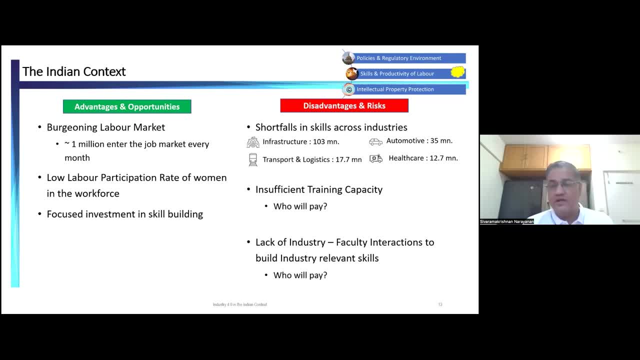 And that's biological, Nothing you can do about it. So there are a lot of these fine electronics, advanced electronic assemblies that could be done and we have a large low labor participation and women in rural India are looking for better jobs, just like men are looking for better jobs. 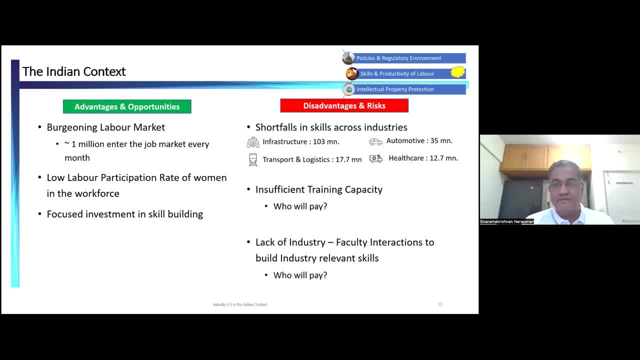 I'm sure a lot of them do not want to do the agricultural manual labor and they would be benefited by a formal employment. given a chance, given an opportunity, And the government is putting a lot of effort and focused skill building right. 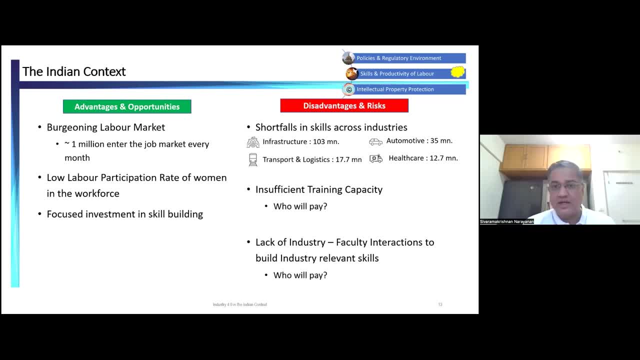 At the same time, there are again mountains to climb. If you look at it, infrastructure alone, which is our biggest problem to date in India. If you look at any foreign report- investment banking or investification reports- they mention infrastructure and not in a positive way, Despite the fact that, literally, 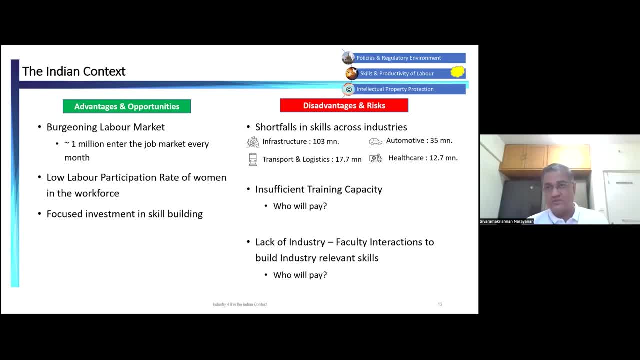 billions of dollars have been spent in upgrading the infrastructure right over the last- I don't know- 30,, 35 years. a lot of investments have been gone have been made into ports, into airports, into road infrastructure, into inland shipping, but still more needs to be done: Infrastructure. 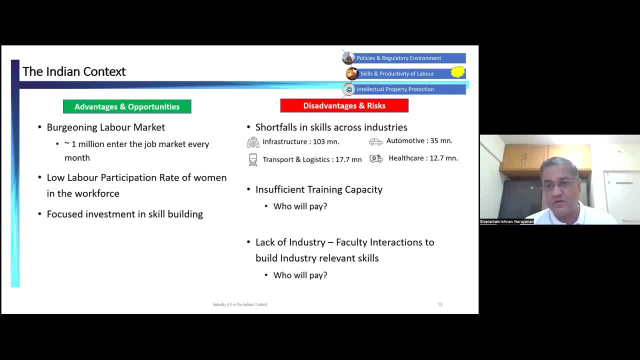 alone has a skill shortage of 103 million people. Automotive: 35 million. Transport, logistics: 17 million. Healthcare: 12 million, 13 million. So if you look at this, you know these are the industries, these are the sectors where healthcare, for example, or transport, logistics, or travel and 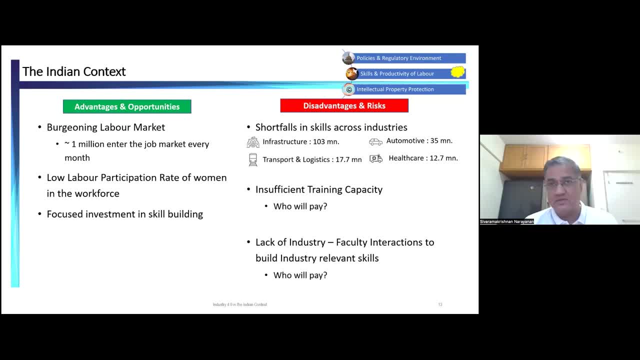 tourism are sectors where women can be employed. You know they are safe jobs. They require a different set of skills which probably a woman will readily bring to the workplace, And it is possible for them to be gainfully employed and grow and have a secure future for 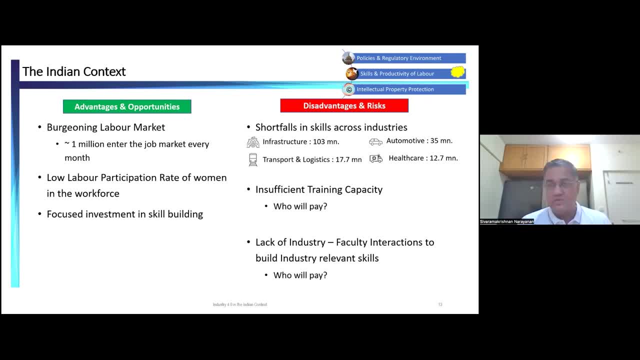 them and their families, obviously resulting in huge economic gains for the government, for the community. But at the end of the day, we do not have training capacity. So if you have a young girl who's coming from a rural area and she wants to become a nurse, she wants to get trained. 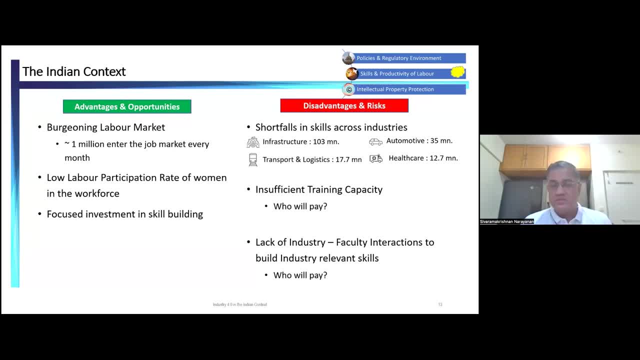 she will have a few institutes. Those institutes you know she has to pay. she has to pay her fees. Or if the institute offers the training for free, who will pay for the training? Maybe she doesn't have the wherewithal to pay for training. So the first question is: will the 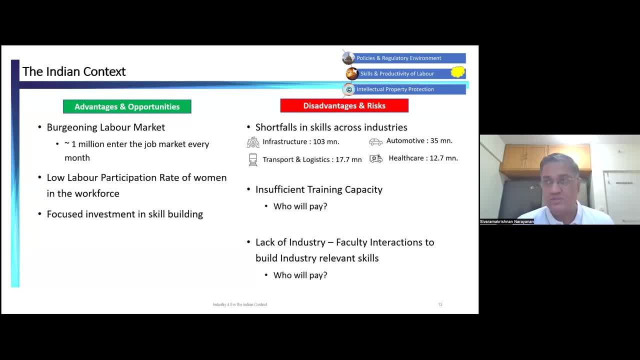 healthcare industry pay? Their answer would be: why would I subsidize somebody's education when I can't benefit from it? And that's a fair question. So the training capacity question on who will pay: who is accountable for making these people skilled and deployable in an industry? 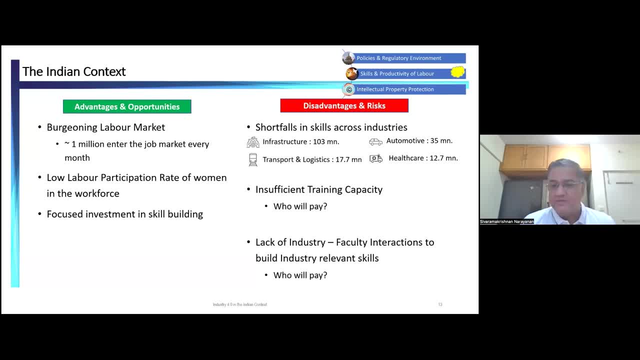 context is very critical: The lack of industry faculty interactions. Now this is improving with platforms like this, like the one we are in today. But can academics, academia and industry collaborate? The answers are found already. You know some of them I will talk about today. But the question remains for these industry faculty. 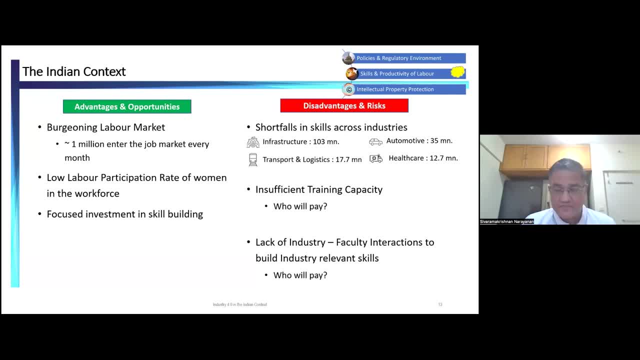 or industry academia interactions? who will pay? Right, If we have to do internships for students, if we have to do projects, you know, industry projects by the academia? who will sponsor whether the industry will sponsor exploratory research into some of these areas which are unknown today? right, How do I know? 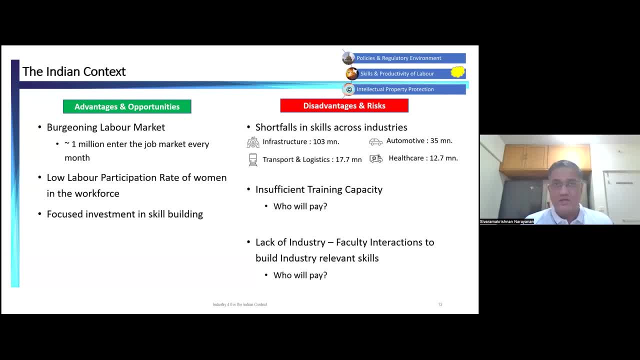 what to do with a brain-computer interface, right, But if there is a practical application of that, I'm sure a lot of industry people would be immediately interested. But somebody has to pay right? 3D printing: when it took shape, nobody would be bothered to look at it, But today, 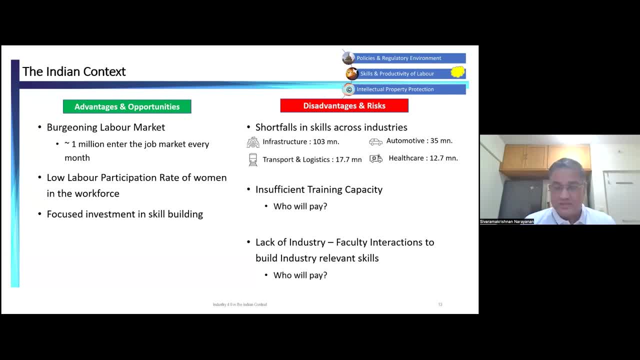 everybody wants to jump in. So I think it's a good question. And I think it's a good question. So if there is somebody who can foot the bill for some of these exploratory discussions and research, there would be a lot more progress. that is possible. So the question that we need: 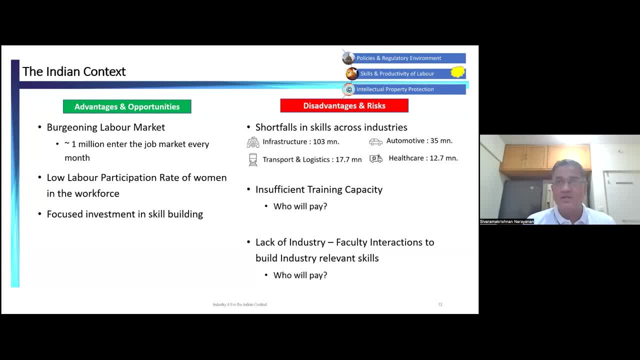 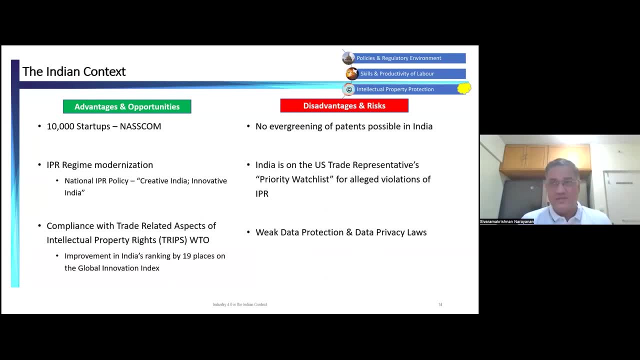 to answer pretty urgently is: who will pay right? Because it needs to make sense at the end of the day. That is the important thing. The Indian context, right. So one of the questions that is being addressed- the academia and industry interactions- is the 10,000 startups of NASCAR. 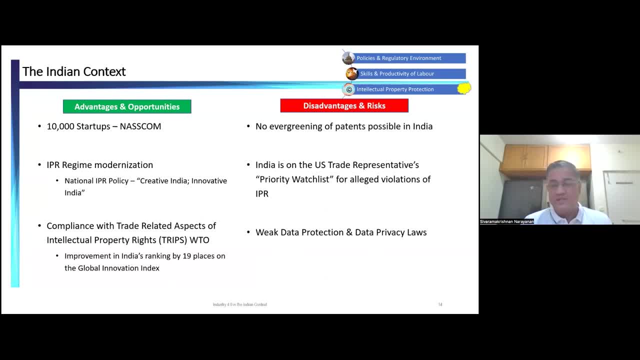 This is a pretty famous program. They want to have 10,000 startups under the ages under the ambit of NASCAR And they are growing a lot of them And a lot of them are doing phenomenal work, eye-poppingly surprising work, right In a very, very positive sense, And 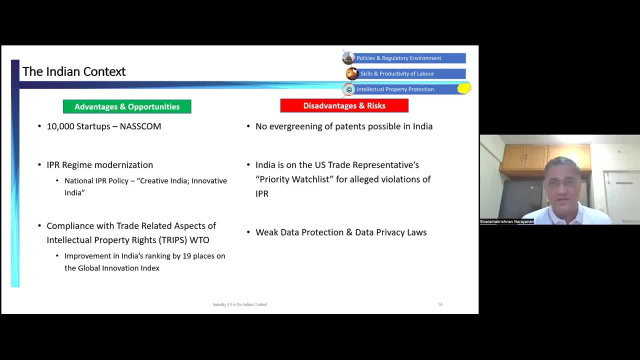 it's a huge matter of pride as an Indian, as a person of this country, for us to see the kind of work that we can do if we just put our mind and will to it. IPR regime is being modernized Again. the criticism is that it's not being modernized. 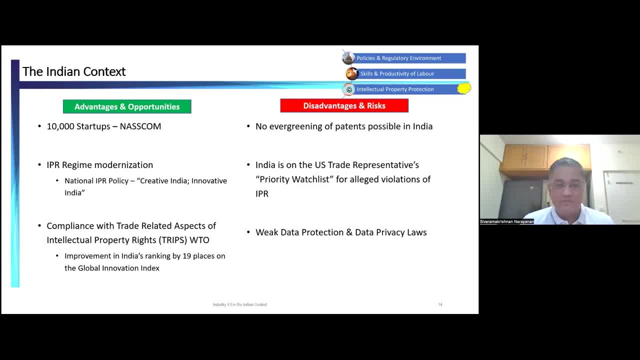 Fast enough. We are in compliance with TRIPS of WTO. but again, but we need to do more right. So the evergreening of patents is not possible. So there is a lot of resistance from Western countries who have patents, who are sitting on patents, to share that with our country. 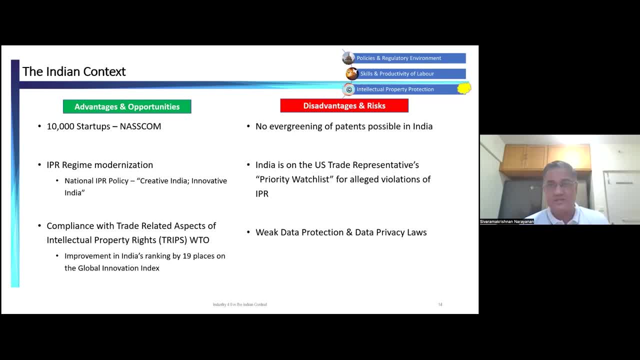 Of course, we have our own point of view on that which says, as a developing country, some of these patents ought to be shared so that the larger humanity will benefit. Alas, there is, you know, not many guys still around, like the inventor of the polio vaccine. 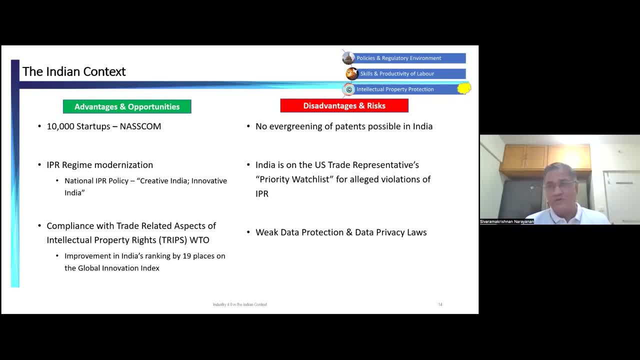 who gave it away for free to the world, And today we have no polio in the world. right, There aren't so many people left. Everybody wants to have their research payback on an ROI- But yeah, I am a little bit of a romantic in these matters- that knowledge are to be shared. 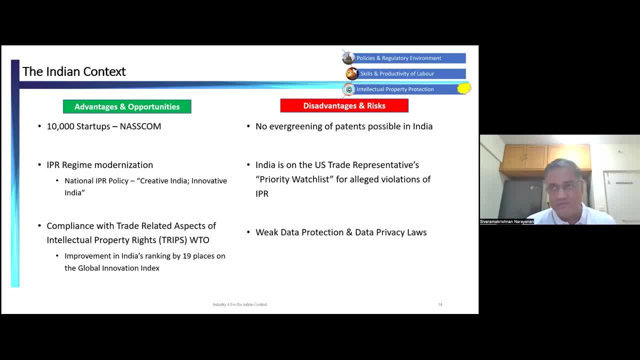 And the more we are able to share the knowledge, the better we all will be collectively Right, India is on the US trade representative's priority watch list for IPR. How we get out of that, I am not the expert, I wouldn't know. Weak data protection and data privacy laws. 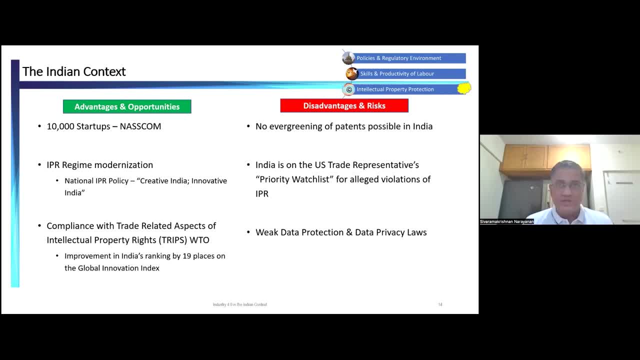 We are in the process of addressing this and hopefully our data privacy bill, which is currently going through various committees in the parliament, will come out in a way that meets some of the expectations of the rest of the world. So at this point in time, 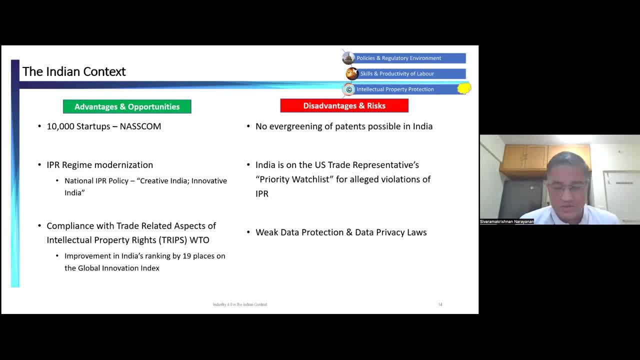 I will pause. I will request Professor Muriel to check in and provide his perspective, because till this section or till this slide of the presentation, I've been talking very high level And at this point in time there is a perspective that I think will be valuable. 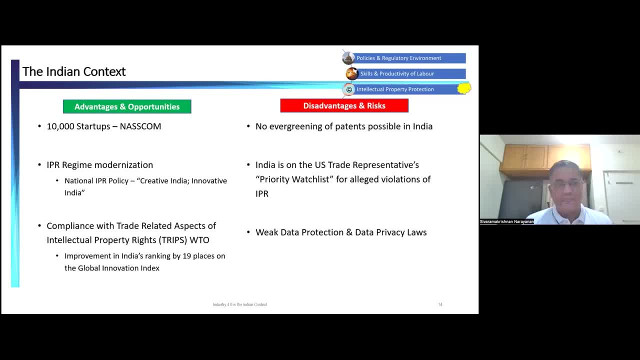 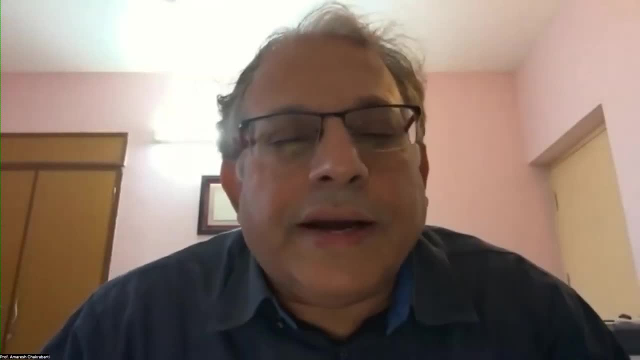 for us to hear from Professor. Professor, over to you, I'll put myself on mute, Okay, Thank you. Thank you, Mr Sivaramakrishnan Narayan, for your views. Wonderful, There are two, I think I have. 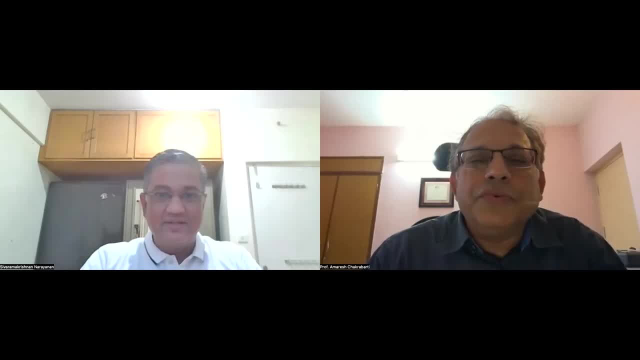 been already warned by Dr Sushila that we are running behind time and therefore we shouldn't take too long on this, So let me just say a couple of points and then maybe take one or two questions that are already enlisted in the Q&A, so that we can also involve our participants in the discussion. 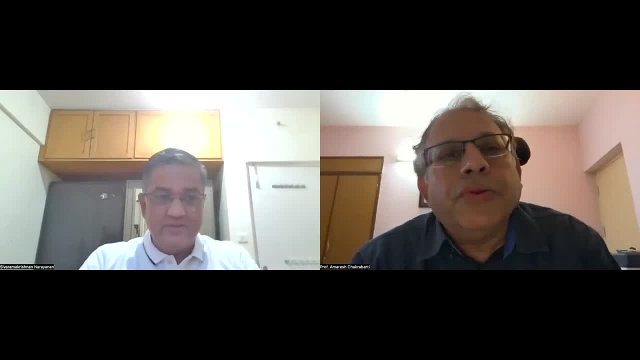 I would say that you know, one way to look at Industry 4.0 is to say that from Industry 3.0,, if you like, it sort of translates from automation or individual automation to institutional or organizational autonomy. That's the distinctive feature of Industry 4.0. Not that you have achieved it, but that's the ideal. 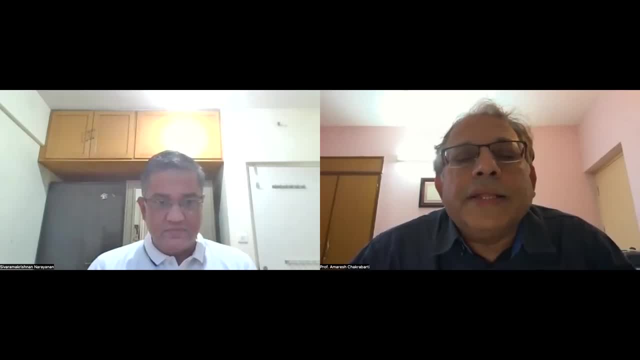 You're watching. how do you have a connected system where there can be connected intelligence, with which more can be achieved with what is available? So there is a question that is there. I will just start with that and I'll just read it out, because it's framed rather well by Mr Rahulam. 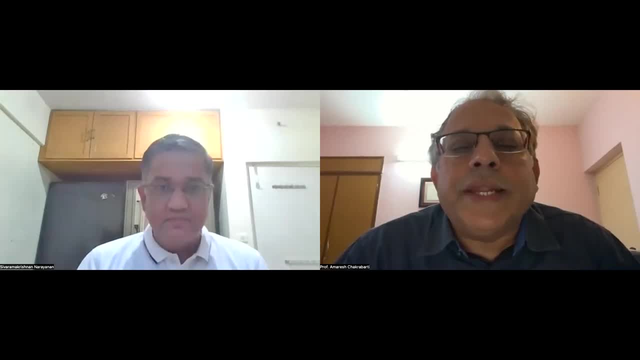 What are some first steps that a traditional company can take to embark on an Industry 4.0 variety in their jobs, on an industry 4.0 journey, without getting overwhelmed by the plethora of technologies? So please go ahead. So this is like they say. 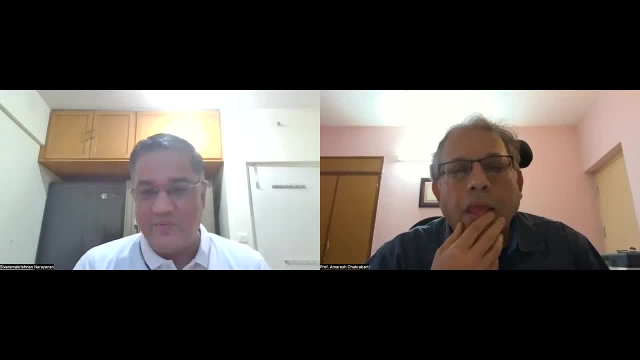 like eating an elephant. right, It's one small piece at a time. So the first thing that I would look at is: what is the data that is available to the company right? Where are there any tasks, any daily transactions that need to be automated? 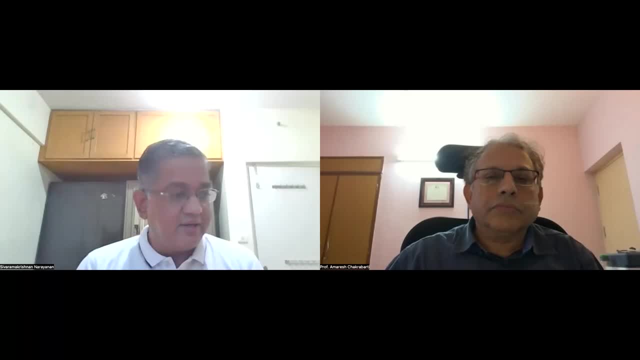 that can be connected in a different way. So, to give you an example, I was visiting this company yesterday, which is in the aerospace business, And in the aerospace business, because of safety reasons and regulatory reasons, they will have to maintain an invoice for every part. 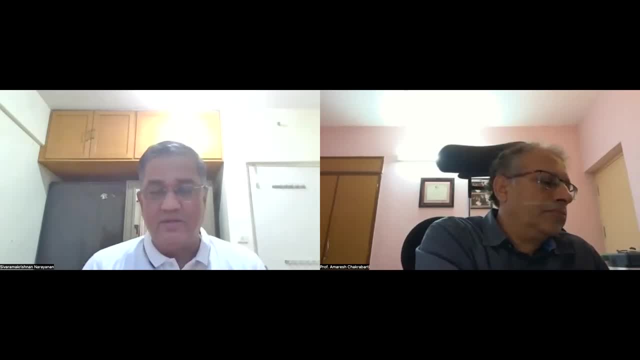 Every single part they ship out of their company goes on a separate invoice. Now this company makes something of the equivalent of 18,000 different parts And obviously multiple copies of the same part has to be invoiced out. So they run in the region. 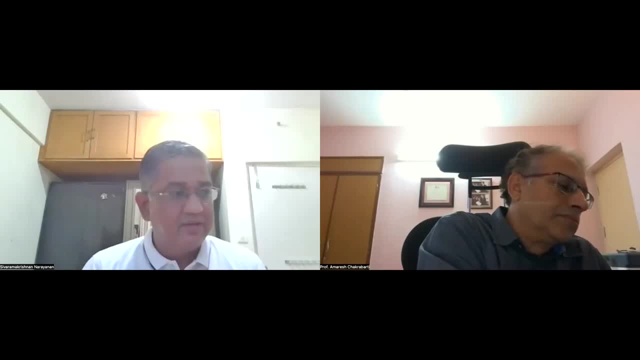 of about 200,000 to 300,000 invoices a year. Now, if this were to be entered by a human being or a team of human beings every day, you would need an army of human beings doing this entry. This company has embarked upon a journey. 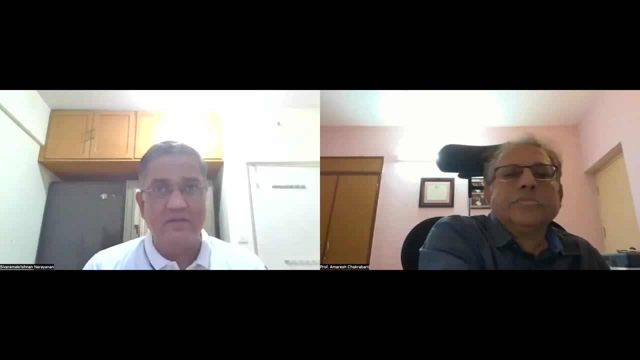 called robotic process automation, where a robot, a software robot, is entering the invoices into their ERP transaction system automatically. So they just feed the data into a standard format And the robot actually enters the data. and they manage this whole operation with two people. 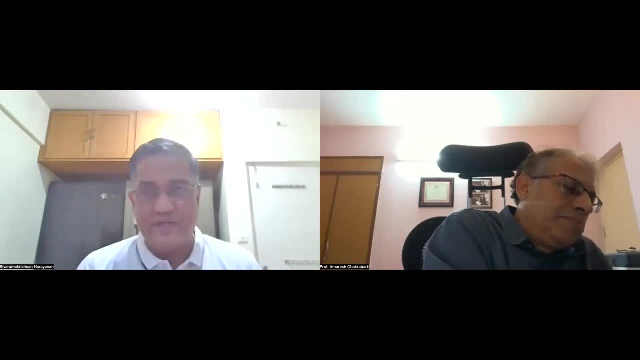 Now, at the face of it, you have actually lost the employment of 10 people that could otherwise potentially be doing invoice entry. But the question is: do you really want those people to do invoice entry or do you want those 10 people that you could otherwise deploy? 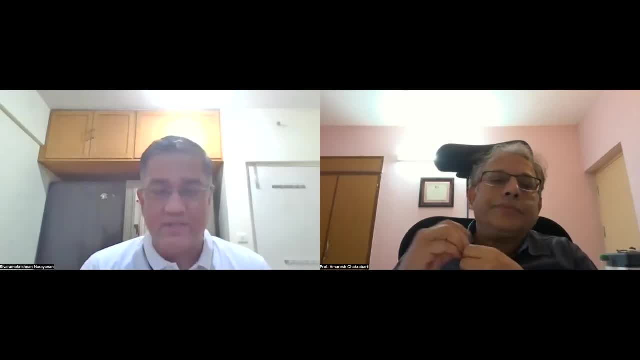 in another, more value-added job, And the answer is obviously the second right. You would want them to do a more value-added work. So it's a small area where they have started. Now they have understood. okay, this is a good step forward. 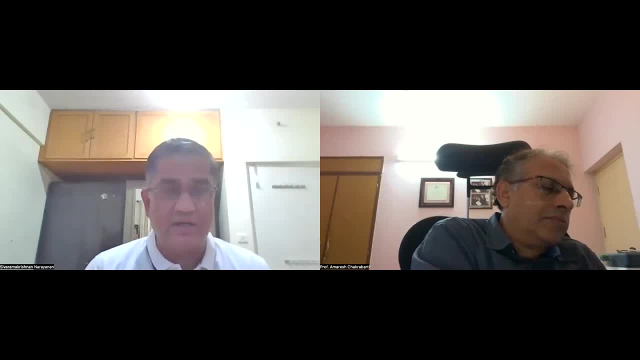 Now, can I do this robotic process whatever in other areas of my shop? Can I do this in my warehouse? Can I do this in some other procurement-related activities That I have today where I have a huge amount of data or data entry right? 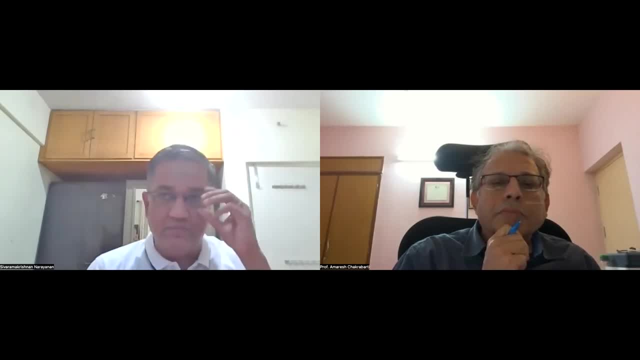 So it goes like this: It's an organic journey. It's not something that you should impose from top. Of course there is a little bit of direction and vision required for the company, But areas where you can actually generate, obtain and gain in efficiency. 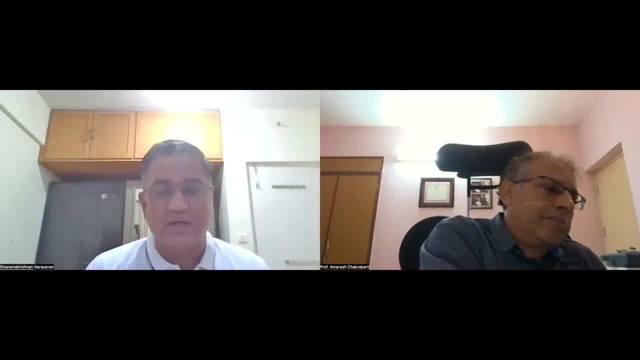 and some of those will be pretty obvious when you start- would be the way to go. That's normally how companies start these journeys. Look at one aspect And see whether you can fix that, And then you're off. You don't need to think about it too much. 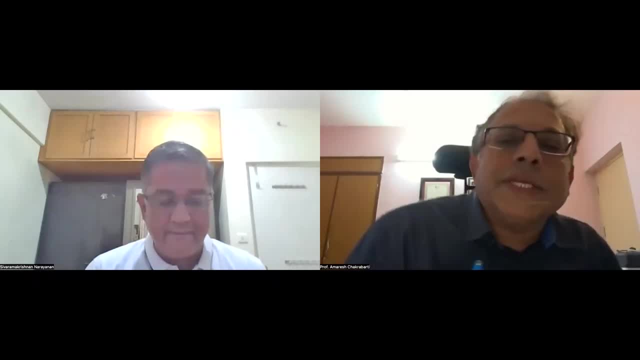 Okay, thank you. Maybe we'll just take one more question and then move back to your presentation again And I will perhaps ask the following: that there is a in a sense- and I'm just expanding someone's question here a little bit- 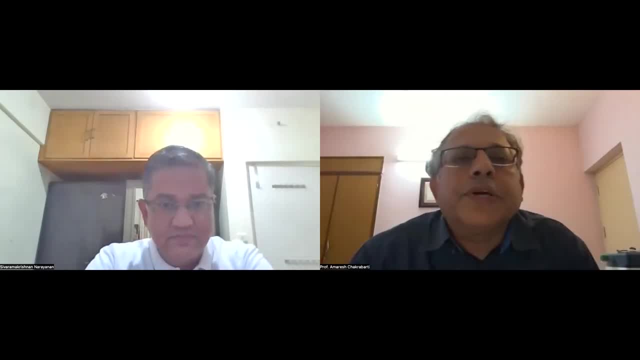 That there is a. if industry 4.0 gets implemented, as the it's being promulgated, right, Then you are going to have these millions of sensors, IOT devices and so on and so forth that will be deployed in addition to the energy. 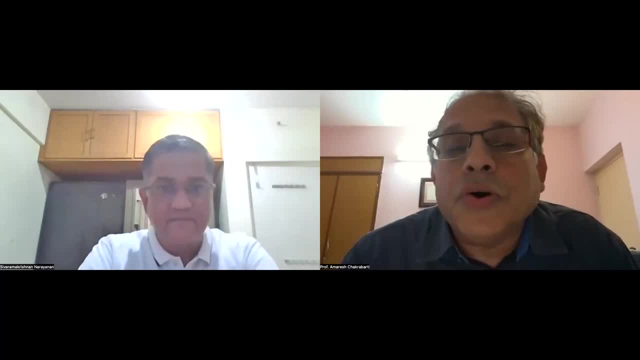 perhaps energy intensive technologies that are already there. So I have seen and noticed that you have said green technology or green energy, But that alone is perhaps not enough. I mean. so It's surely going to be far more capital intensive than it is right now. 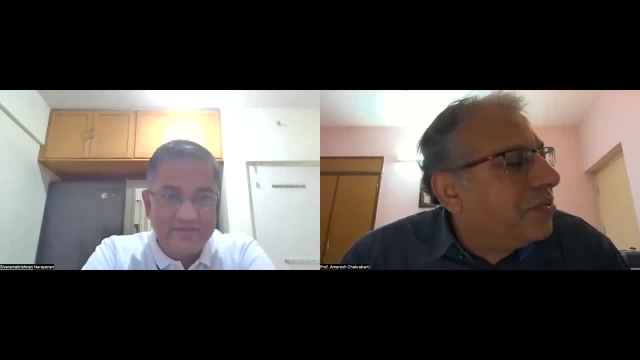 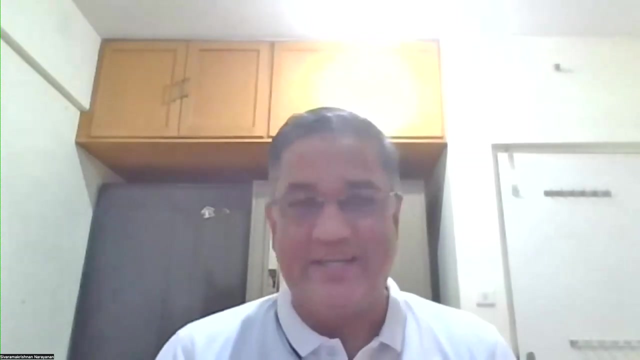 So how does it help us to remain or become more sustainable while being in industry 4.0, sorry, So brilliant question, professor. thank you. So that is one of the dilemmas that we have today. right, So we don't see the impact of the large data centers? 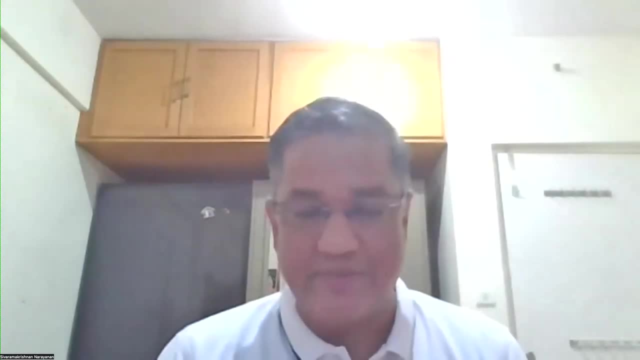 that we somehow implicitly consume. I mean, all of us are on Facebook or Google or Twitter or any of these, or Amazon in various forms, and we don't really see the impact of these giant data centers that are running in various places, that are today considered one of the largest generators. 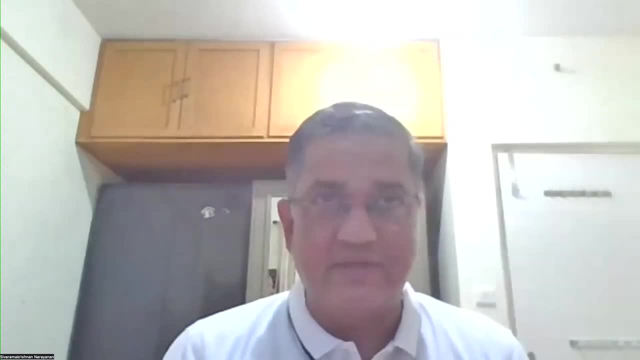 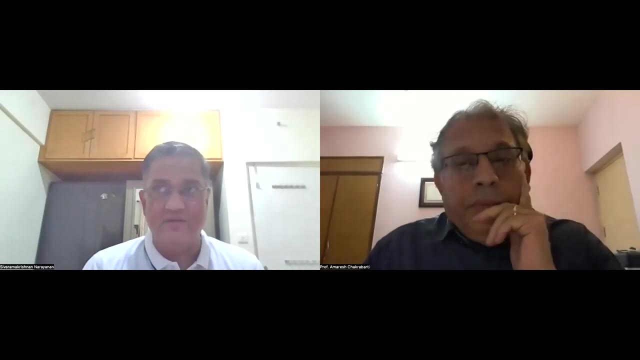 of greenhouse gases in the world, So I don't have an answer to you. It is a. it is a very valid question. when we have sensors and when we have instruments that are generating millions of data points per single piece manufactured, We are going to have a huge data center problem. 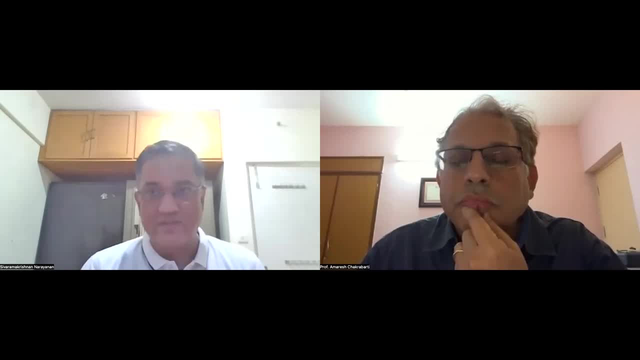 And I don't know what we have to do. It is definitely not sustainable the way we are managing our data centers today, And that's something to think about. But no, I don't have an answer for this. You're on mute, professor. 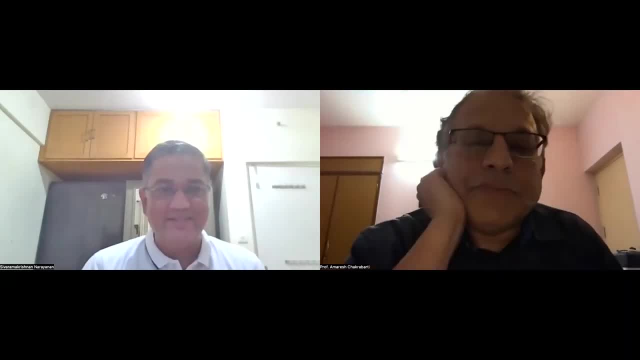 Yeah, sorry, I was just saying that this is the last question I'm going to ask before I give the mantle back to you for the rest of the presentation, And that's the following, because this is an oft-asked question, right? 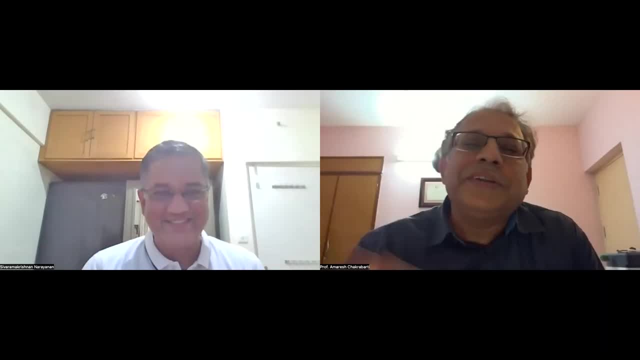 I'm not necessarily expecting an answer, but I would still like you to deliver it on it, And that is: what does industry 4.0 mean in terms of employment? Oh, I have that as a question as well, So I will answer that in a little bit. 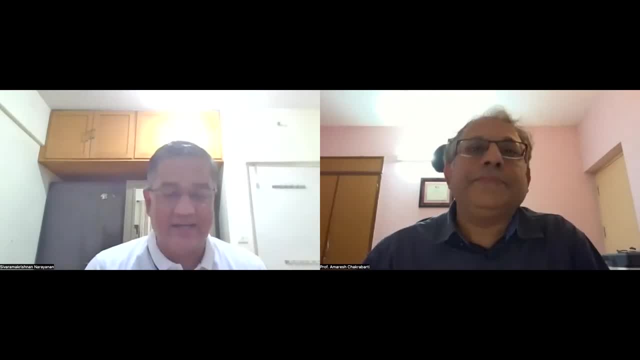 if I may park this for the moment, because it is one of the questions that I have taken up to be addressed as part of the final set of questions. OK, brilliant, So then please defer that And please go back to your presentation. 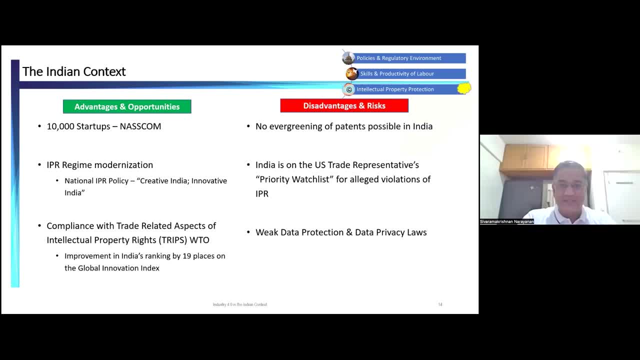 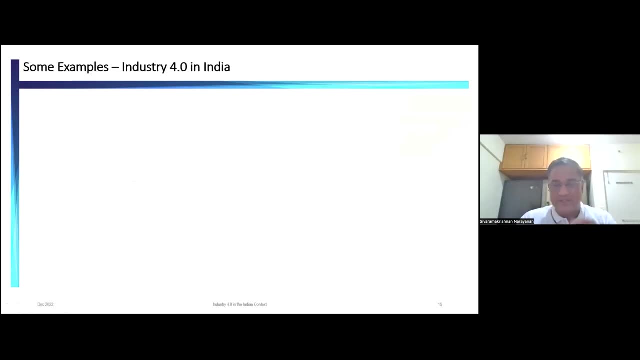 Sure, I'm sharing my screen again if I can just get a confirmation that you all can see my screen, I can see. OK, So let me go down now to the examples of industry 4.0 in India. I'll spend a little bit this part of the presentation. 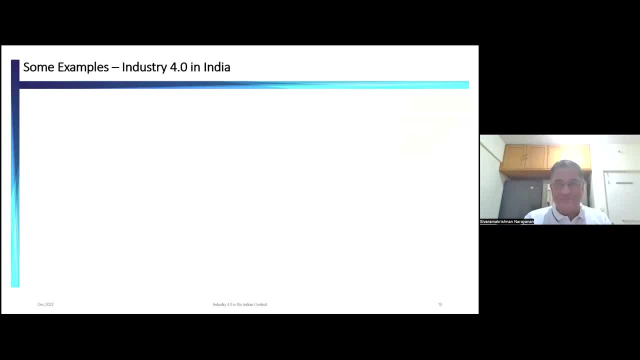 because I can't name the companies. They are all companies here in India that are doing this kind of work, But I'm happy to have a one-on-one conversation with any of you Using nanotechnology for food packaging. I briefly touched upon this a little bit earlier. 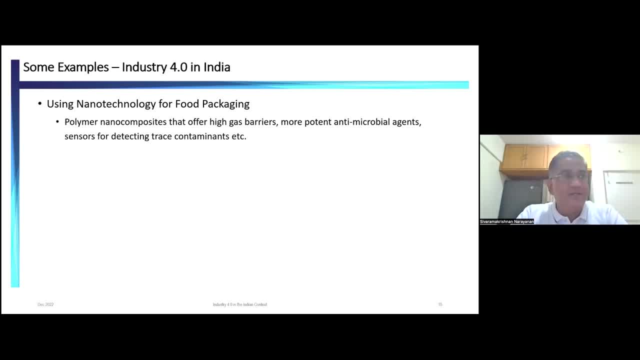 So, if you're manufacturing chips or if you're manufacturing, say, idli batter- and a lot of companies are there in the market today- One of the key things that, or even coffee powder, for example- a lot of companies are. 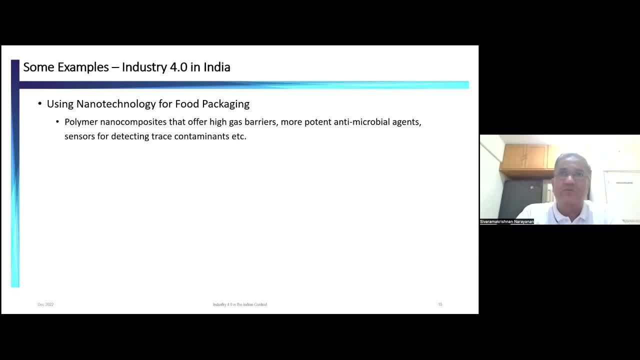 there which are trying to go direct to consumer right, To take Products, agricultural products, from the farm, Process it in some way, Deliver it to the consumer as fresh as possible so she can actually enjoy the benefit of fresh food And keeping it fresh. 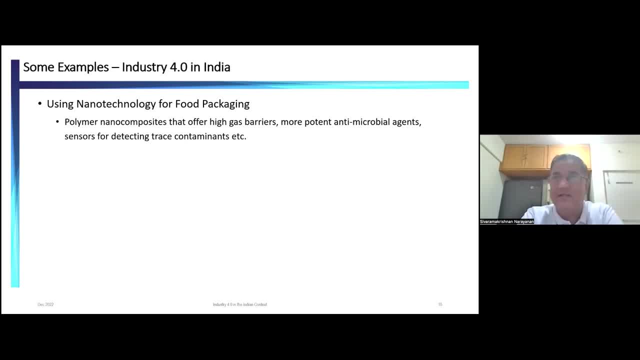 I mean these days I find raw mangoes, which was for me a treat in the summer months, in the month of October and November, During Diwali, I was happily chomping down a raw mango, And that's an incredible agricultural feat. 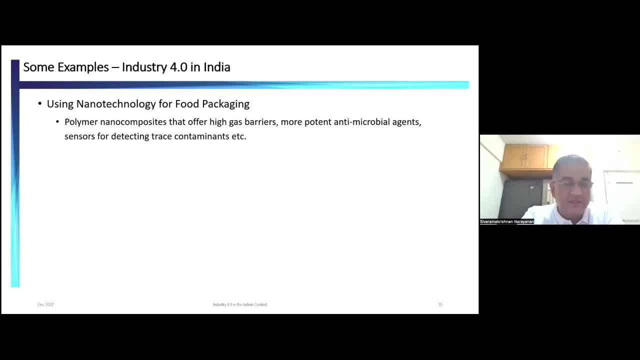 if I may say so, And some of this is part of the green supply chain or the nanotechnology-enabled supply chain that we see in the food processing business, or even deep freeze or frozen supply chains that we see, So this has made food pressure more accessible to consumers. 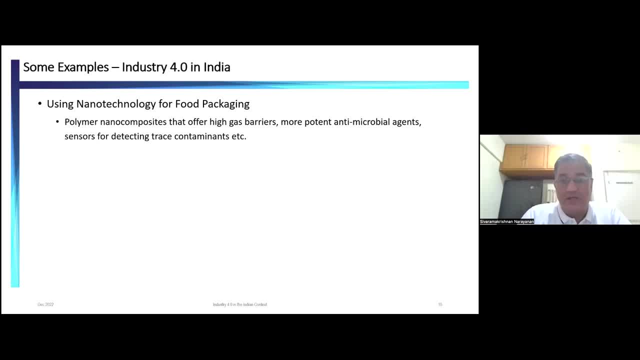 in, even off season, And that's something that people are working on, And this is also, to a certain extent, applicable in the pharmacy and pharmaceutical industry: nanotechnology-based packaging, Using biotechnology and nanotechnology to manufacture artificial skin. I think all of us can immediately understand. 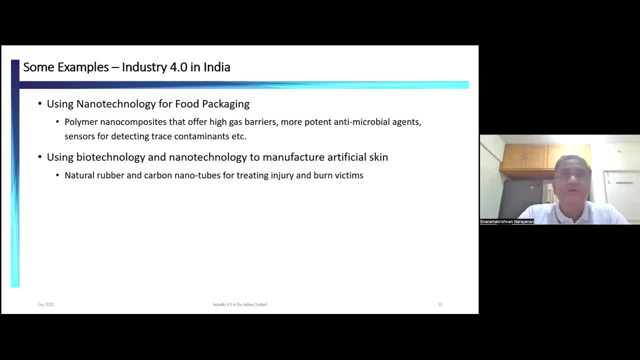 the applications of such a manufactured product. Natural skin is a difficult thing to source. Skin grafting is something that is required, unfortunately, in many, many hospitals for different reasons, But it is possible to treat this using artificial skin. What is even more incredible is 3D technology. 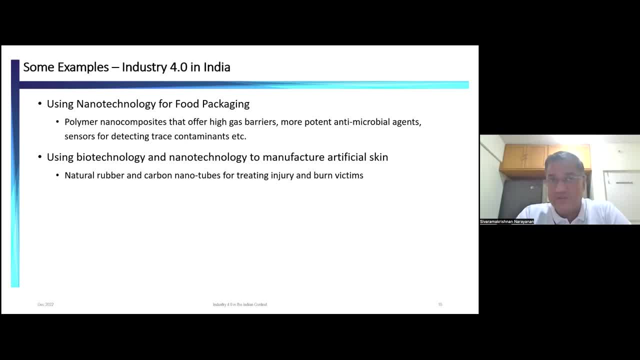 3D printing technology has gotten into the act as well, So it's possible for us to print skin. There are companies in Bangalore that can print liver tissue, And you heard me right. There are people that can print liver tissue And the company that I have had the privilege. 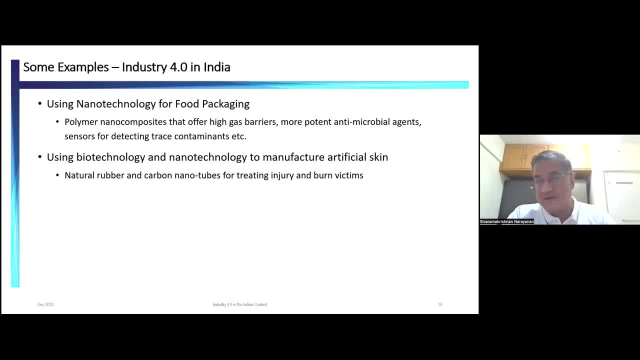 of associating myself is in the business of printing corneal tissue, eye tissue, And there is a condition that causes incurable blindness And there are about 600,000 people in India that go blind because of this condition on every year. 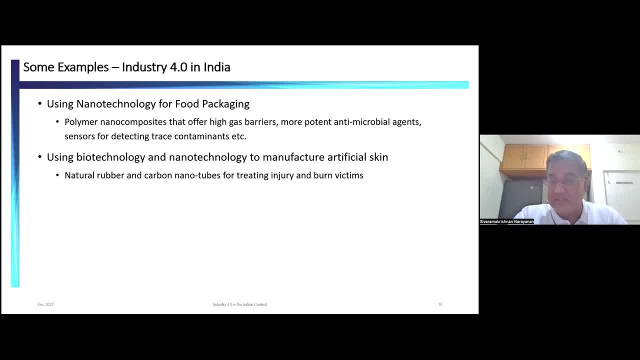 600,000 people every year go blind because of this eye condition, which is peculiar to the South Asian region, And this company is in the business of actually working on a path-breaking technology that prints eye tissue that can cure blindness. Imagine the societal impact. 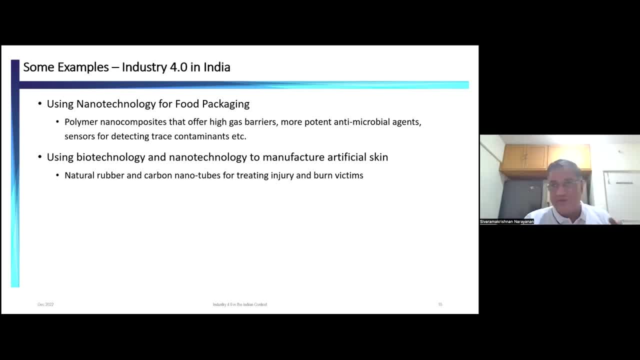 of this, right. So this is you know somewhere. it goes beyond just manufacturing. It becomes inspiration, right? A lot of this is happening right here, And some of it is in Bangalore, using blockchain technologies to prevent counterfeiting. 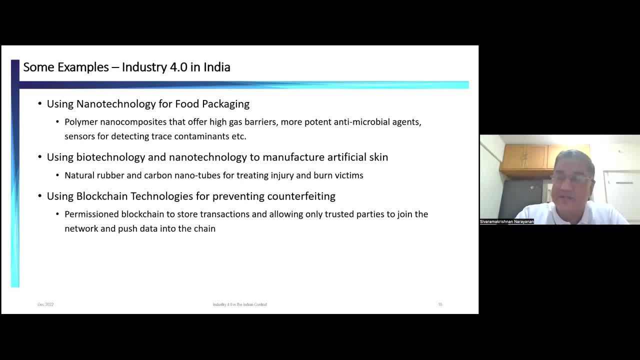 Now, this is an old, you know, in relative terms, an old problem. You know fakes in pharmaceutical business, right, Fake tablets, the unfortunate incident of young children dying in Ghana, I believe consuming substandard cough syrup and also maybe spurious medicines. 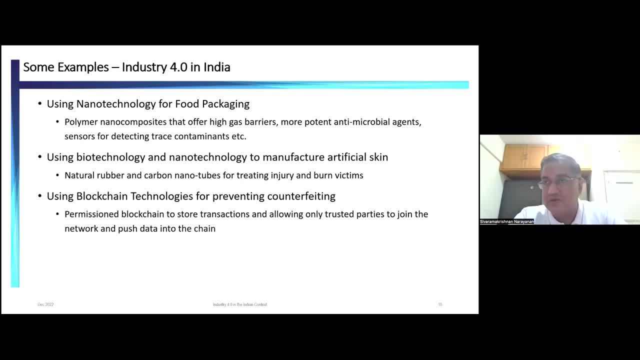 or spurious spares in, say, machinery or automotive parts, spurious parts which cause accidents and death. So can we use blockchain technologies to prevent counterfeiting? Can we use a permission blockchain with security in place so that we can only allow trusted parties to join? 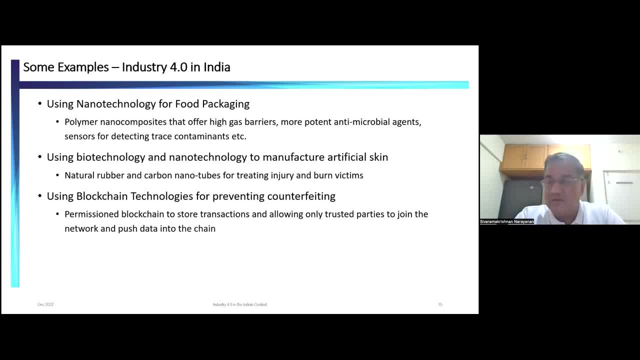 So this is a wonderful application of blockchain which doesn't cause monetary loss, Which prevents actually the risk of death because of spurious parts or spurious medicines, Saves lives, saves costs, because otherwise manufacturers have to spend lots of money countering counterfeits in the, in the shop, in the market. 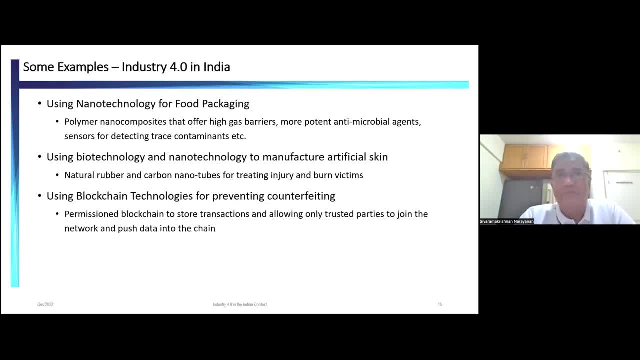 And this is happening right here. Okay, some of the biggest pharmaceutical companies in India, in the West, in the Western part of India, for example, have been experimenting with this for at least at least a decade till now. So, like I was mentioning a small part, which is you know, 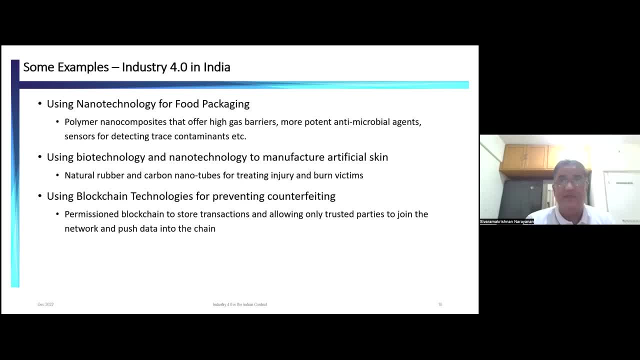 something that offers an advantage to you as a company. if you start an experiment there, and if that experiment is successful, then you can actually start moving it into other areas of your business, And this is one of the best examples I can give you. 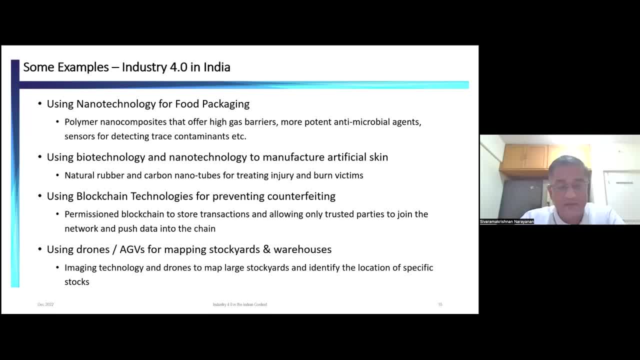 of using blockchain for counterfeit management or counterfeit preventing, counterfeit, Using drones, automated guided vehicles- right. So very recently, we may have read in the news about Reliance acquiring a company which is in the business of automated- sorry, autonomous guided vehicles in a warehouse. right. 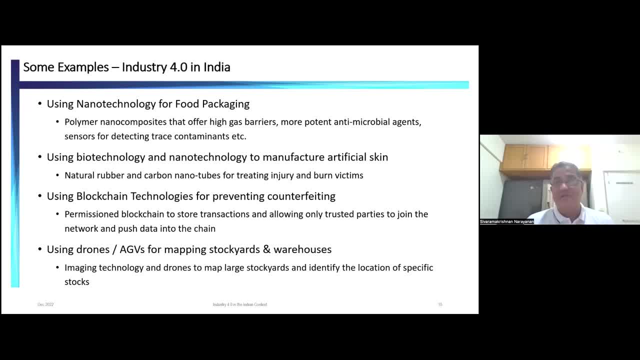 And that's their business. This is an Indian startup that is making this happen. There are large warehouses with with, say, for example, Amazon, or the Indian company Udaan, or Urban company, Urban Ladder, which is the furniture company of Pepperfry. 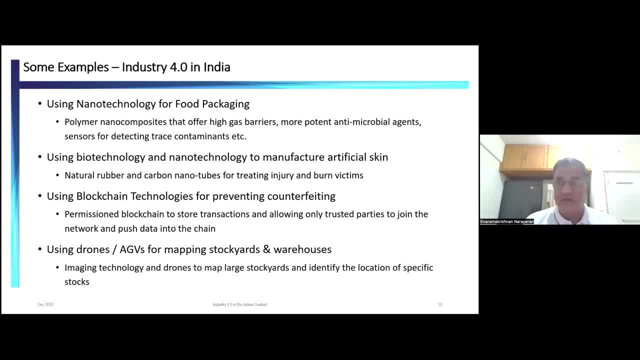 huge warehouses where you do not know where your product is. It's stocked in the warehouse. It's possible for you to deploy some of these things I have seen. I have worked in steel factories for a bit And one of the biggest challenges in steel 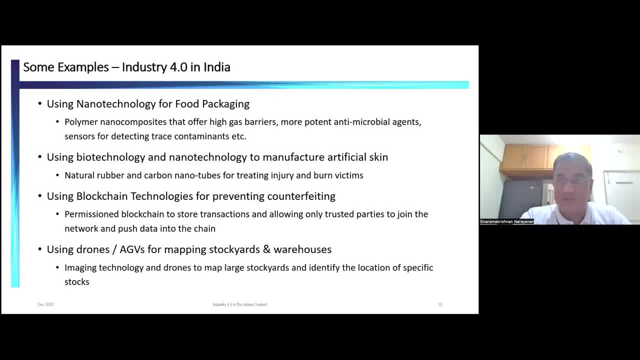 is to identify the specific piece of steel that you need to ship to your customer, And having a drone in a yard which could be a kilometer long can be a massive advantage about selecting and loading that particular steel coil or steel coil. 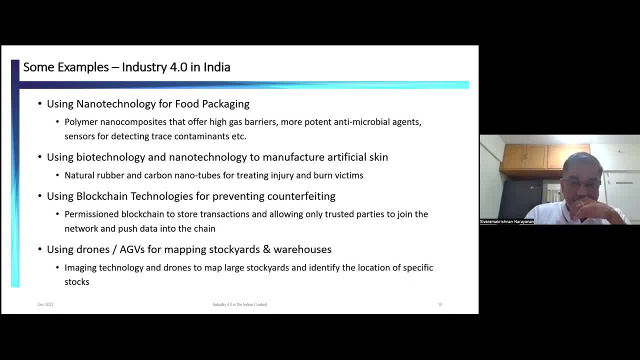 or steel slab onto a, onto a rail wagon. Okay, Also cars. I mean, we've all seen those of you who've seen automobile showrooms or automobile yards. again, it runs into a couple of kilometers and there are literally thousands of cars of various colors. 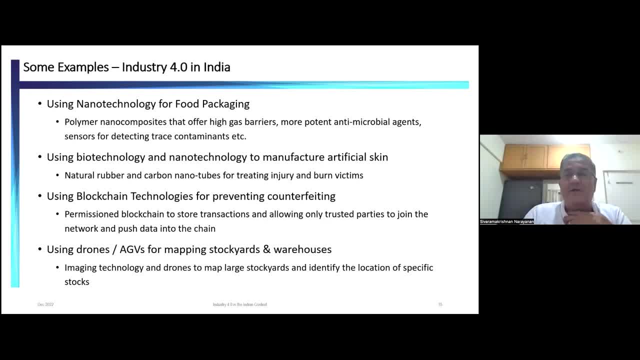 that are parked in these yards prior to shipment. Identifying those cars where they are and then picking it up and putting it on a truck for it to be shipped out is a big, big challenge, right, And there are people trying various things. 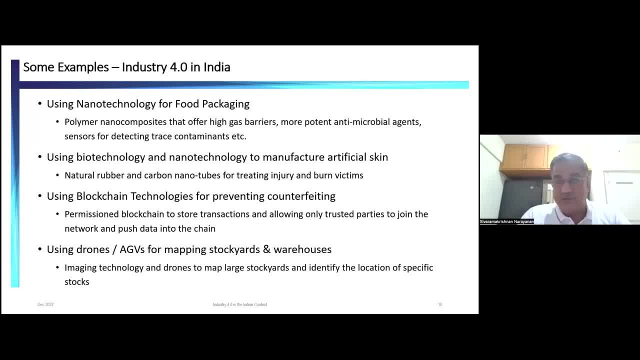 including 5G technologies And drone, is something that I have seen personally happen. Right, And this is a very simple application. Today, what happens is a worker goes every day- morning, afternoon, evening, walks- through the yard. you know, make sure that the car is in the place. 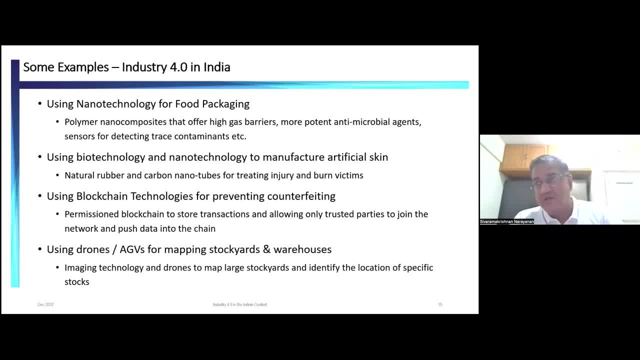 where it was supposed to be marked right in the system. If there is any change, then he makes a note on a paper. then it goes back into the system. They actually update it. A drone, on the other hand, scans the RFID. 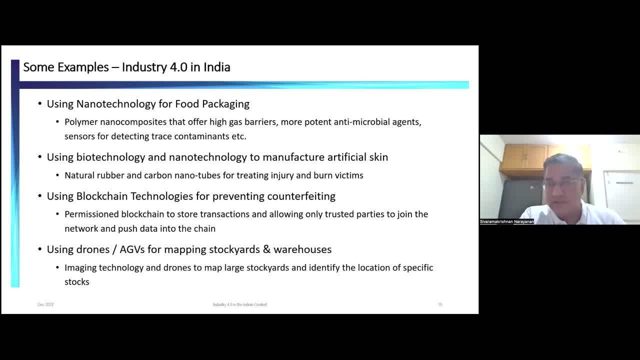 that is pasted on the car Directly updates the system. There is no worker. What the worker does in six hours, the drone does in 15 minutes And there couldn't be a more- you know dramatic productivity gain that I can say in this. 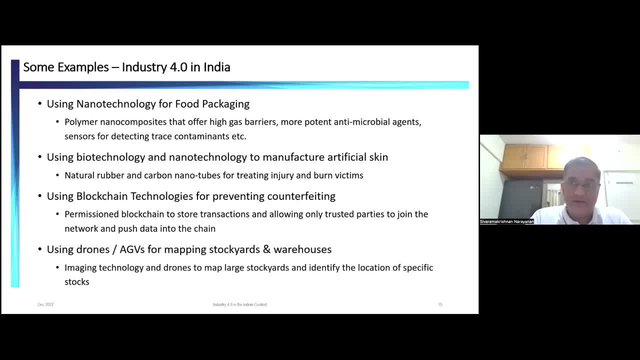 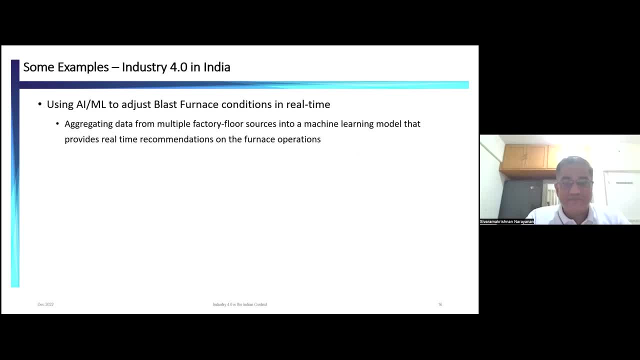 And this could be a car. this could be a steel coil or a steel plate or any other large equipment that is in a big yard. Let me run for several kilometers. Blast furnace right. One of the biggest challenges of energy consumption in the steel industry is how and where. 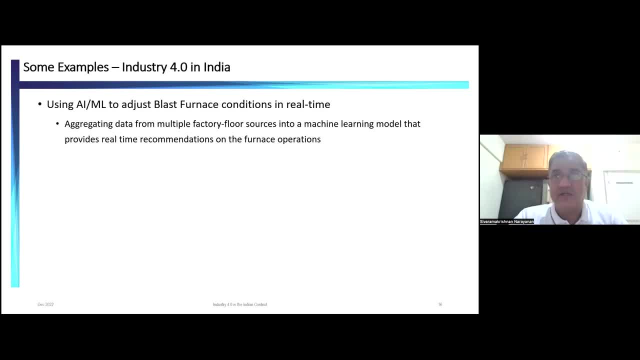 how do you position what is called the oxygen lance right? So steelmaking involves a lot of injection of oxygen into the process. How do you position the oxygen lance? When do you inject the oxygen? At what angle do you inject it Depends on a lot of furnace conditions that are not known. 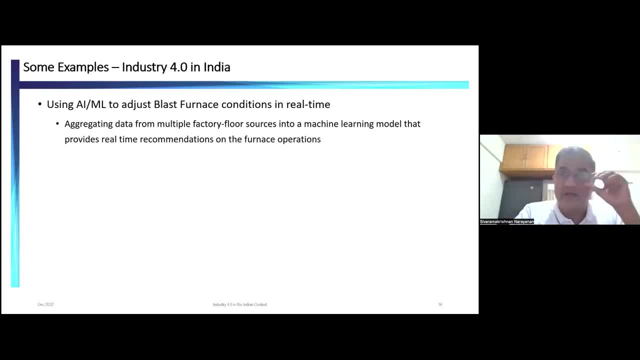 You know that happens dynamically And you melt typically anywhere between 150 tons to 200 tons of steel in one batch, And it's a very dangerous environment, right? So the person that controls the oxygen lance- right, is the person that controls the oxygen lance. 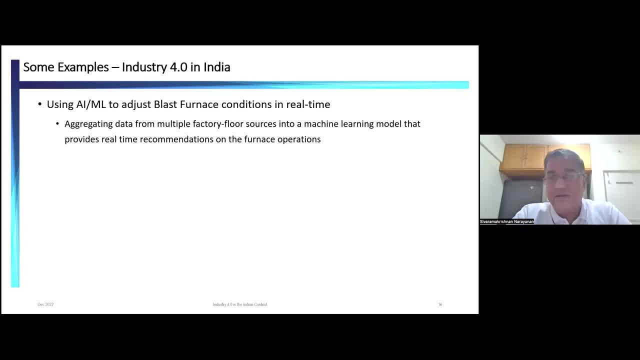 Looks like somebody from outer space. right He's wearing. typically it's a male. it's a very exhausting job And he is standing there in 70 degree heat trying to manage an oxygen lance that has to be pushed into a live furnace. 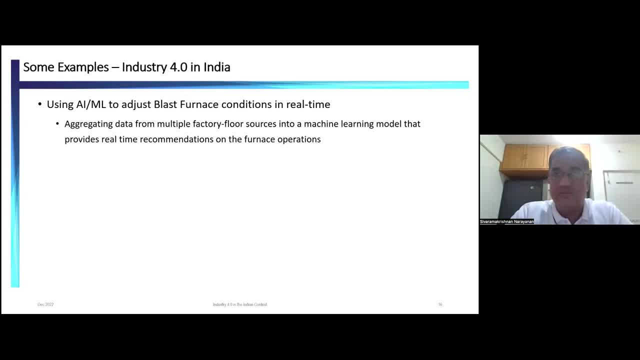 But if you have a machine learning model, then the oxygen lance can be actually positioned by a robot that can do it far more efficiently and far more accurately than a human being can, And this is something that is already happening in some of the Indian steel factories. 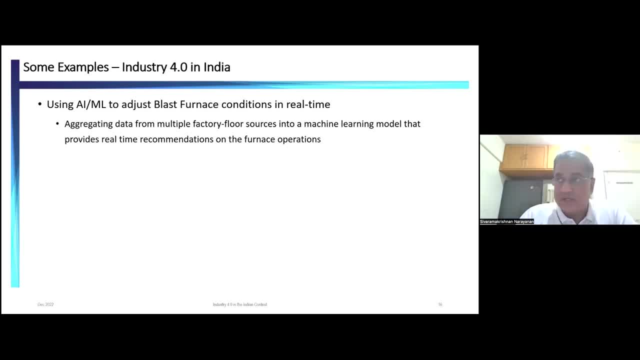 that I have visited right. So this is another very good example of how you can make a small beginning, because this is a typical case where the work environment is dangerous and you know. you need a lot of accuracy as well, And it's hard for a human being to maintain accuracy. 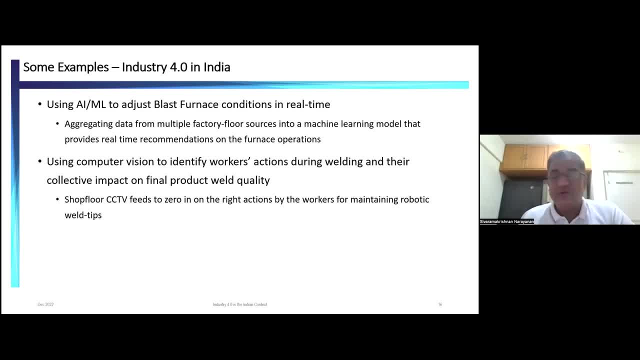 in a highly toxic and dangerous environment, Using computer vision to identify workers' action on the shop floor right. We've all seen CCTV right And one of the auto companies that I have worked for in the past has you know: typically automobile involves a lot of welding. 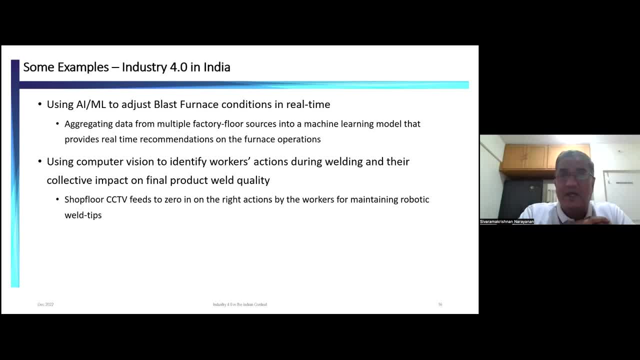 on the body of the machine, on the body of the auto, And weld tips. the way the welding technology is, weld tips get deposited with carbon And one of the problems is if you have a weld tip which has been deposited with carbon. 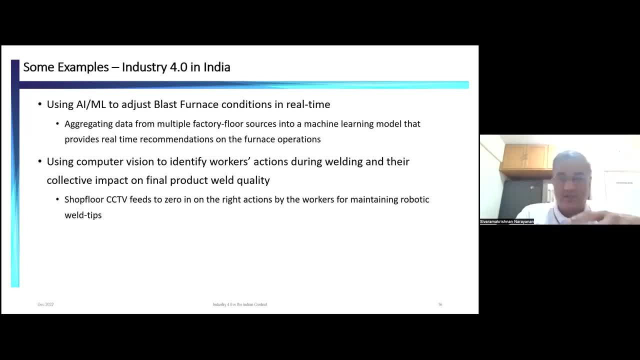 the weld quality kind of goes down. If the weld quality is down, then it could either be a safety issue for you or it could be just an irritation, because you will hear rattling. Two metal pieces will keep bumping into each other. 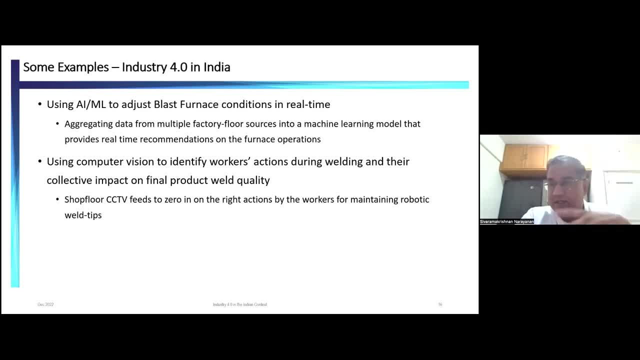 if they are not welded tightly together right, So it could be an irritation or it could be a safety issue. if you have an accident, the whole car falls apart because of poor quality welds. So you have to dress the weld, you have to make sure that the carbon is removed. 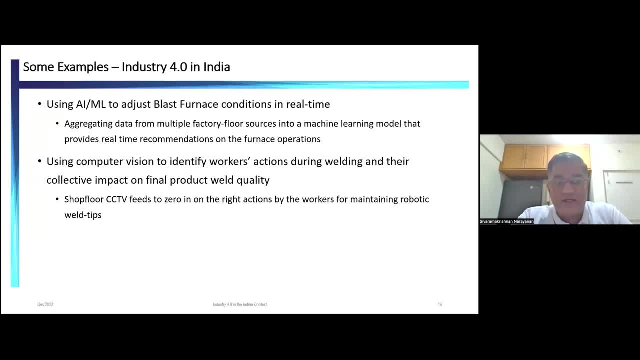 and the weld quality is maintained, And what we were doing is using CCTV cameras that were in the shop to understand from the actions of the worker whether they are actually maintaining those weld tips properly, right? So there are various actions that the welder does. 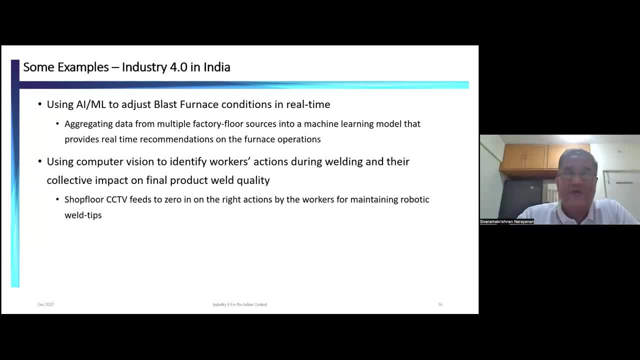 on the shop floor. So we actually trained a model, a machine learning model that helps understand whether the welder, the worker, is dressing the weld tip or not with a certain level of accuracy. right. So these actions are from images. 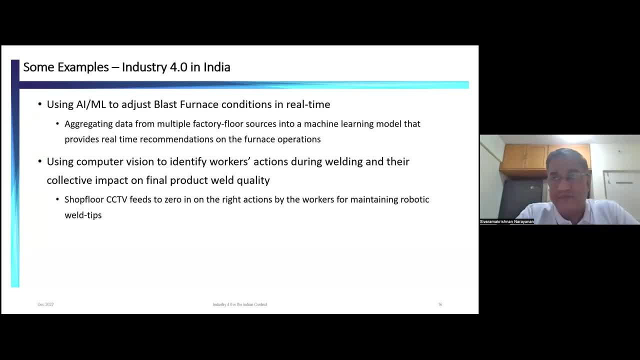 So we converted the images into numbers and classified the actions. a whole bunch of things that we did, which I'm happy to talk about in an offline conversation. Digital twins for complex systems, like I was mentioning a little while earlier, using big data. 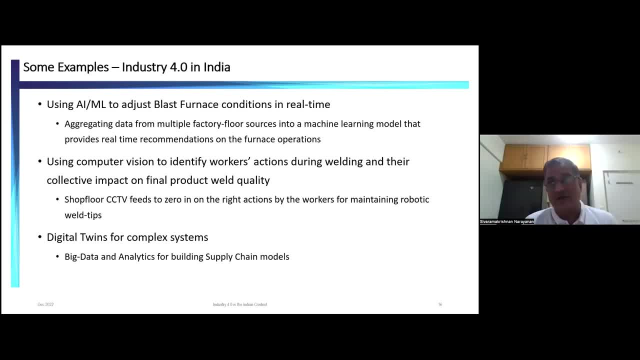 using data that is coming in on the fly and using analytics to build complex things like supply chain models. in an Indian context, where there are multiple handovers, multiple stakeholders, multiple methods of data exchange, it is possible for us to build this. 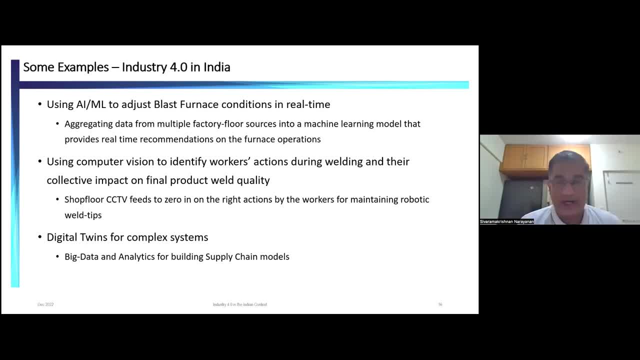 Big companies like Google are actually building digital twin platforms, right? So if you want to actually model your manufacturing or your procurement or your entire supply chain, Google has an offering for you. It's incredible because some of these things 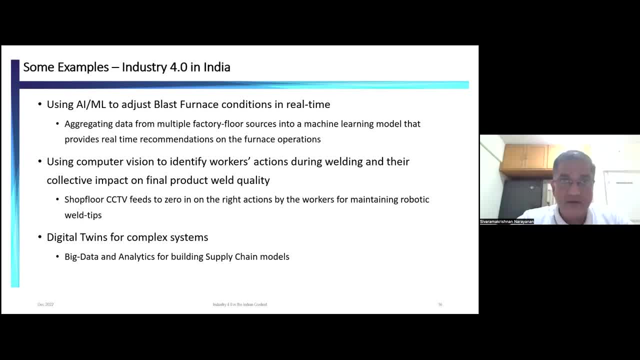 you wouldn't even expect somebody we know more for their mail and their drive, Google Drive and Google Mail- to be interested in a digital supply chain solution. but you haven't. Google has an interest and they have actually built a product that will help you do a supply chain twin. 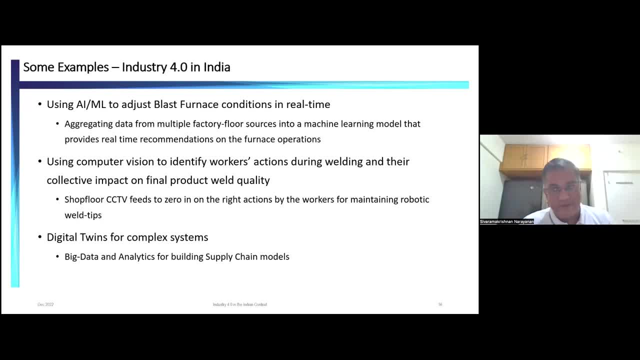 So some of these are examples where I have worked myself. Some of them are examples where I've had the privilege to talk to the CEOs or the founders of these startups. Some of them are just what I have read in the internet and, because of my curiosity, 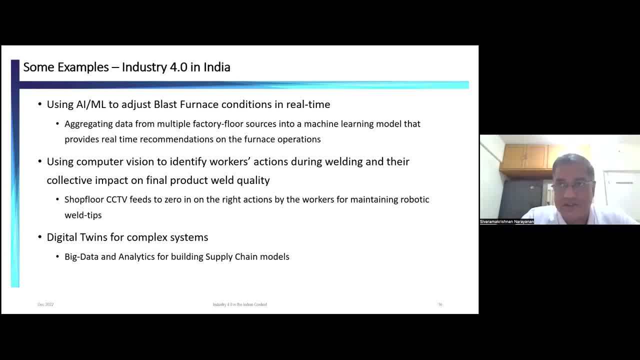 done a little bit more digging right. I'll not name which is which, for obvious reasons. these are all client confidential information, but I'm happy to have a conversation on a one-on-one basis, provide a little more detail on any of these various examples. 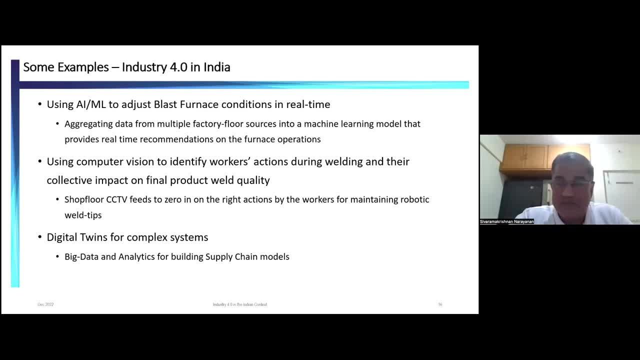 that I have spoken about, So you can imagine the scope and the scale of work from what I have done, And there are other examples that I can just talk about. For example, enforcing contracts right, One of the big challenges in whether it is capital procurement. 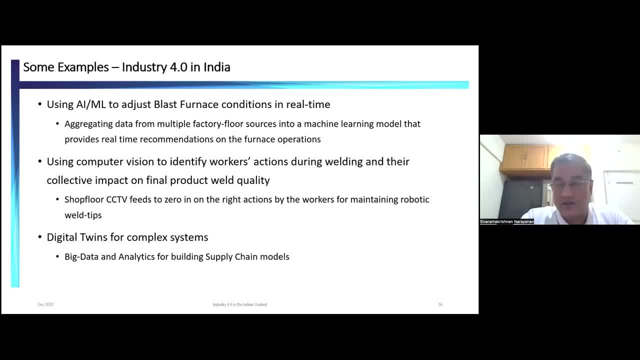 or whether it is repetitive procurement, is how do I enforce the contractual terms on my vendors? And today there are machine learning solutions available which will highlight to you, And there is an entire family of solutions called contract life cycle management, which is today powered by artificial intelligence. 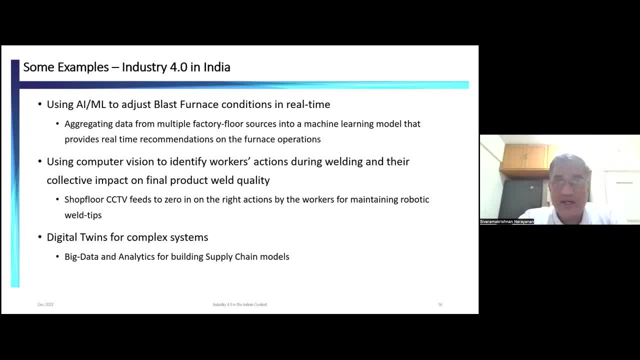 and machine learning And it's extraordinary how the solutions work. Chat GPT, which I was talking about a little earlier, can replace you know, potentially it can replace a million, 3 million, whatever number we have in the BPO industry. 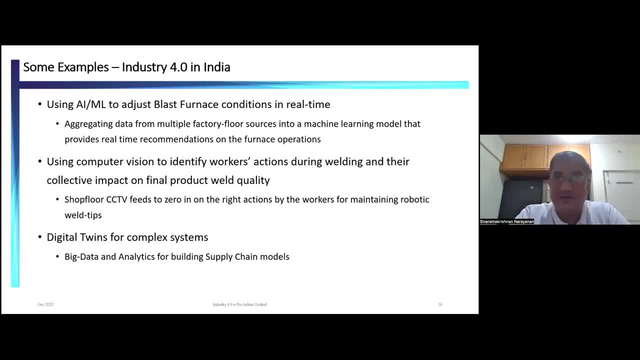 You can just put a chat bot. This can generate human-like responses and nobody would know. And you can even tweak the accent. So you can say: I want this chat bot to sound like an Australian, and it will. You want this chat bot to sound like a Nigerian, it will. 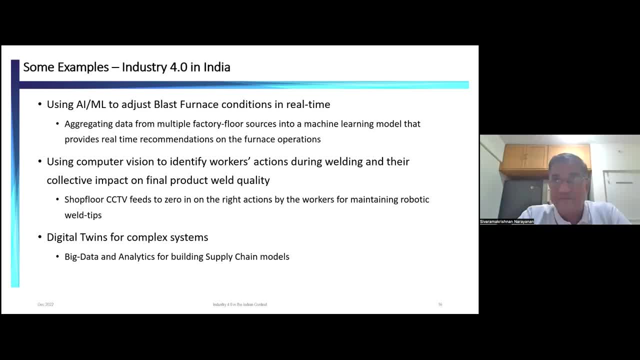 right, And nobody will know anything better. Today, Google assistant can book you a doctor's appointment or a haircut appointment, And the person that is receiving the call from Google assistant will not even know that a robot is calling him or her. So some of these are scary. 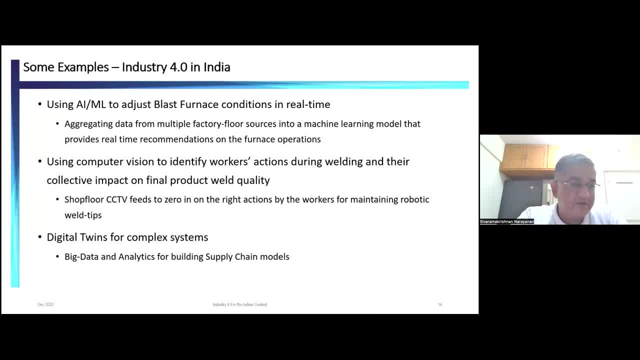 Some of these are incredible. for me, you know, without the burden of a moral compass, If I look at some of these technologies it is incredible, But there is obviously a very strong amount of ethics required to bring these technologies to the industry, to make sure. 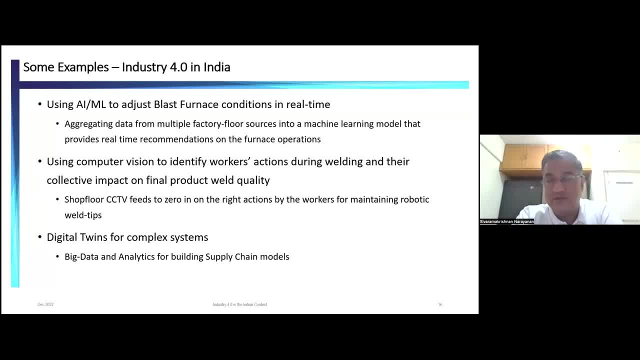 that the boundaries of human privacy or human decency or human intellect are not violated, right It is for us. these are all human creations and we need to respect those boundaries, right? So robots are very great, but a weaponized robot is not so great. 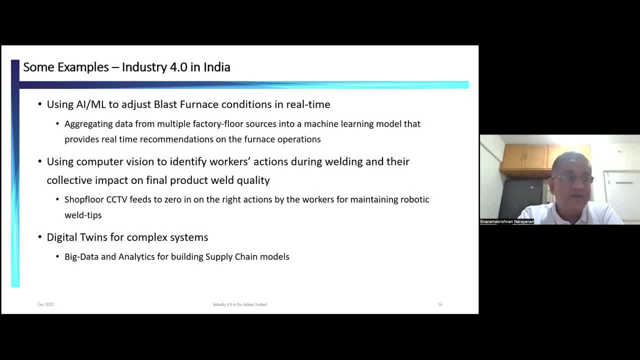 you know those kinds of things. So there is going to be always this debate. There is going to be a lot of ethics that are involved. You know all those thought experiments about self-driving cars and should it kill an old woman or should it kill a bunch of school children? 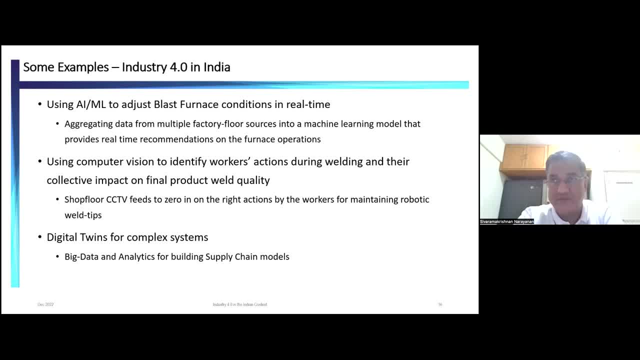 if confronted with such a moral dilemma? These are all famous problems in artificial intelligence, None of which, for none of them, I have any solution right, But there are better minds than me that are occupied with this, these problems, And I'm sure we'll find a way or we'll find a compromise. 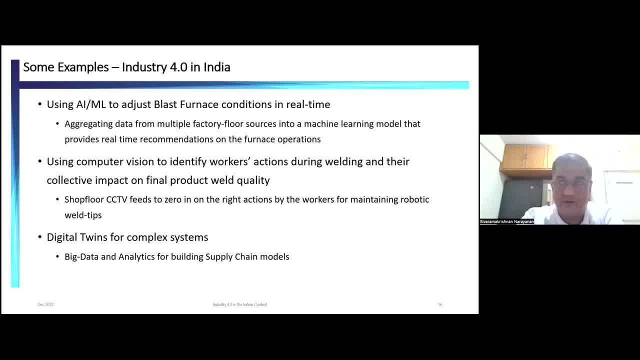 that looks practical, agreeable, ethical and all of that. But you know, while here, for me the role today is to play the cheerleader for a lot of these technologies, And I am doing that job. There are also a lot of ethical, moral, societal. 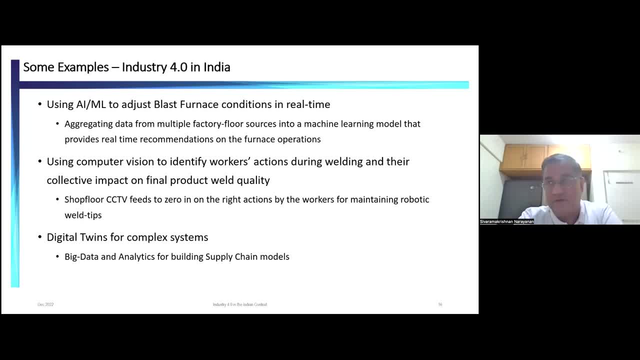 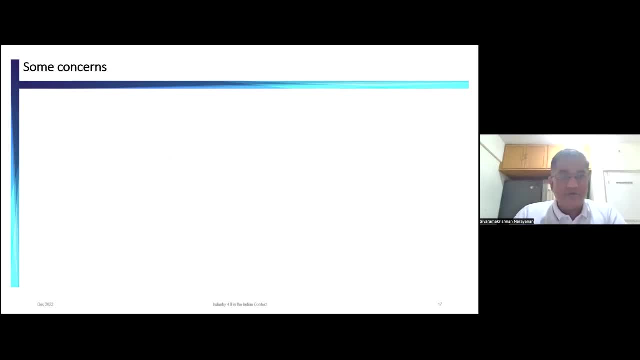 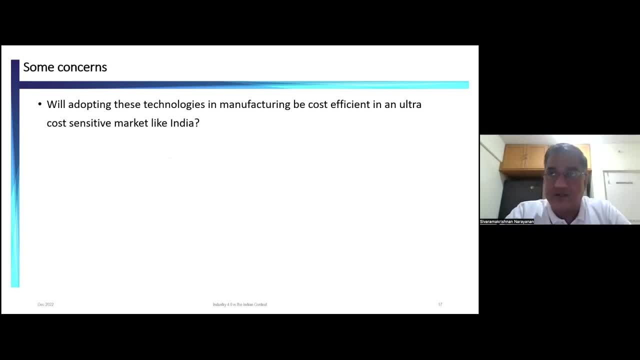 How can we protect ourselves? And the second question that was asked by one of the participants is: are these even relevant for India? Right, Is industry four relevant for India? Should we do something else? Industry five: I think that is one of the questions. 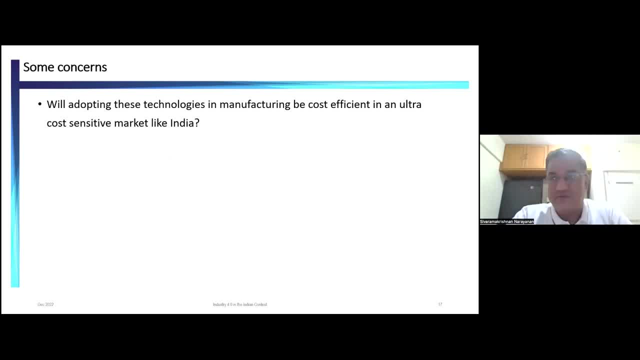 Right, No. So I think we have to learn to stand before we run, We have to learn to stand before we walk. even Industry four would be the place where we go. Of course, industry five is already taking shape. Technology always, you know, advances in leaps and bounds. 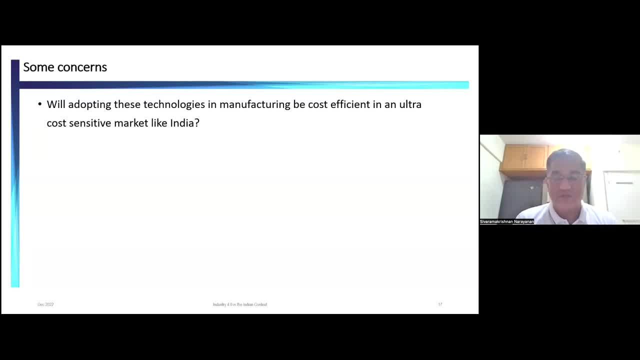 but we as a society need to adopt those technologies that make sense for us and industry. 4 in my view, in my personal view, I think, makes a lot of sense. it has huge potential for improvement in society, for improvement in our productivity, for raising the livelihoods. 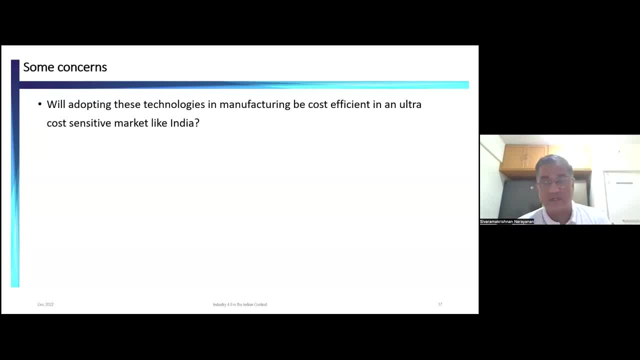 of millions of people, just like IT and IT services did it between the time that the prime minister, PV Narsimra, opened up our economy along with Dr Manmohan Singh, and we have really taken off. the kind of lives we lead today are far different from the lives our parents led just a generation back. 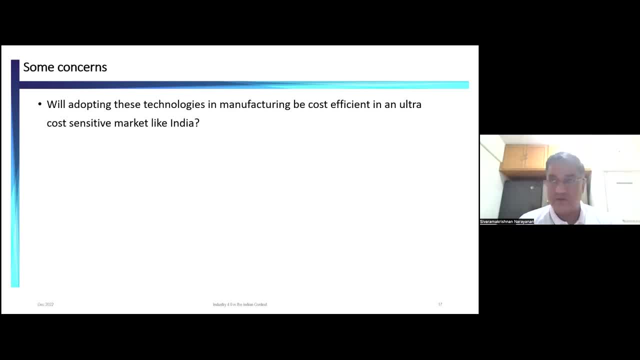 so industry 4 is the way to go. industry 4 is very relevant and I believe manufacturing, being the vehicle of growth, would be the, you know, the right way to go. so would it be cost efficient would be the second question that comes to. would it be cost efficient? right again, the answer is maybe. I will not say it's. 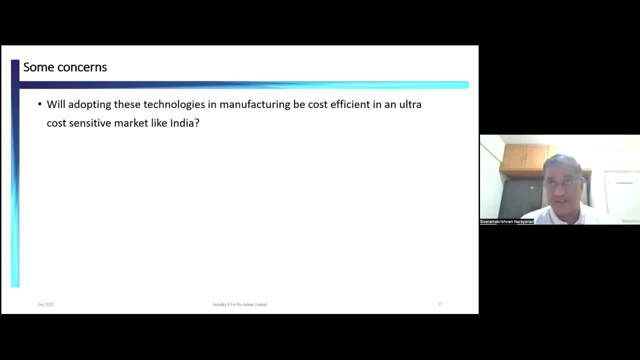 an unqualified yes, because a lot of these technologies today are expensive. right, a robot is probably as expensive as 100 workers working for a whole year. would it pay off in the long run? yes, so we need companies who are committed to this in the long run, who are willing to stay. 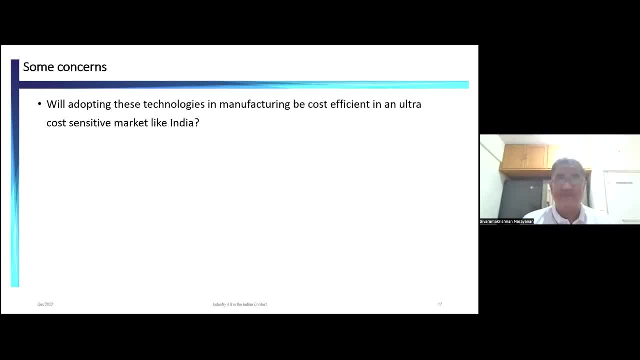 the course for, say, five years at least, invest in these technologies, allow them to mature, be stable in the environment that they are working in and not look at this as a quarterly revenue kind of and ROI based investment right. so so there are dimensions to this. it would depend on the 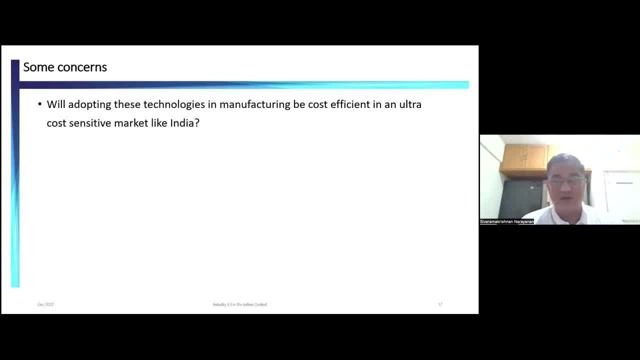 industry. it would depend on the like. if you say, I will put in a chatbot in a in a tourism industry, the answer would be obviously no, because tourism requires a lot of high touch, right, high interactions with the customers that you have. putting a chatbot in such an area would be a 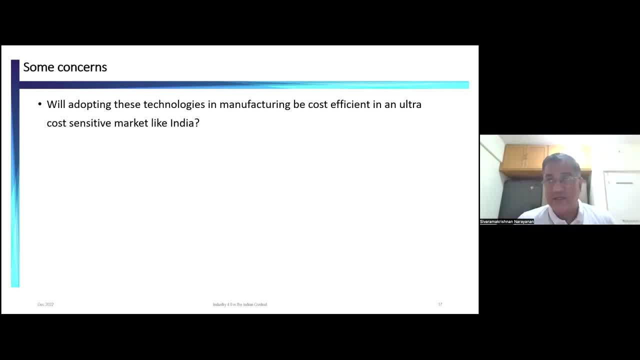 bad idea. so there will be areas where cost efficiency is not the primary concern. there would be areas like BPO where cost efficiency is the primary concern. so it would be selective. it will be in a sense contextual and industry has to adopt technologies where it makes sense and where 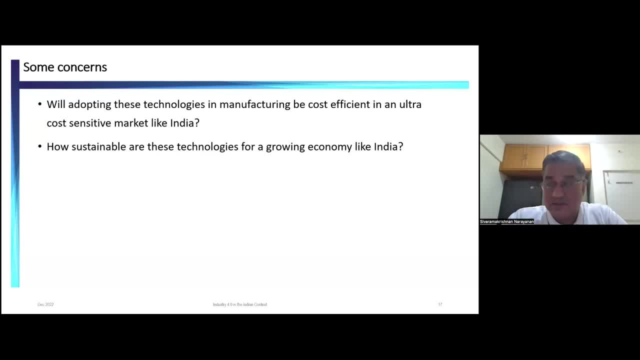 it doesn't. it should not. are these technologies sustainable? again, it's a qualified yes. exactly the question that Professor asked earlier, that if I start putting a thousand data points for every piece of manufactured item into a data center, will my data center not become a huge carbon? 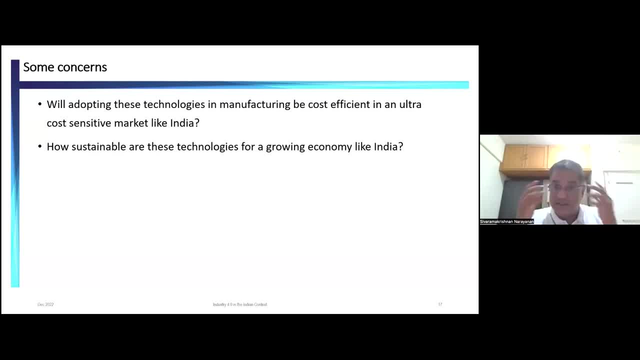 energy, a carbon green gas generator. the answer is yes, it will. the question for us then to answer is: are the productivity gains and the visibility gains that I get out of this, excuse me- going to offset these gains, these disadvantages that I'm getting out of greenhouse gases? it's a qualified yes for. 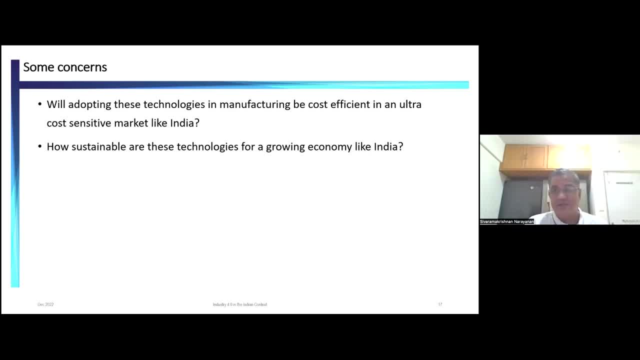 now because I being more from the manufacturing and the industry side, a technology like this offers immense possibilities for productivity and growth, and those are the two primary factors that that play in my mind. sustainability is something that I'm still learning how to build: sustainability in the solutions that we bring as consultants to us. 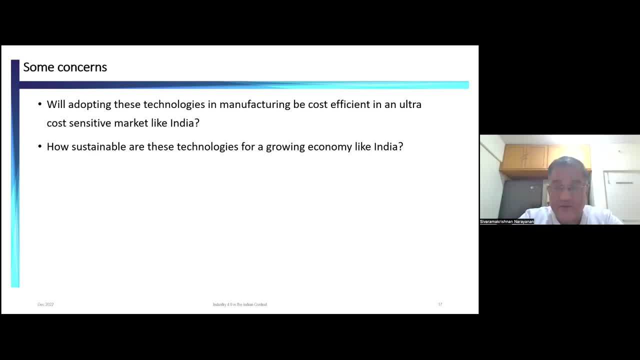 clients. uh, that's something that I I don't have the wherewithal to answer today, but the answer should be yes, they are sustainable. they should be made sustainable. will we give away our inherent democratic demographic dividend advantage? you know we read a lot of articles saying the next. 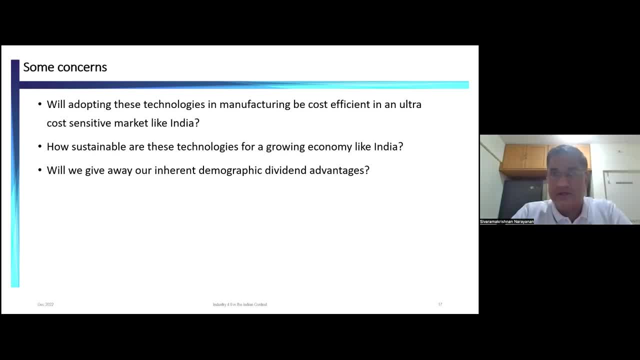 30 years. we have a lot of young men and women in the in the workforce we have. you know, our young people will go on till 2060.. a lot of us will not many carriers left at that point in time, But at that point in time 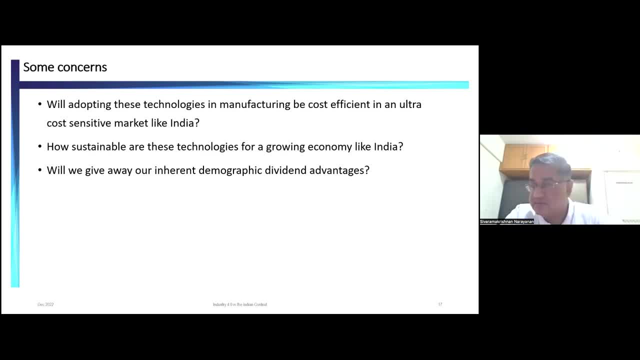 the demographic dividend will end for India because already growth rates, birth rates, are falling. Will we give away our inherent demographic dividend? The answer is no. I would say no. We are not giving away our demographic dividend by adopting these technologies, because a lot of the people 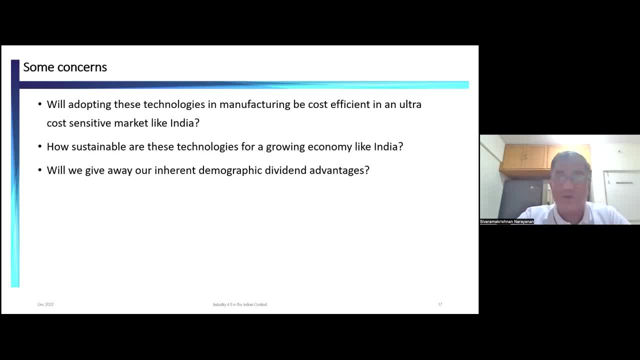 that are coming into the workforce will work in jobs that we don't know today. The jobs that will exist in 2030 will be dramatically different from the jobs that we see today, And for reasons I cannot fully articulate in a conversation of this nature. 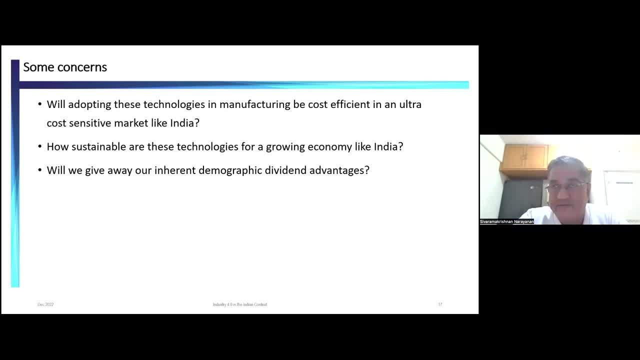 but there are several things that didn't exist as recently as five years ago that exist now. You hear a lot of data scientist roles. If I had asked you a data scientist in 2010,, 10 years back, I'm not sure if I would have got. 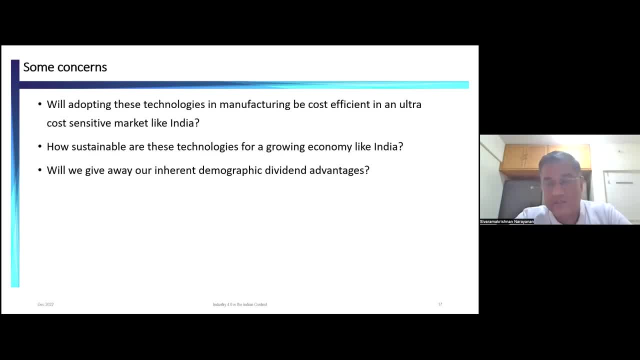 a consistent answer across, Let alone a large audience, right? So there are jobs that we have today, like YouTuber. YouTuber was not a job in 2007.. Today, there are people making millions of dollars by being a YouTuber. 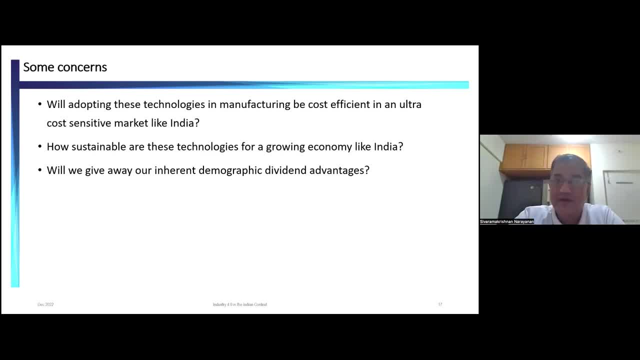 or a TikToker for that matter, right. So some of these things are very, they are curious. They are curious phenomenons of our society. Some of them are here to stay, Some of them will go away, But one thing is sure: 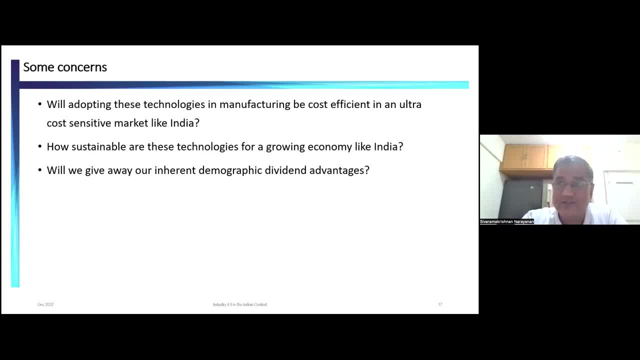 That we will not give away our demographic dividend because the young men and women will be doing a lot different jobs. That will be freed. I mean, just imagine we have, I don't know, close to a million sanitation workers in India. And if you had sanitation robots? 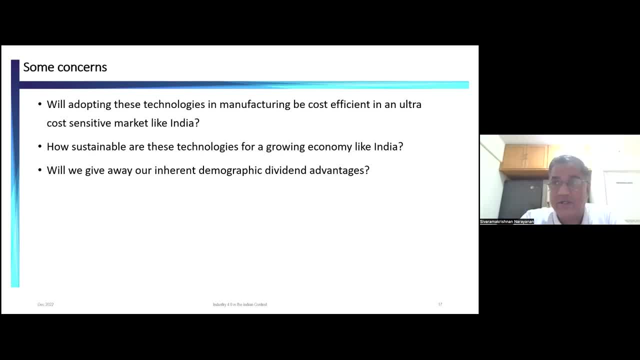 that cleaned up our drains. that's a million people that we can otherwise employ. right, I'm being a little bit dramatic here, but you get the picture right. Do you want your young men and women to be sanitation workers, or do you want them to do something more meaningful? 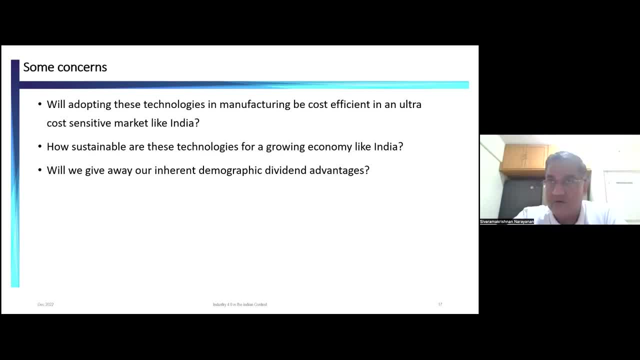 If I ask that, the answer would be obviously no. I don't want people to be sanitation workers. They are doing sanitation work because they don't have any better opportunities. So if I can create those opportunities by using any of these technologies, then I have some dramatic impact on the society. 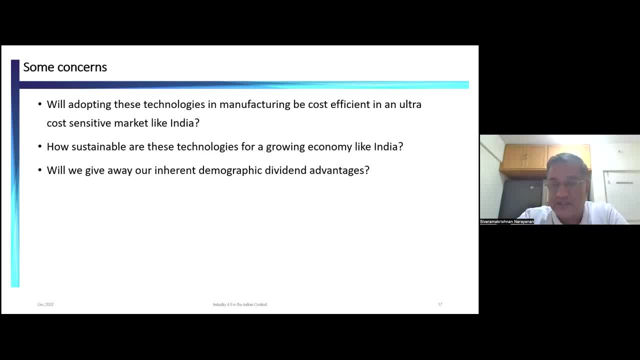 Maybe all million will not get out, Maybe half of them will, But that's a dream that we can all aspire to have. Do we have necessary skills? No, at the moment, And you know, I don't know, I don't know. 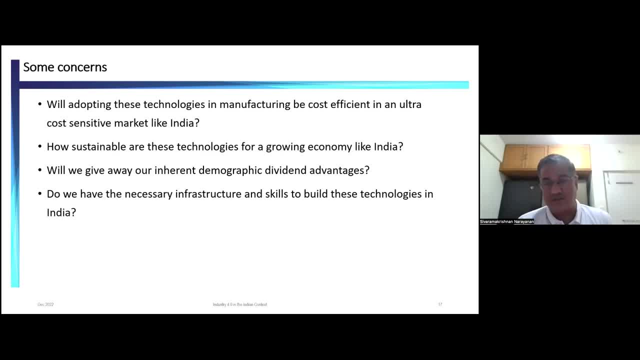 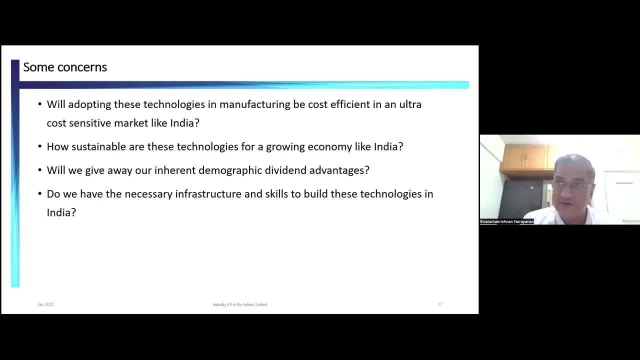 but training that makes a real economic difference to the people, to the people that are not writing IIT exams. You know government jobs across India, whether it's in the south, north, east or west, have applicants, you know, for every seat. 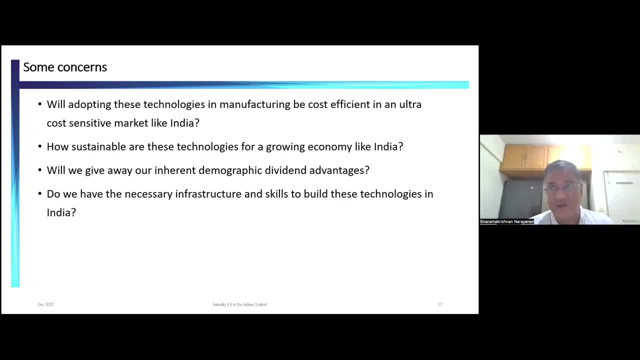 there are 100 applicants writing that exam and people overqualified for that exam. So you know, not getting jobs for years and so on and so forth, because simply they don't have the skills and they want a government job to just secure their future. 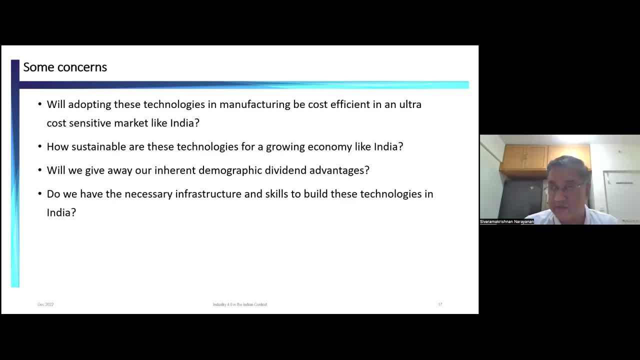 Can we secure their future through skills? The answer is yes. We have to provide those infrastructures to them, And the more we make our people skilled, the better we will be in a position to use these technologies and grow The impact of skilling our people. 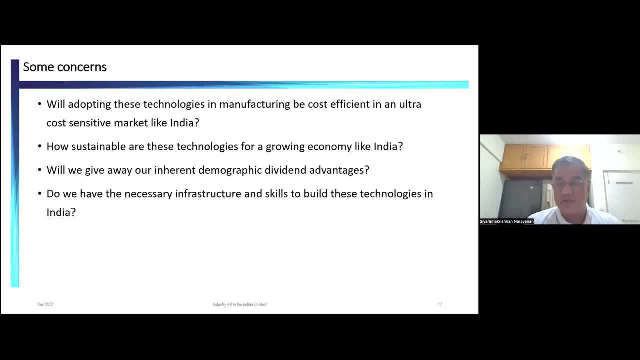 making use of their skills to open up opportunities that did not exist before is immense right. I mean, I cannot overstate the importance of skills and learning, And I think India is waking up to this possibility that we may lose our demographic dividend if we don't skill. 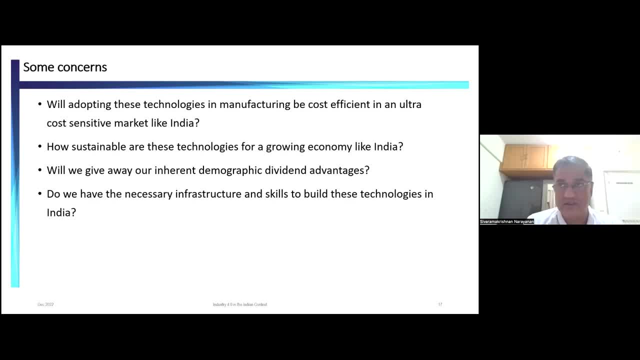 our people adequately in time. So there is a lot of trust. There is a lot of importance being given to skilling people, to educating our children in the right way so that they come out with literary and numeracy skills that can earn them a rupee. 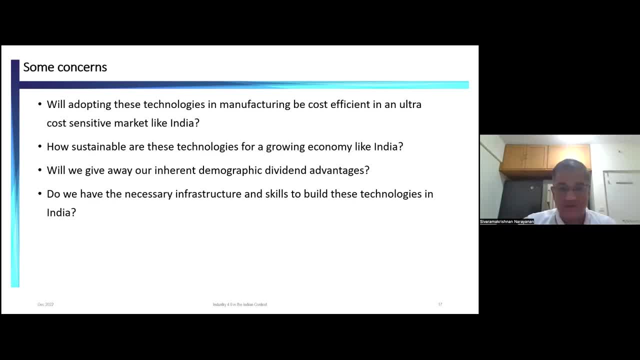 in the market right, And that's important. It's important for us to build meaningful jobs. Will they take away jobs from new Indians? No, The answer is no. They will actually free young Indians to take up jobs that make sense to them in the longer run. 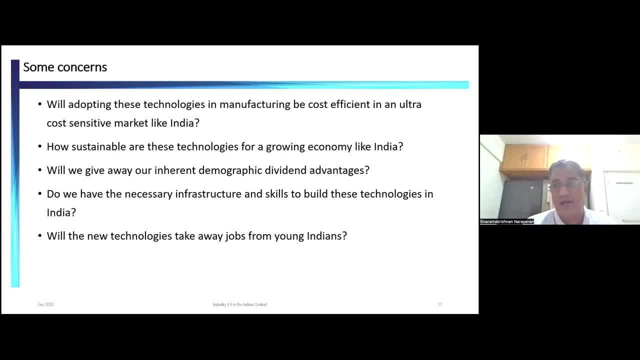 And this is something I believe very strongly. I am a very at my heart. I'm a very technology savvy, technology friendly person. So I believe technologies will free us, will make us more productive. I see the positive effects of technology on society. 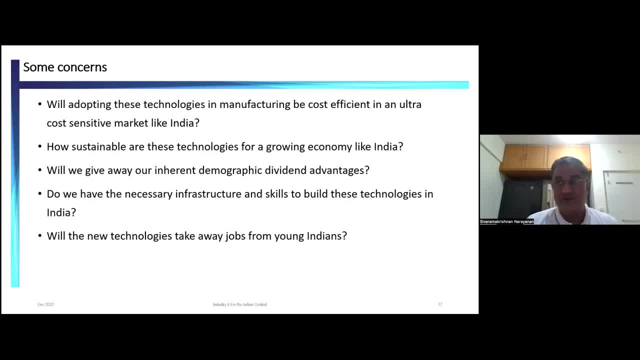 And that will result in leverage for our young Indians. I'll give you a small example. I was volunteering for a. you know, giving my time for social causes. Diversity and inclusiveness in Indian society is pretty low. Those of you who've traveled- 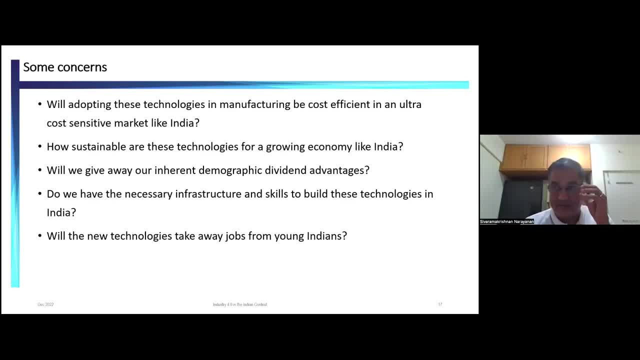 in and out of Bangalore would have seen Mitty Cafe in the airport. Now, Mitty Cafe is a cafe by a young Indian who has taken upon herself to provide employment- meaningful employment- for disabled people, people with Down syndrome, people with hearing disabilities. 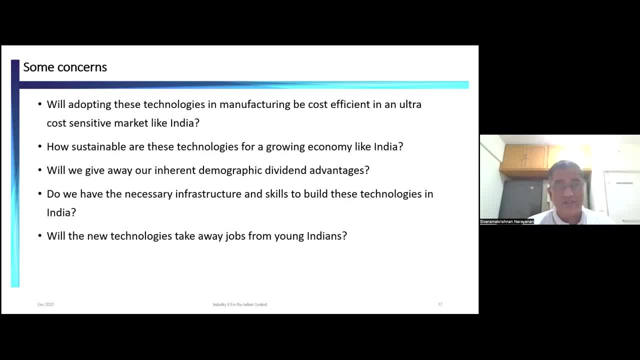 or you know, blindness and so on, And they have a lot of pride in the work they do. They actually serve. it's a cafe. they serve you snacks, tea, coffee, and they serve it with such joy. Your heart is filled. 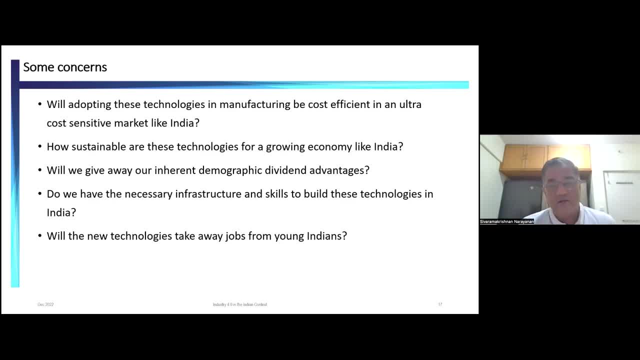 not just you know your craving for tea or coffee or a snack, but you're just overwhelmed by the amount of pride these young men and women display when they're doing something as mundane as a job: serving tea or coffee to people Right. 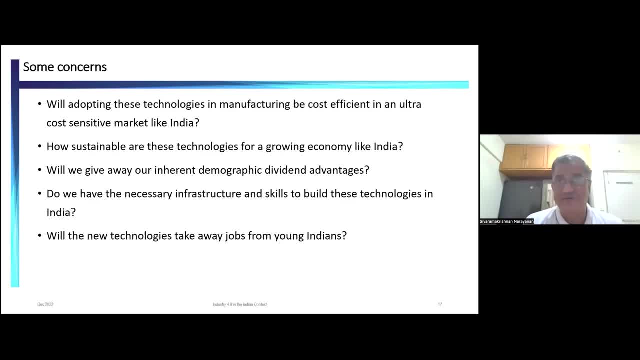 Now imagine this multiplied a hundredfold if you were to create jobs for disabled people, people because of artificial intelligence or machine learning, or touch sensors or any other different types of technologies that we have today- robots- You can imagine virtual reality, augmented reality, 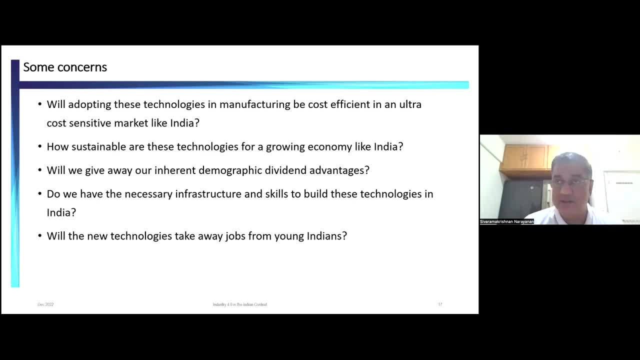 You have a person who is a hearing, a disabled person, who is working in an Amazon warehouse and she is able to look at a warehouse shelf and understand what is going on in that shelf. What is the product? What has to be packed next? 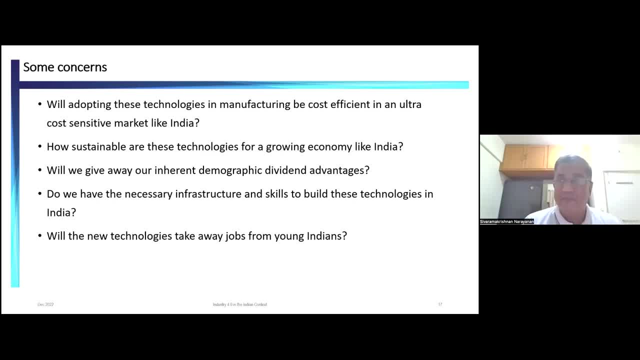 What has to be, where should it be shipped? She makes those decisions because technology is facilitating. Today we see a lot of blind people that are able to use a computer like this, like a laptop, because there are voice-activated commands. 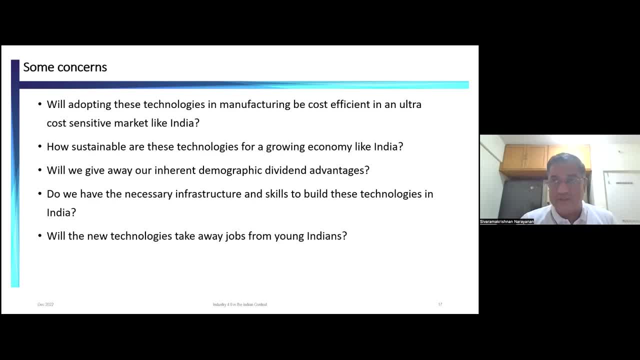 Right. These are all small examples of how we can bring technology to help people with skills or abilities lesser than an able-bodied young man or woman to be productive Right, Instead of serving coffee and tea if such a person was also able to make a mobile phone. 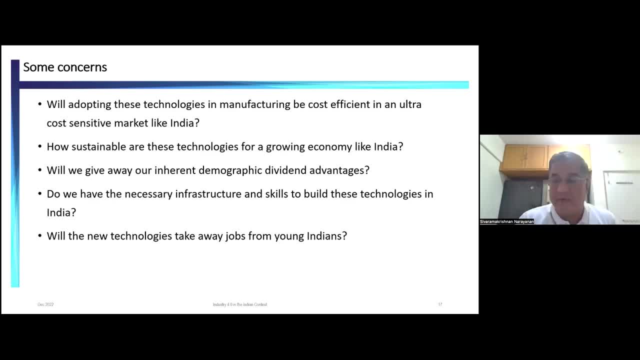 or send out a package to a customer in some part of India. that person would be so proud of the job that they are doing that they will actually bring 10 more people into the work life, into the work life, And these are small jobs. 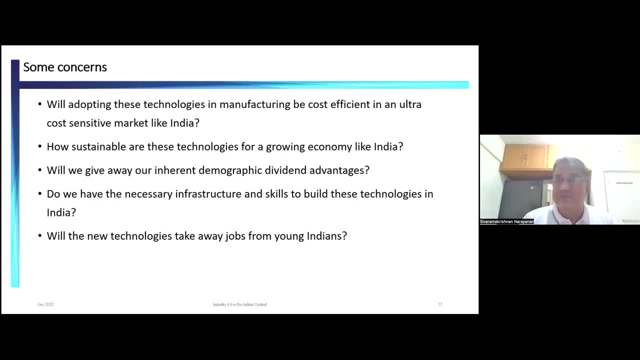 These are not- I'm not talking of some rocket science kind of jobs. These are everyday jobs. These are required to keep our wheels running. Healthcare workers, You know there are so many opportunities which technology can open. this kind of technologies can open. 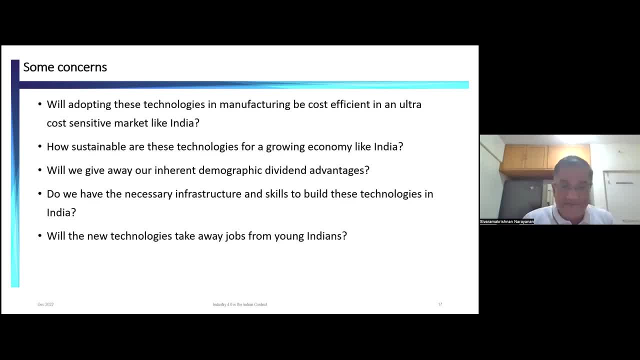 that I don't believe that jobs will be lost. I believe jobs will be created, Right. So that is my take on this whole thing. That brings us to the end of the hour. I have some references in the deck. I'm sure this will. 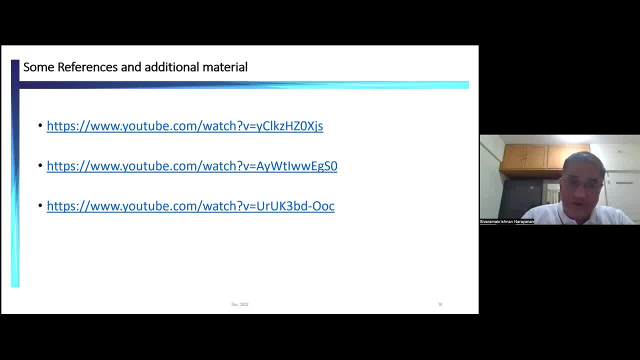 be of much use to you. These are all on YouTube. They are available publicly and I would love for them to be watched by you. There is a TED talk. There is something around Industry 4.. There is a lecture. Please have a look. 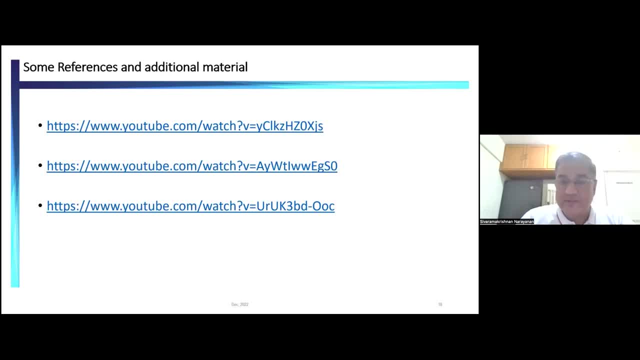 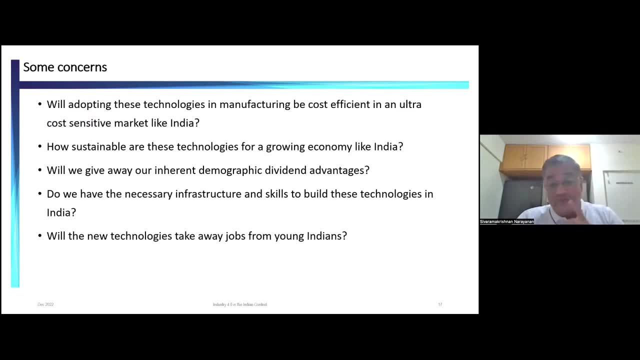 I mean, these are incredibly insightful videos. Please have a look and, you know, I hope some of you can make a journey start One last thing right: What kind of skills do you need today? That is one of the questions that came up. 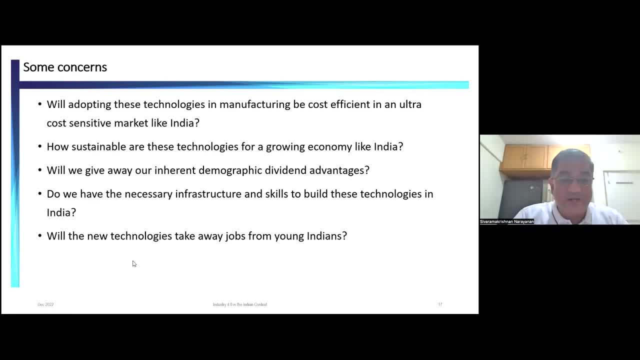 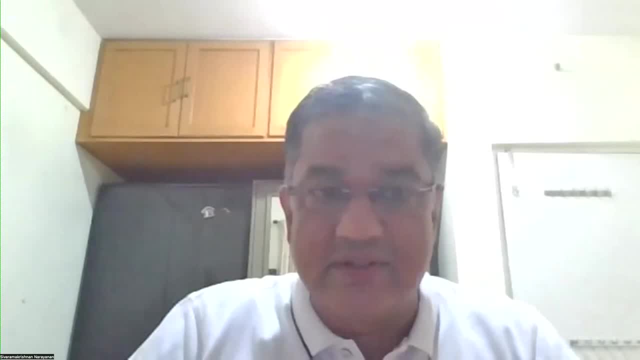 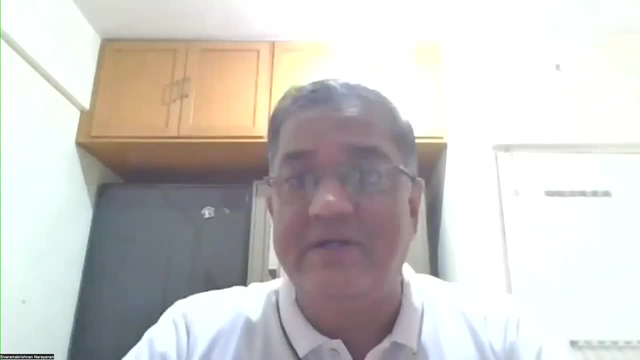 Sorry, I'm just looking at the Q&A. What kind of skills do you need? Skills that you need we already. excuse me, sorry, I should close this. Skills that we need are essentially around data, data management, All this. 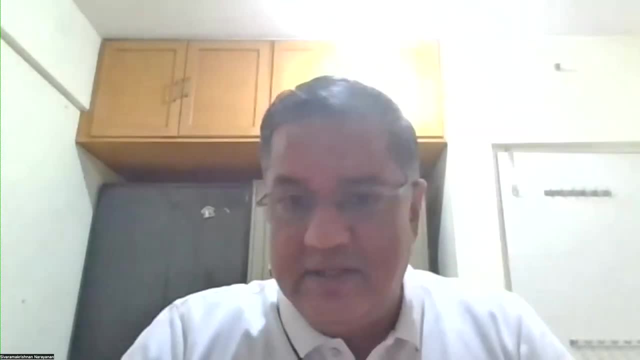 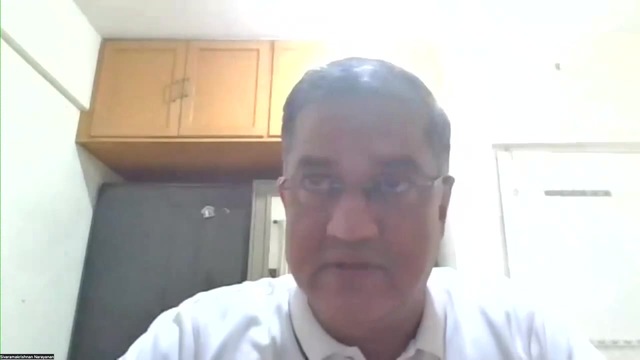 we have an inherent advantage. I think that was one of the questions. We have an inherent advantage because we already have a lot of these technology skills. We are an international service-driven economy, very connected to the Western world. We deliver a lot of services to them. 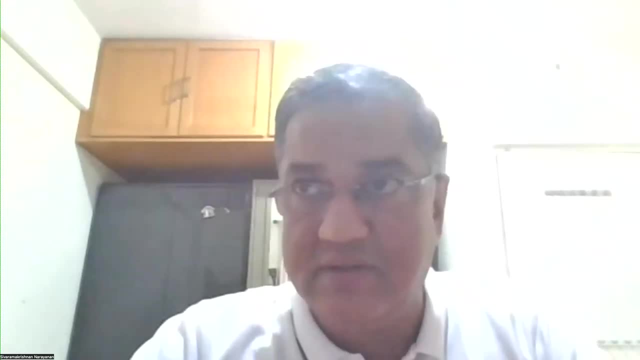 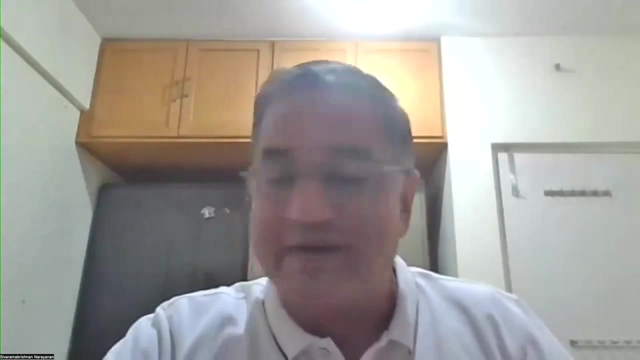 Some of those will translate to better manufacturing product capabilities. We have a lot of issues in manufacturing Today. we have, you know, a lot of industries that I go to. they talk about the seasonal workforce, right? So people that are cutting sugarcane. 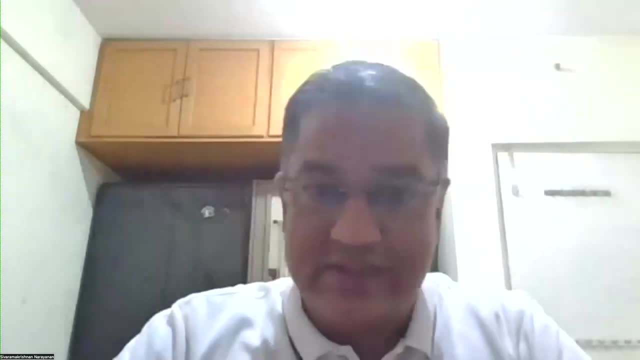 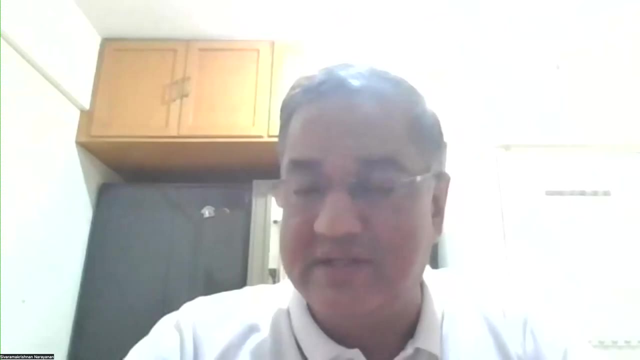 during the sugar season, come to work in factories during the non-sugar season, right? So between cutting sugarcane and assembling an automotive vehicle or working in a steel factory, there is a huge difference, And that brings a lot of skill gap to our manufacturing. 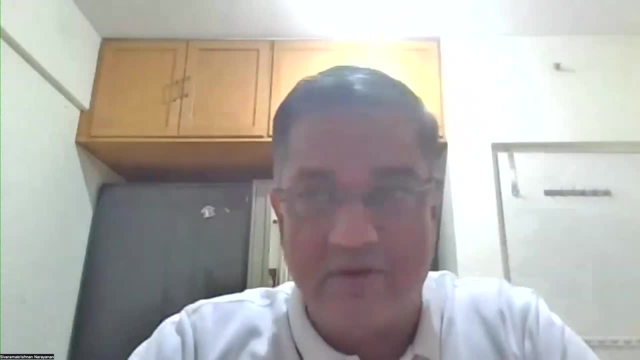 Our chalta hai attitude, which is not normally a good thing, impacts the quality of products that we generate. So the diligence and the quality that we can see in a, for example, a Vietnamese product is not there in an Indian product, And that's something. 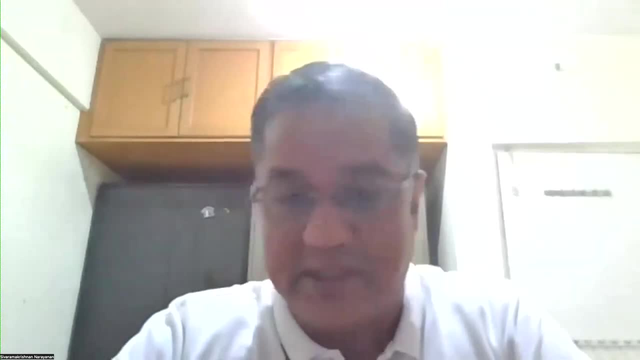 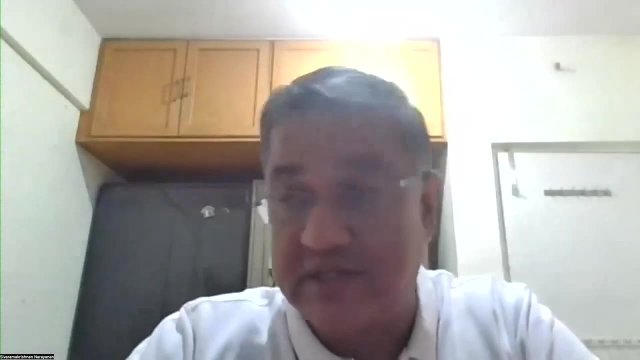 we have to fix as a society, because that's not just the job of the government to do. So there are a lot of things that we should do. we can do. What are the skills? Currently we have a lot of those skills. 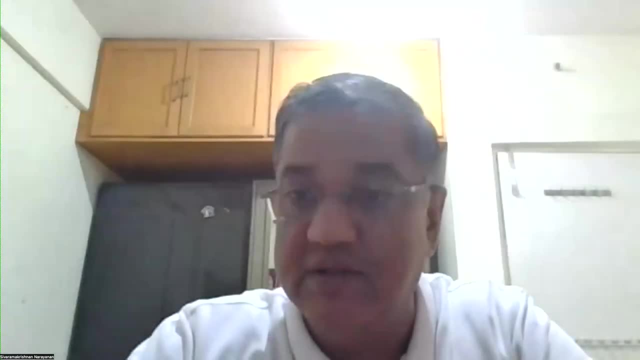 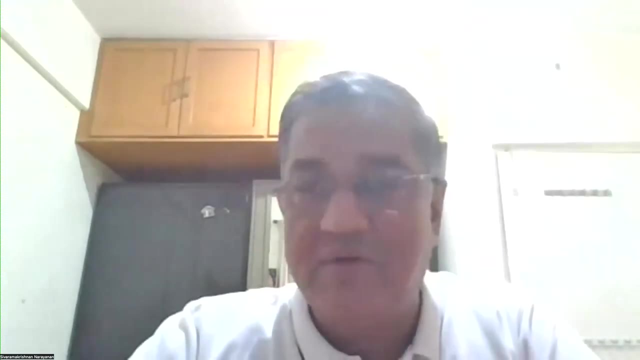 We have a lot of skills. We have a lot of understanding of the market driven demands for services. the quality, the diligence, the discipline that we need to do. And I'm not talking of the technology skills at all, The manufacturing technologies for the moment. 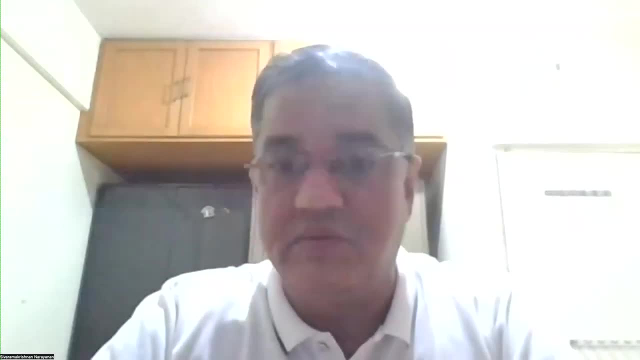 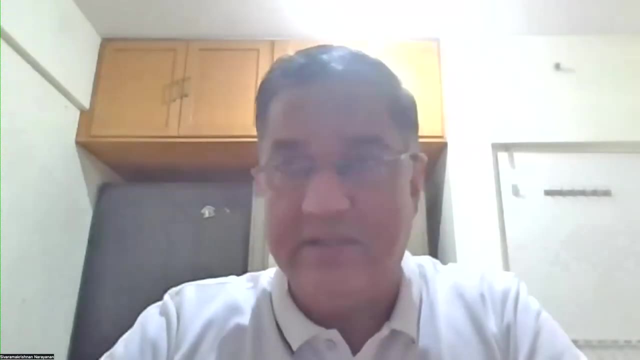 we'll have to probably buy import from Western, the Western world or even China or Japan, But there is something that we can bring that is unique. There is one. there is a large population that we can bring. It's almost an endless well right. 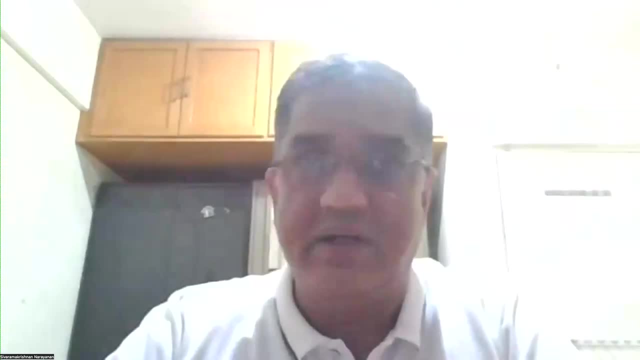 We can bring people at will, and we do bring people at will, and that will make a huge difference. We can bring a lot of quality education to the table, which is one of the main differentiating factors in manufacturing. as we go along this journey, 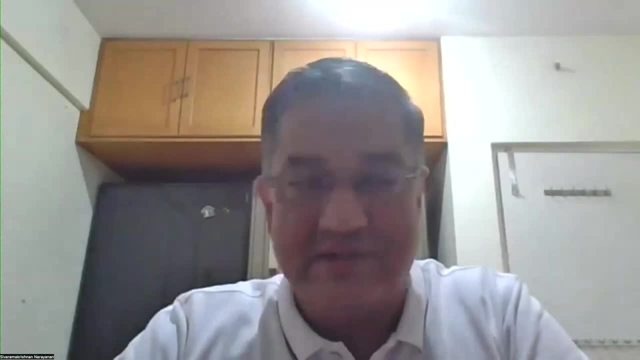 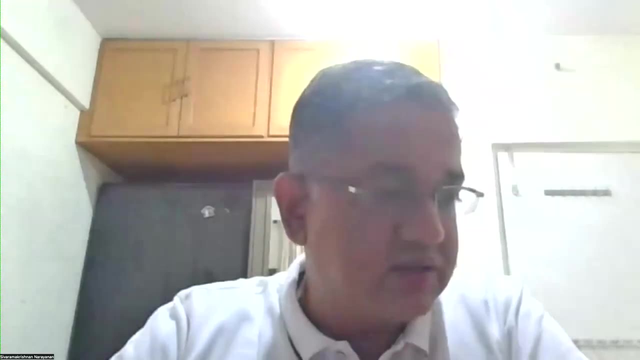 And we have a demographic dividend that is expected to last for another 40 years- And that's an incredible amount of time in a country of our nature- And we will cross our 100th year still in the middle of the demographic dividend It's for us to seize. 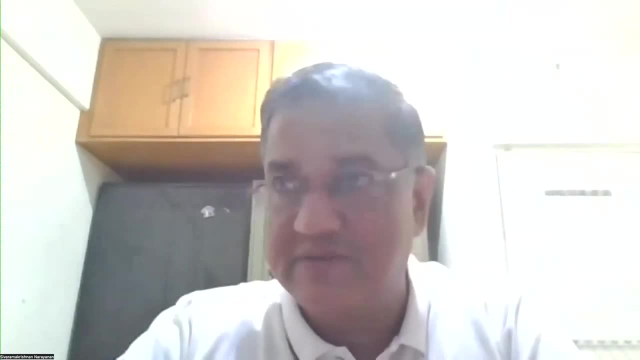 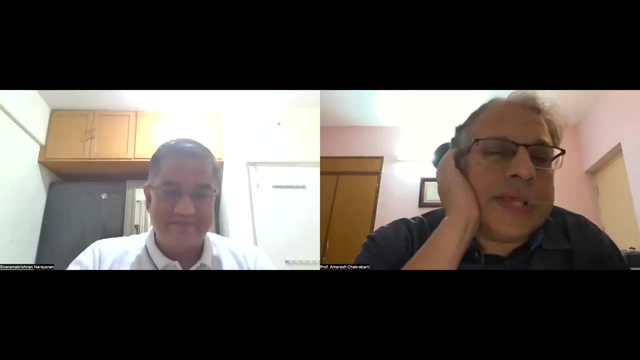 this moment and make it happen for ourselves. Thank you so much. So, Sheila, Thank you. Thank you again. Maybe we just take two or three questions, So maybe there is a question that someone was saying that we also hear of the industry. 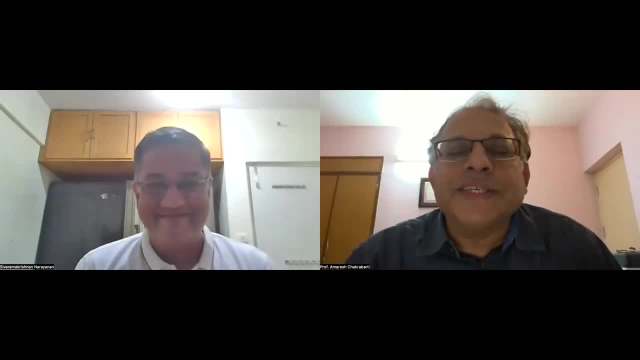 5.0.. So would you like to just distinguish industry 5.0 from industry 4.0?? Yeah, So I don't have the expertise, professor, so I must dimmer. I spent a lot of time in industry four. 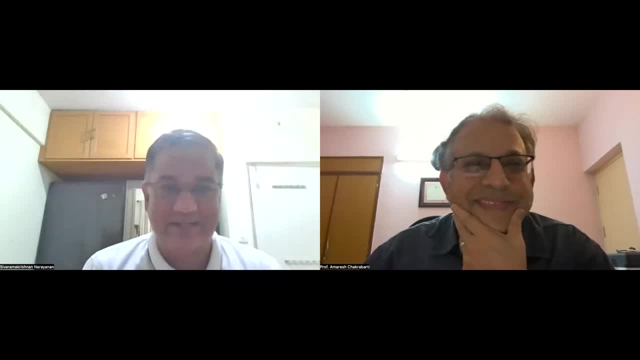 I don't understand fully at the industry five concepts, so I must dimmer. There's a lot of time in industry 4.0, I don't understand fully at the industry 5.0 concepts, So I must dimmer. 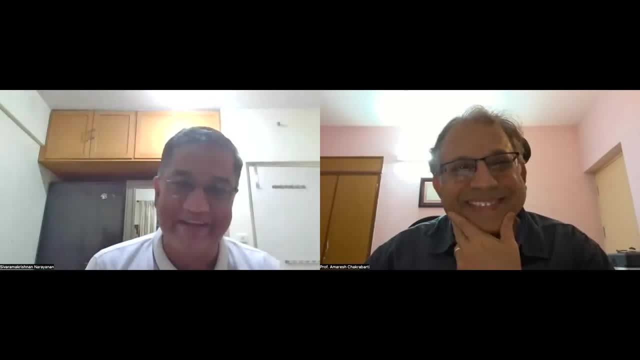 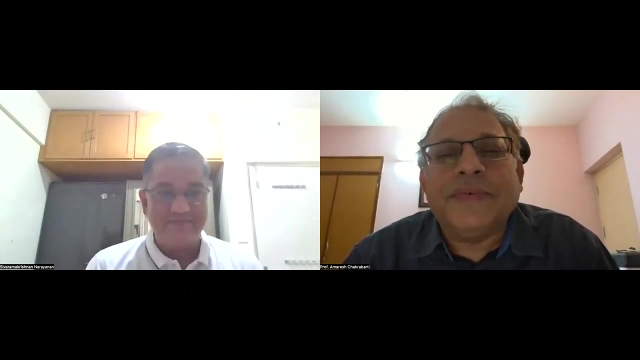 I must park it for another time so that I can do my own research before I can make an attempt at answering this. Okay, So let me give my sort of thoughts on that. The industry 5.0 is really, you know, trying to say that we need to make industry 4.0. 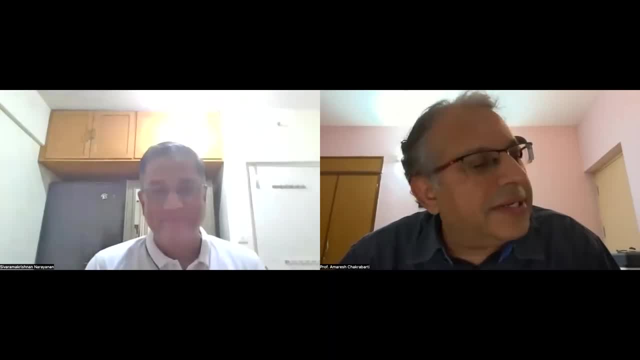 more people-centric and people-empowered. So that's what industry 5.0 is about, And there are different names again for these, just as industry 4.0 also have other names, such as smart manufacturing and so on, And Japan, for example, calls it society 4.0. 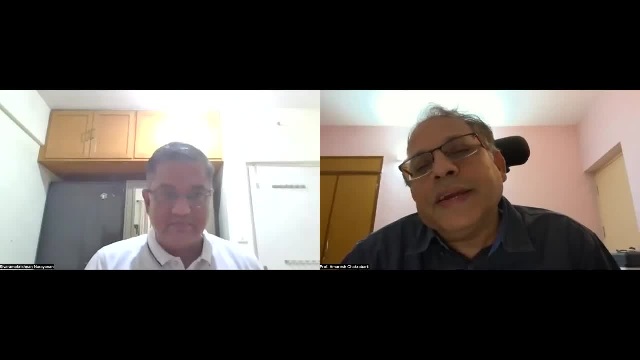 or 5.0,, I think, because they sort of look at it as the pre-agreedian society to agreedian society, then industrial society, information society and so on right And finally now the kind of society that we're looking for, where it is human-centric society. 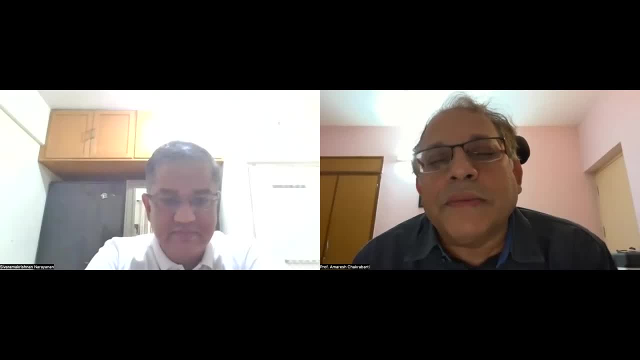 So that's the sort- I think the paradigm- of thinking. I'll just move on to the next question. I think these questions are asked in multiple ways. You know one: we are worried about the competition from countries that have better cost advantage. 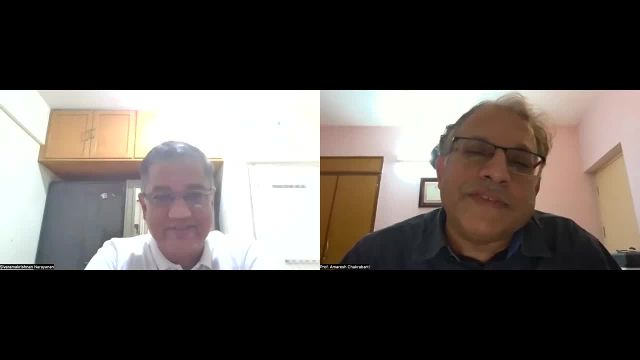 and also countries that have better- what I would say- knowledge advantage. And then you know, somebody has also asked: you know, Israel is more innovative, Why can't India be? and so on. So I think it's a very interesting question. 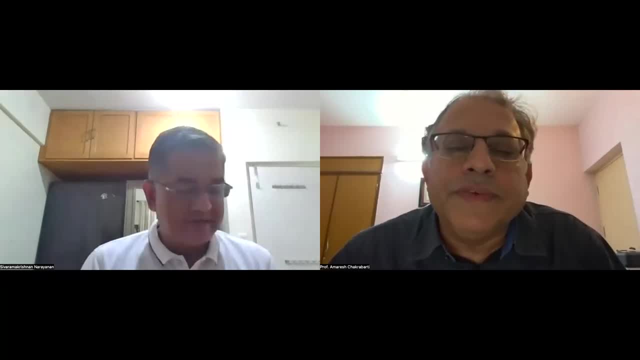 which is that what's the distinct in nature- apart from democratic dividend that you have already spoken about- that distinguishes India from others, so that it can also have its claim on a portion of this pie. So thanks, Prof. I think that's a very interesting question. 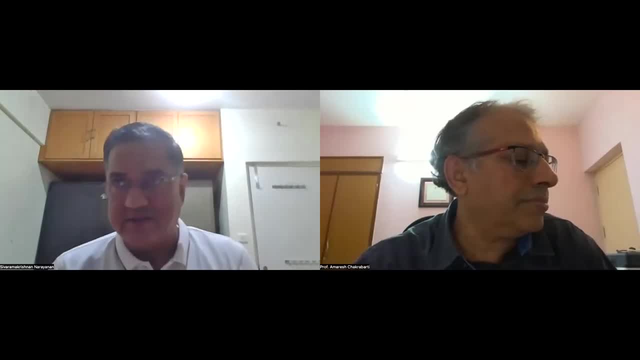 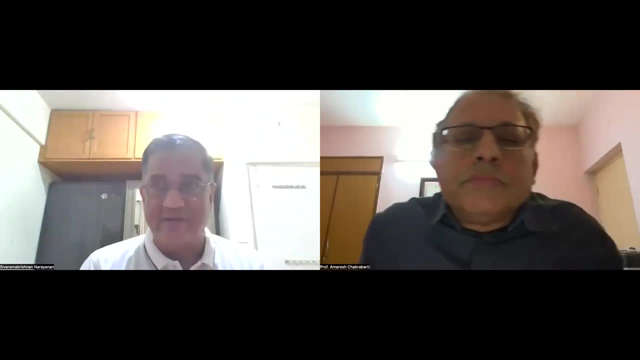 But actually, as an industry practitioner- or as industry practitioners- I think you touched upon this a little bit earlier- that we should focus on delivering value, right? The question for us is really: and if we can make radiator caps, world-class radiator caps. 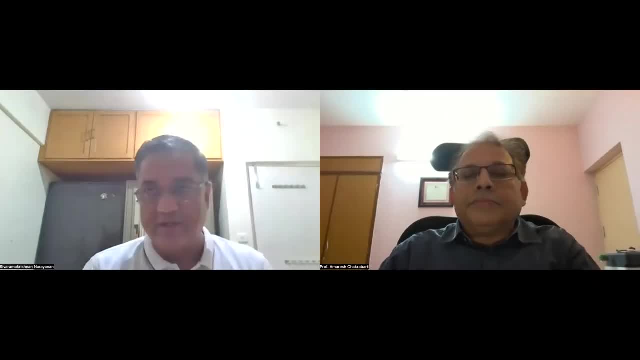 you know, as part of the TVS group- and we all know their story to quality, we can do anything that we want right, And you know this. I can. for those of you who are from Bangalore, I'll relate this to a very everyday example. 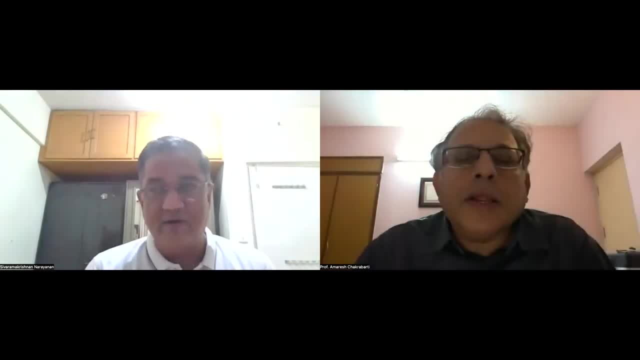 Darshanis- right. We all have had experience in eating in Darshanis in Bangalore right Today in Bangalore. it's one of the modern cities of India where you can have a meal for 100 rupees or less and feel satisfied that it's a clean 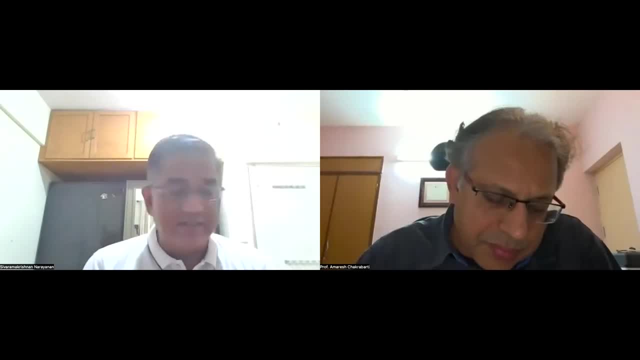 hygienic, healthy meal, And Darshanis have made that happen right. It's not like we didn't have experience of idli and dosa and vadas before Darshanis came in, but the Darshanis found a way to serve that thing. 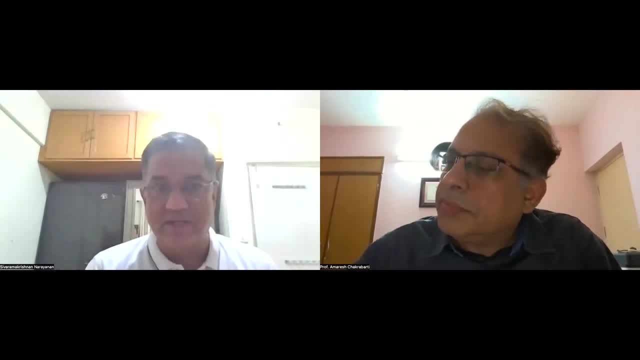 in a way that made value-added sense to you: that it was clean, you could stand and eat. it was not a fussy sitting down on the server and the server comes to you and asking you for your order. You could go collect your food. 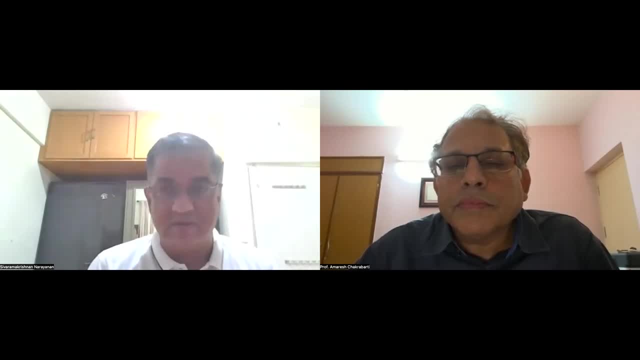 eat it, have a cup of coffee and be on your way in 10 minutes or less. Now, this is value for a customer, For a customer who is in a hurry. he or she just wants an OFAS meal and move on from that thing, right. 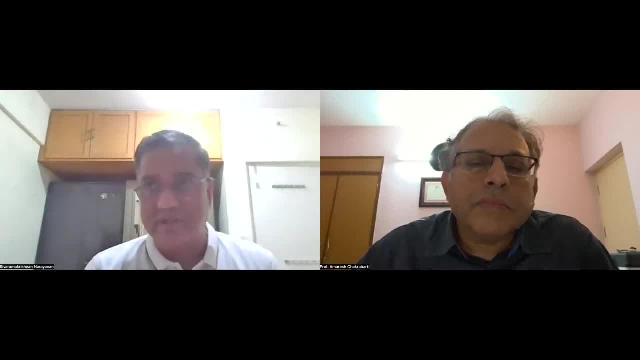 So in this way, there are multiple ways we can service customers across the world. There are customers who are very finicky about quality- Japanese, Germans, South Koreans, for example. There are customers who are looking up to us, as Indians, to deliver better quality. 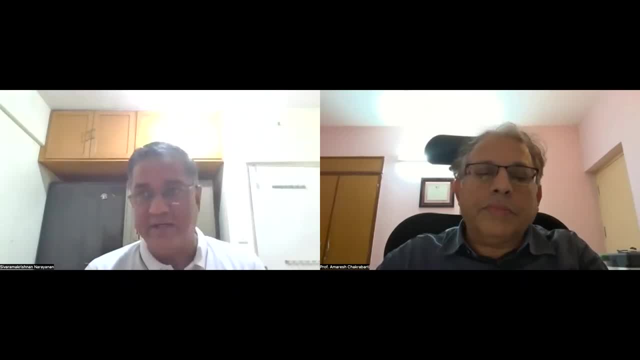 people, probably in the African continent, as an example, right People that we can actually deliver off-patent medicines or healthcare services in ways that they haven't thought about. I mean, medical tourism is a big thing. already. Narayana Hridayalaya is doing seminal work. 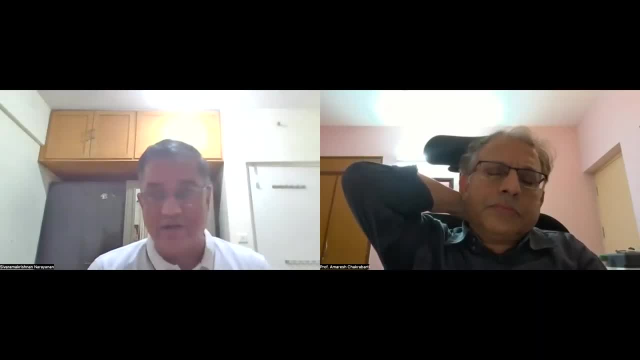 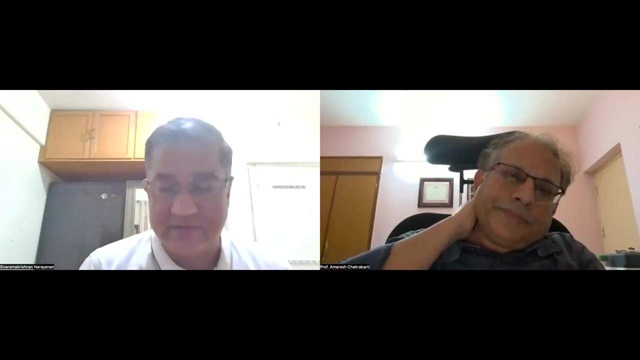 for people in West Asia and northern parts of Africa. People come here for getting treated for cardiovascular diseases. So it's possible for us to be global in terms of services And we have more technology at our disposal than some of these countries have. sub-Saharan African countries have. 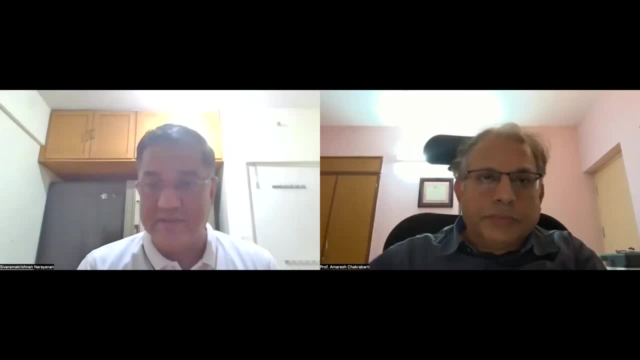 And it works out a lot cheaper for them than go to a Western country. So the answer is for us to find. if we deliver value, if we find the space where India can offer unique advantages, we will win. If we try to compete with others, 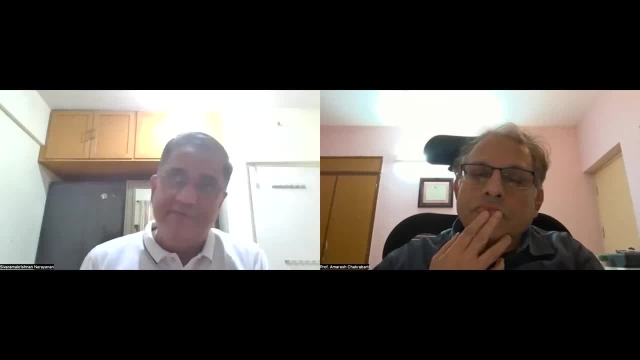 on the parameters of cost, on the parameters of cheap. we may not win, But then that is their game, right? We shouldn't go and play their game, We should play our own game. That would be my solution. Professor, you're on mute. 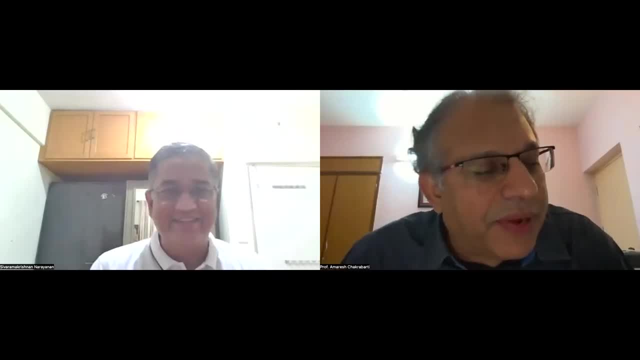 Sorry, I was just going to say that I'm going to add one point and that is the following, And that's sort of the question: The question of: is industry 4.0 for us? I think the answer is an emphatic yes. 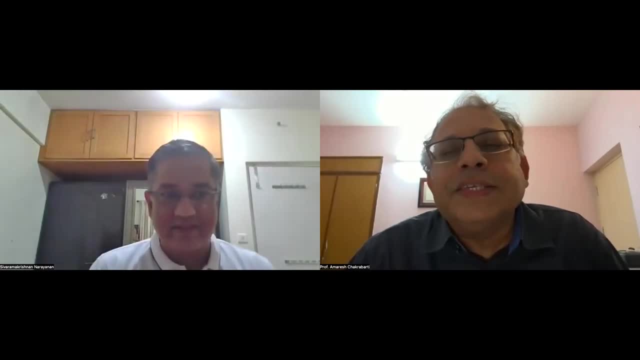 And the reason why it is an emphatic yes is that we need to ask this question. The moot question is the following: Can having data, can having connectivity, can having analysis of that data provide value for any of the bottlenecks, problems, opportunities for you? 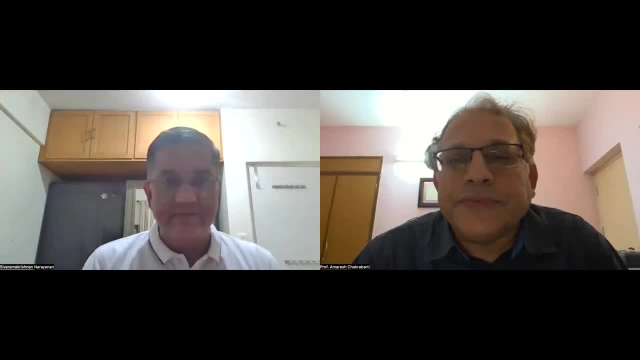 And if the answer is yes, then yes, industry 4.0 is for you, And if it's not, then it is not. So I think I don't know how long more we have, but we don't have a great deal of questions. 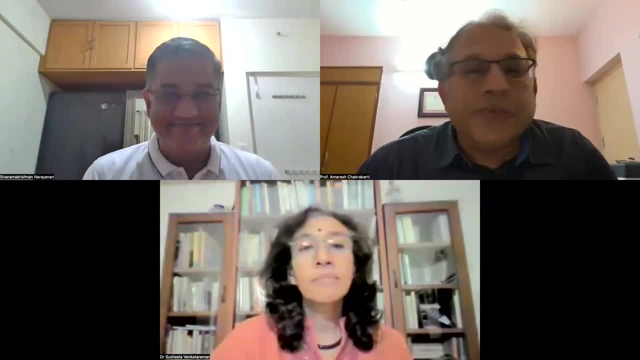 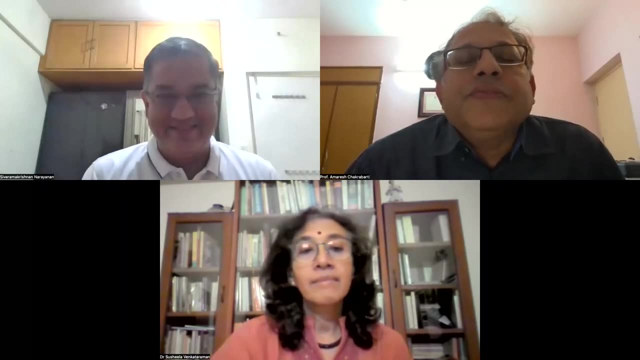 at this point of time. So I'll say that I would like to profusely thank you for bringing a very wide array of points together. It's not easy to give a talk on industry 4.0. And you have done a splendid job. 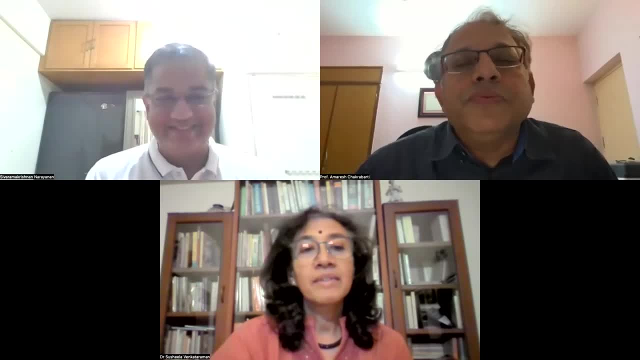 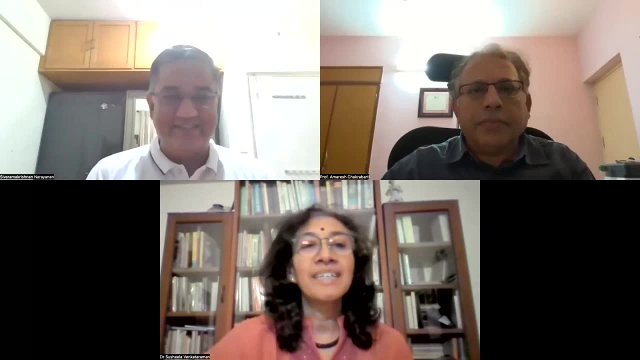 and I'm thankful to you for that, And I'll pass it on to the organizers. Thank you, Thank you. Thanks very much, Professor Amrish Chakraborty and Krish Krish. I've known you, I think, through most of your career. 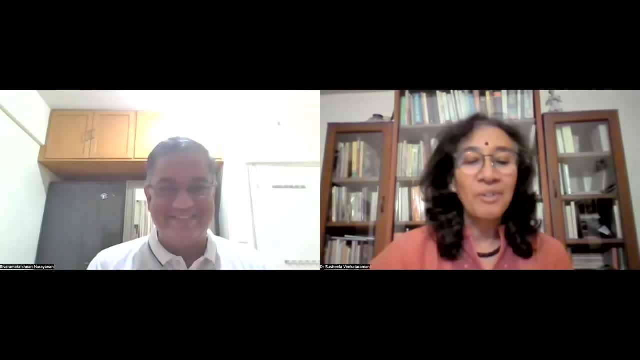 And what stood out today, as it has always, is the same level of systematic and clear thinking and the enthusiasm that you bring to everything that you do. So thank you ever so much for taking this up and thank you for being here and doing this wonderful talk. 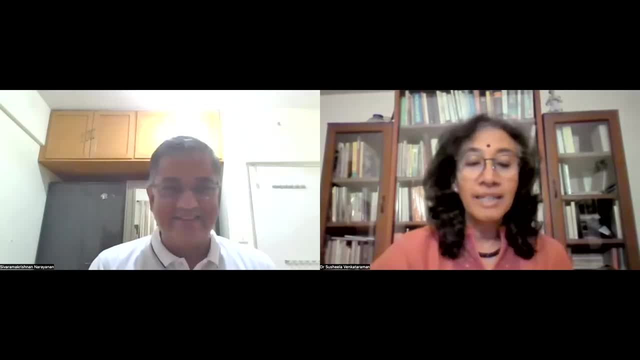 Thank you. I thought the positive tone and especially the examples of the great innovations that are going on right here in India was really, really nice. And the question then is: how do we take advantage of all this good stuff that is happening to get to that 5 trillion economy? 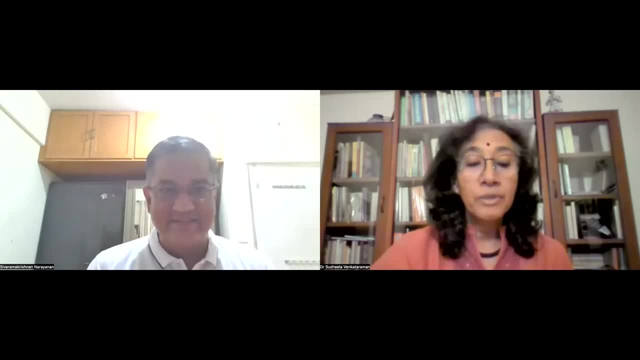 that we want to build, That we want to become, And you mentioned that, from this 15% contribution of manufacturing that we've stagnated at for half a century to looking at moving to 25% of the GDP is not a pipe dream. 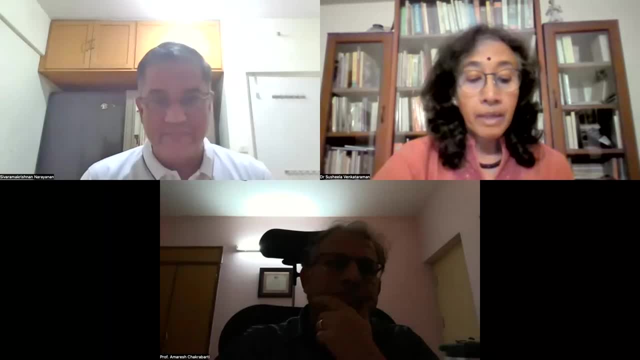 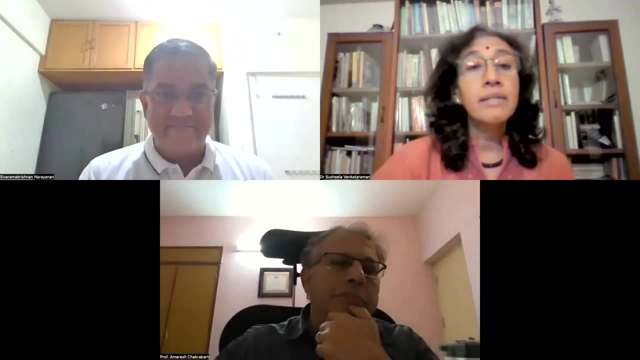 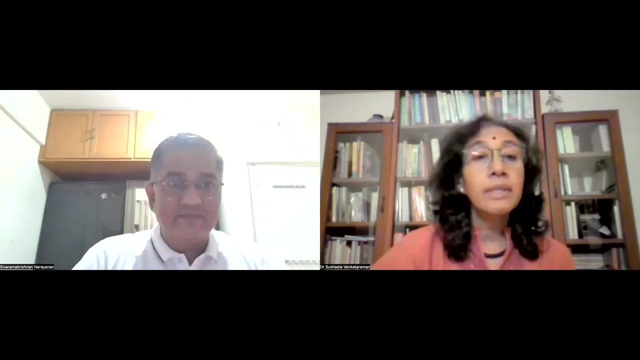 It is something that can be achieved. Okay, so just a few key takeaways from today's session. We looked at various stages of evolution of industry and the first, second, third and then the fourth revolution, which is really industry, what we call Industry 4.0 today. 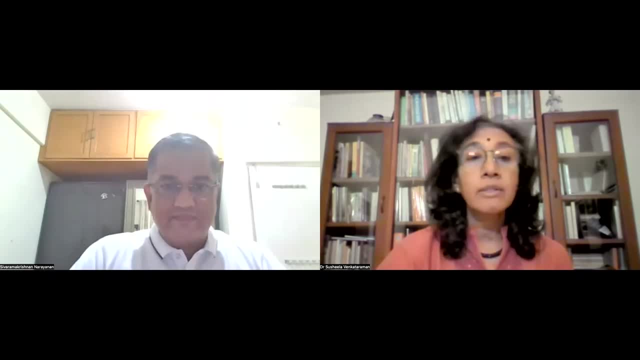 And the key thing there is the cross-disciplinarity of various areas: the physical world, the digital world and biology. So that really is the heart of what has enabled Industry 4.2 to become what it is. And then, as a bonus, 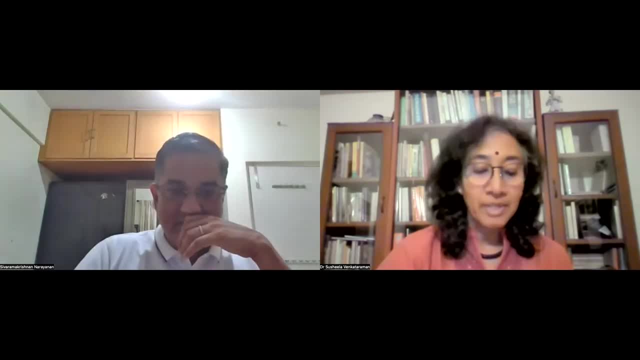 we had Professor Amrish talk about what Industry 5.2 is, which is really a people-centric paradigm. We looked at the building blocks of Industry 4.2, the technology foundations, But for me the more important thing was- I think we've kind of heard all of this- 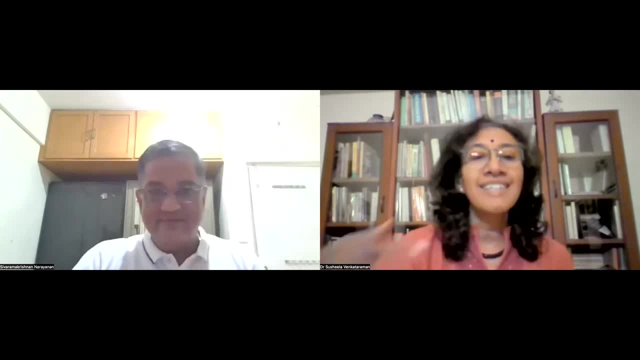 and we've also heard about many of these things in our own webinars here in Bits and Pieces. But what was very nice was painting that picture of how it all falls together to become Industry 4.0. And Professor Amrish mentioned the concept of autonomy. 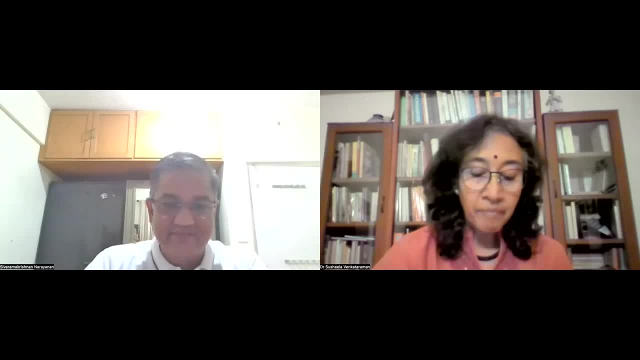 as being at the heart of all of this. The important thing takeaway for me again was that Industry 4.0 is not one monolithic, vague thing, But when we looked at the examples especially, I thought it became very clear that it is. 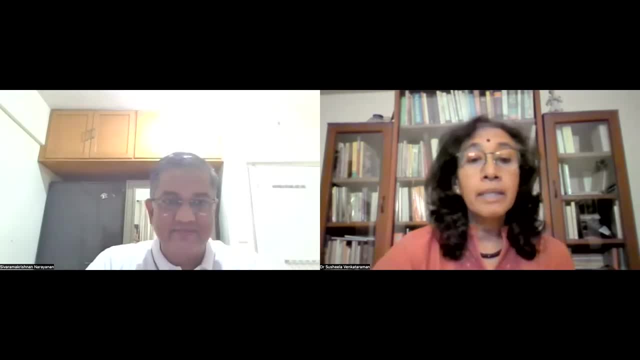 these little, little things that can be taken up, but they do have a large impact, and none of them would be possible if it were not for these pieces of technology that today can work together. It's not about each of them individually, but the fact that they can come together. 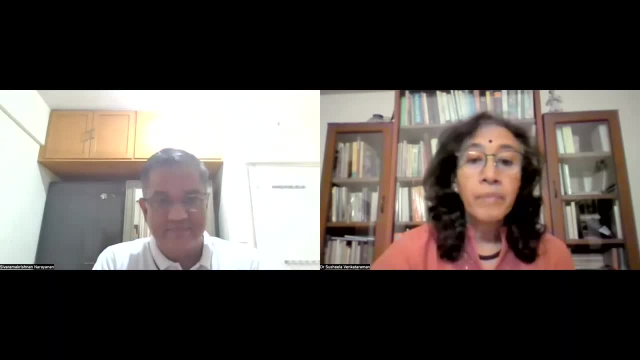 and deliver something in an integrated manner. Then we saw what India's journey in manufacturing has been. We looked at many challenges. We looked at opportunities and advantages. Krish mentioned that these challenges are real and some are imaginary, but we nevertheless need to surmount them. 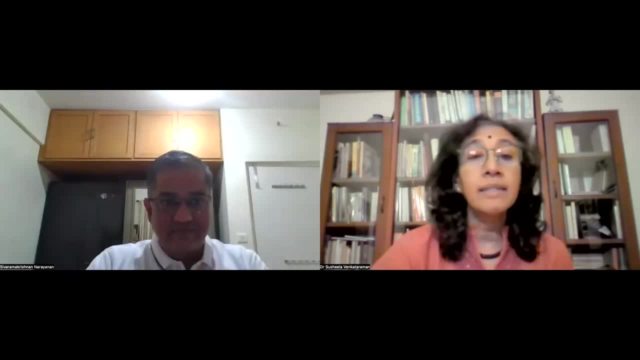 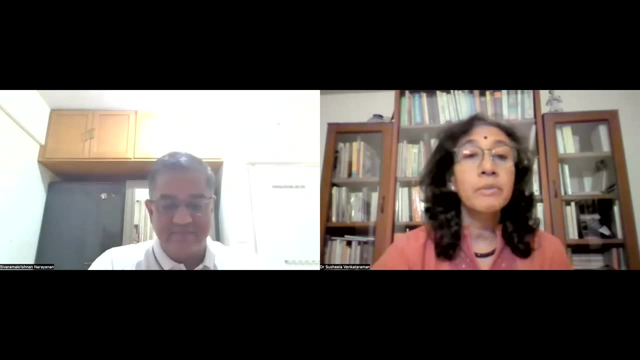 And that, of course, gave us a list of areas that India needs to focus on. The good thing is that we, as a nation, have aspirations to become global leaders, self-sufficient, sustainable, etc. So that's, of course, the first step. 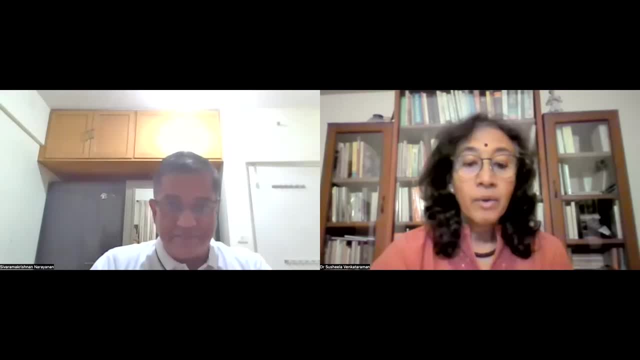 is having that aspiration. I wanted to thank you, Krish, for calling out one challenge, which is the low labor participation of women, And yeah, we do need to do something about it. You know from the time that I remember presenting 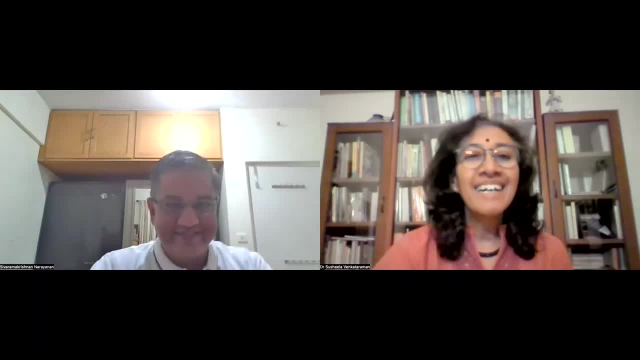 at a CSI conference some 20 years back, I would say exactly the same thing, So thank you for bringing that up. Another one was the industry-academia collaboration, And for our audience I just want to say that's exactly why IIT ACB exists. 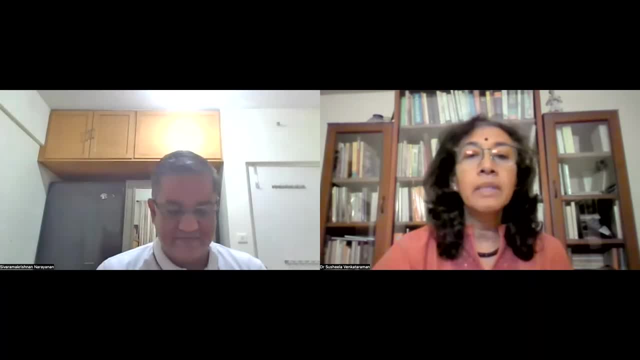 That's exactly what we want to do: to enable the IITs and other institutes and industry to work together, to collaborate to do something that is substantially larger than what anyone could do on their own. So please do talk to us. I've posted our email here. 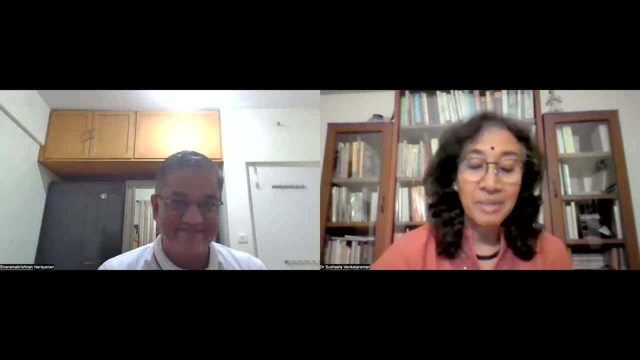 Please do write to us. We are happy to engage and collaborate. Then, finally, we looked at how does a company actually get going on this Industry 4.0 journey, And Krish said: start with single areas. you know things that do have an impact. 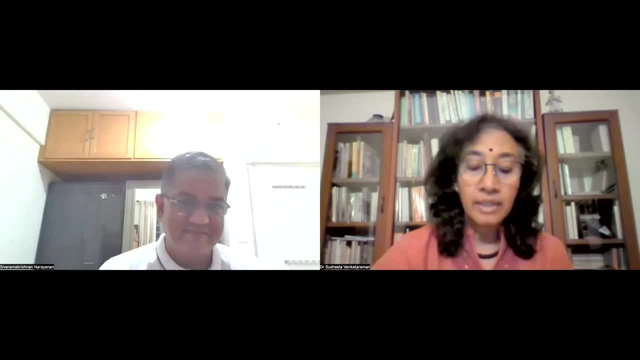 but start with a single area and then the journey kind of just progresses and happens. We saw many examples of what is happening right here in India, and especially, you know, the fact that we have corneal and liver tissue being printed right here in Bangalore. 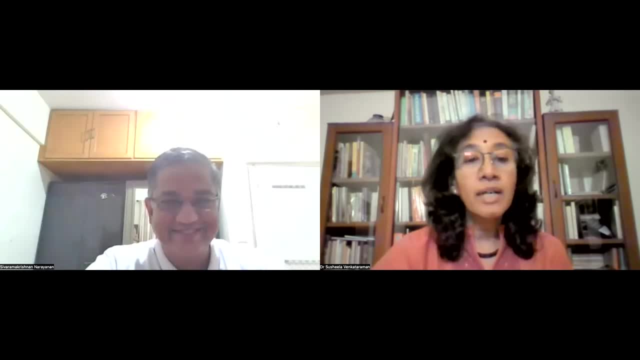 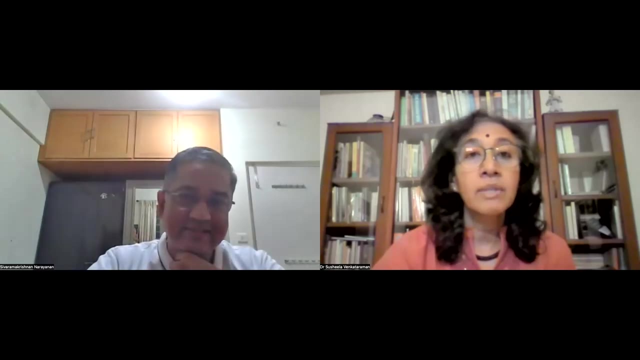 is absolutely fascinating. And then we saw real-life examples of blockchain guided vehicles, computer vision, and how they make a difference, even if that is to a specific area, how that really makes a difference to the company And obviously from there to industry as a whole. 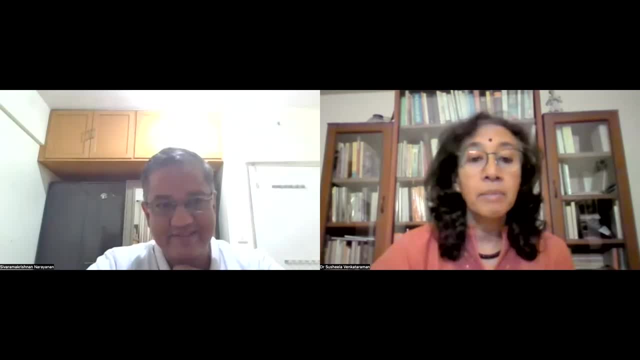 I thought the example of the oxygen lance in blast furnaces was particularly pertinent, because that is an area where we are. you know, human life is at risk, and here's how technology can actually help. We ended the presentation with many questions and concerns. 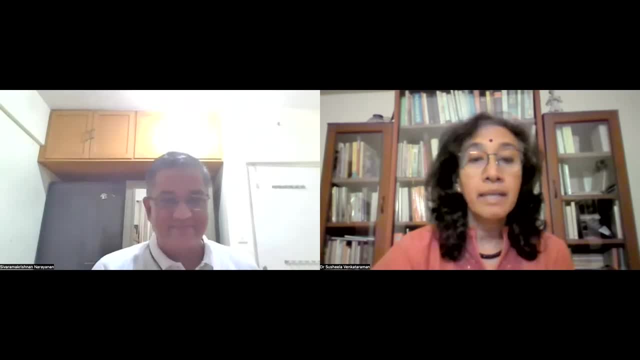 such as cost efficiency, sustainability, relevance to India, the impact on labor, et cetera. We saw many of those issues- New jobs of the future- and they are going to be so different from what we can even think of today. 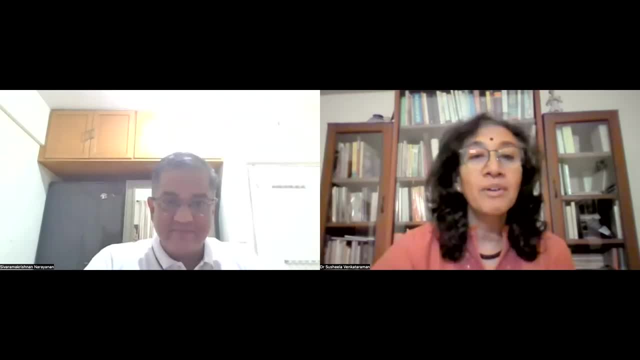 So there's no point kind of thinking about all of that. It is going to be different and we know that. We looked at the impact of all of this on society. The heartwarming story of Mithi Cafe. I thought was very nice.